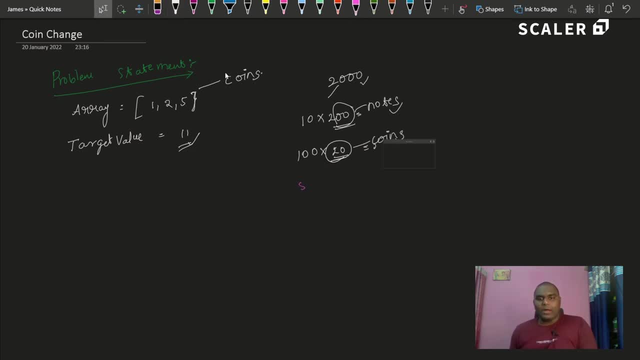 if a shopkeeper has given you a 500 rupees coins and it will be taking four. So here four points will be: scale here is no 200 and, I'm sorry, 250 rupees 500 coins, So thatして 150 rupees 500 of coins, but i'm saying that okay. and if, like, you, have given 2000 rupees, note. 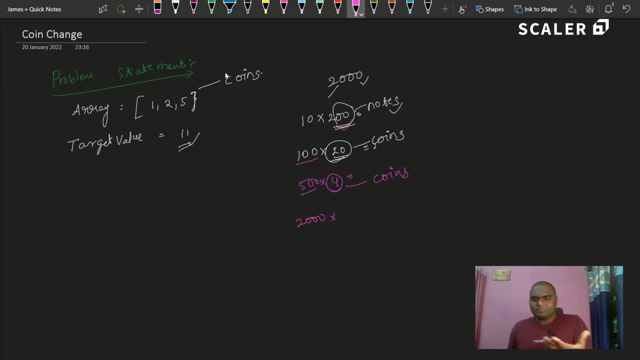 again. he gave you, uh, 2000 rupees. note, okay, then it required only one coin, right, one coin. so this is what? a minimal number of coins, okay, you will get, okay, so this could be your answer. this is your answer. so a minimum coins, okay for an a given a currency, okay, so 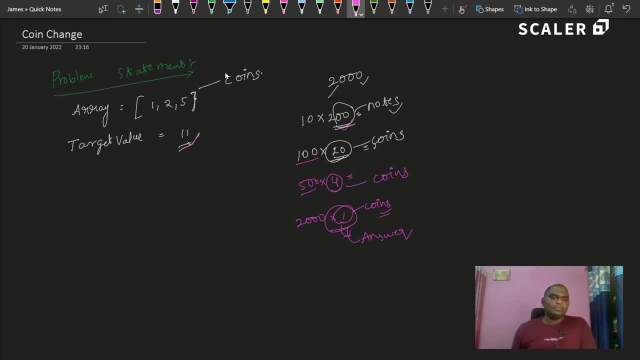 let's try to understand for this particular uh example. okay, so first, okay, so there are one rupee coins, two p coins and five rupee coins. okay, and here one thing to understand here is very, very important. so whenever you are in an interview you have to ask one question at the 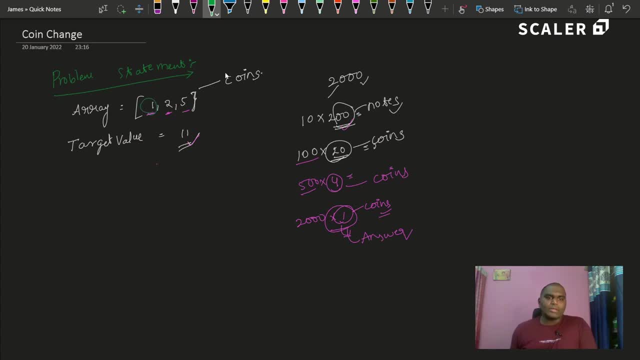 first, what is that question? so, are these coins are infinite supply? means infinite supply like so, uh, can i get this one rupee coins as many times i want? so let's say here to make uh, 11 rupees a change. you required, uh, if you, if you have given 11 one rupee coins. 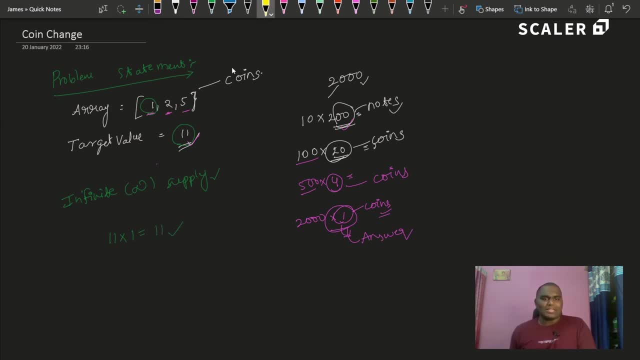 then it will be 11 rupees target, some achieved, okay. so, uh, no, i want, i don't want like that. okay, so what i will do? i will make one into nine rupees, okay, like i will give a nine coins of one rupees, then one two rupees coin. okay, then what happens? it will again 11 targets- i'm achieved. 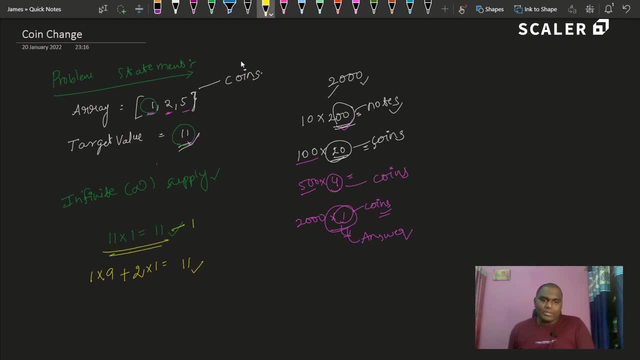 okay. so in this case, totally, we have given 11 coins. i'm now, i am counting 11 coins now here: nine one rupee coins and one two rupee coin, so total 10 coins. so, uh, it's a great right. so i will try. uh, two p coins now, okay. so two into fives are 10. 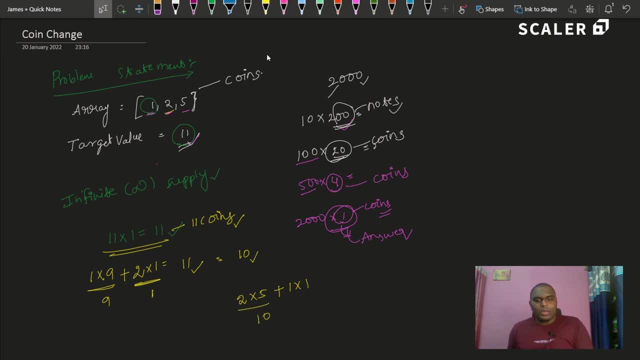 and one one rupee coin. so at uh here and one, it's 11.. so how many coins i have taking now? five plus one, so it's a six coins less than 11 and 10. right, yes, it's acceptable now. is there any other way? let's see, okay, um. 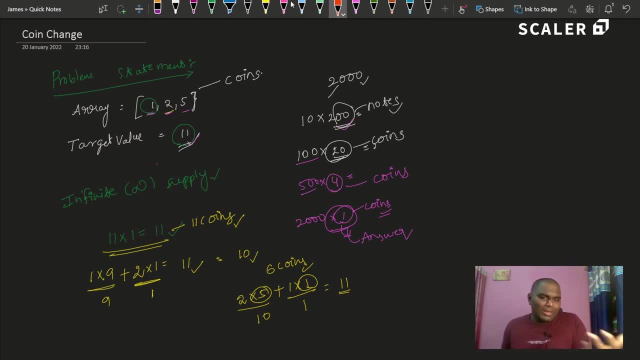 so still, uh, with the one and two combinations we will have, you will be having a more uh coins as well. so like um, three, two rupees coins and five uh, one rupee coin, something like that as well. okay, and uh here, yeah, so now let's come to five rupees. so 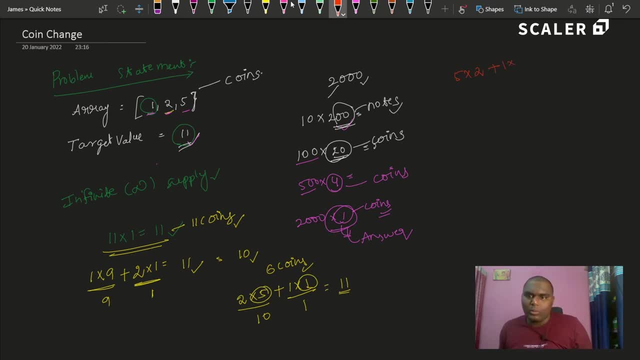 can i say two five rupee coins plus one one rupee coin. totally, i have three coins now, which is um way more better than other solutions, other coins, right, since i am wanted a minimum number of coins required to get target value. okay now, um, so is there any other way that we can reduce this further? let's keep on trying. okay, so one. 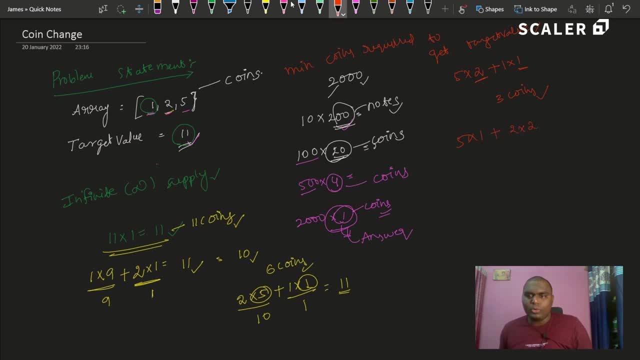 five rupee coin and a two two rupee coin and, uh, so five, four. so one into two, or you can say two into one as well. okay, so it will become four coins. so i can say that three is the minimum coins i required to to make this. 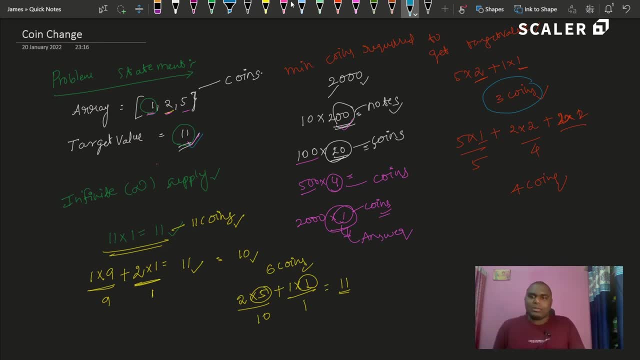 is about 11. so this is what an answer looks like. okay, so this is the answer. if there is an infinite supply of coins, infinite supply of coins, what if? what if, uh, there is only one uh coin is supplying to you at add-on? okay, so, let's see. let's see, uh, the. the given coins are one, two and five. 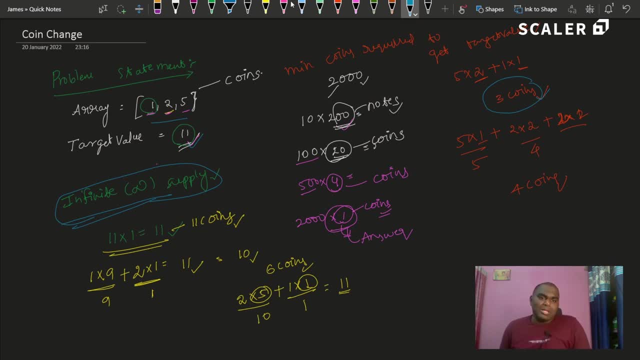 and you're two required to make a 11. it's not required, it's a quite uh greater. so if you add all these as well, you will get only 8 rupees. it's not 11 rupees, right? so you can't make at the change of 11 rupees, so how can you? 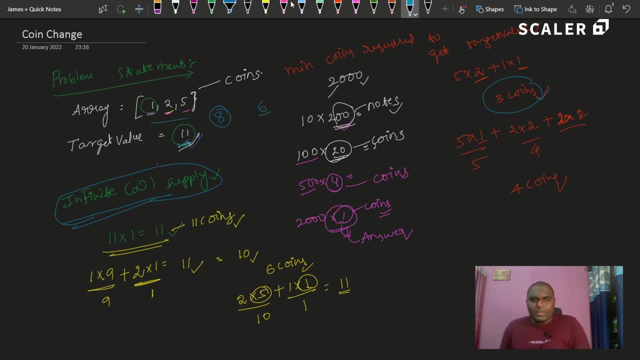 do. let's say, if i have given you a 6 rupees like you need to make change for 6 rupees. now how many minimum coins you require. so if you consider all the 1 coins, then 1 into 6, 6 coins if you required. 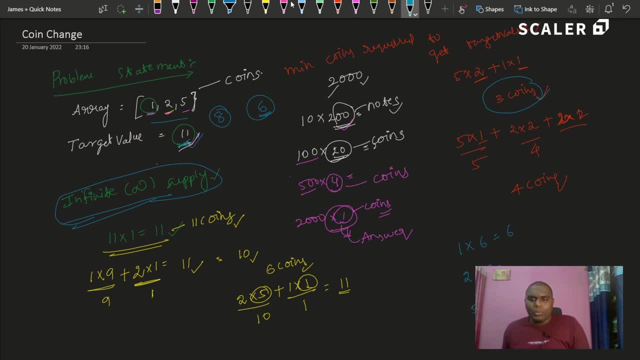 a 3, then 3 coins. 5 into 1 plus 1 into 1 are 2 coins. so this is: can i say this? can i say: at max you require 2 coins. if i am sub, if i am giving a finite and i am searching for, uh, target 6, okay, 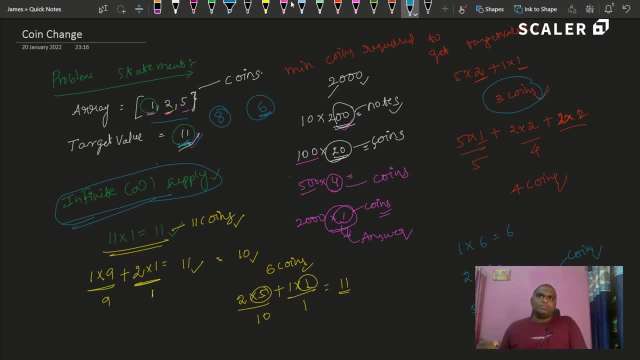 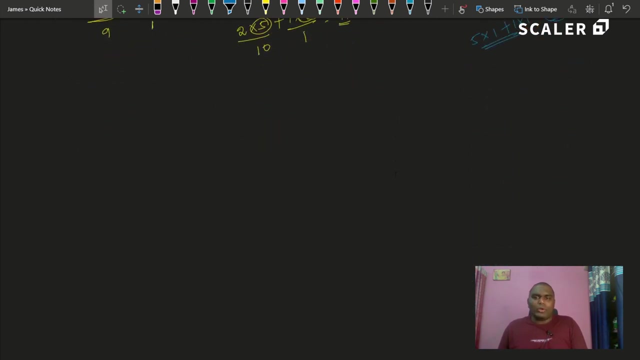 so, but in this, um like tutorial, i will be discussing infinite supply of coins. okay, so i am pretty much sure that after, uh, finishing this entire tutorial, watching this entire tutorial, you will be able to solve this limited number of coins supply on your own. okay, just give it a try. okay, we catch up with another tutorial where i 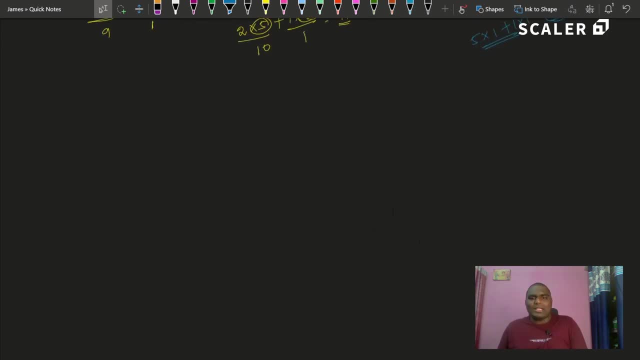 will be explaining with limited number of coins as well. okay, now i hope you have understood the problem statement clearly. so now i recommend you to please pause the video, i think for a while. okay, so i will give you a hint as well. okay, so think in a recursive manner. 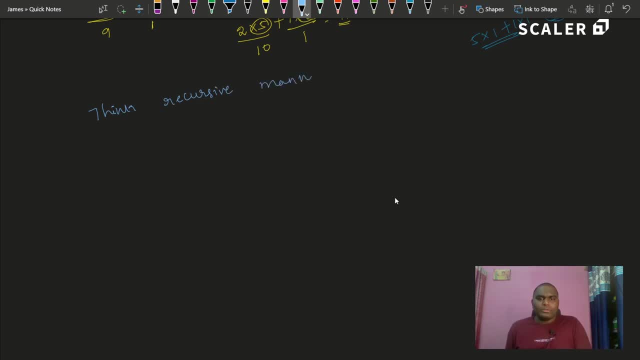 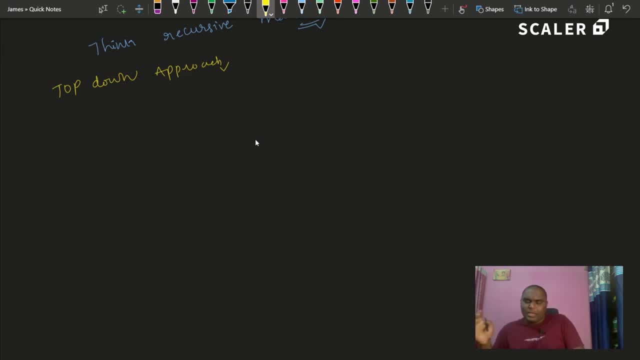 aware. i will be starting from last index and moving towards the starting index. and moving towards the starting index and moving towards the starting index means, means, means, if i have array of size, um, if i have array of size um, if i have array of size, um, like coins of size, uh 10, i will be starting. 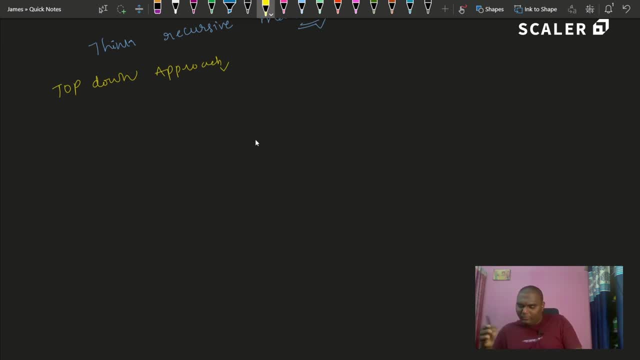 like coins of size uh 10. i will be starting like coins of size uh 10. i will be starting at, at, at 10th element and i will move. i will 10th element and i will move. i will 10th element and i will move. i will keep on moving till the last element. okay. 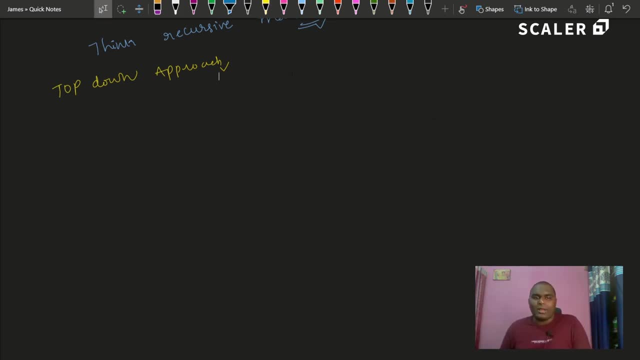 keep on moving till the last element. okay, keep on moving till the last element. okay, first element: sorry, first element. sorry, first element, sorry. okay, that's how top-down approach of. okay, that's how top-down approach of. okay, that's how top-down approach of recursive works. 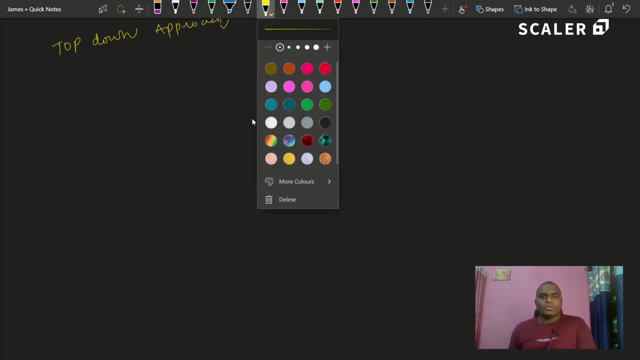 okay, so now let's see. okay, so now, let's see. okay, so now let's see. so, uh, let's stick to the example that we so. uh, let's stick to the example that we so. uh, let's stick to the example that we have now. have now. 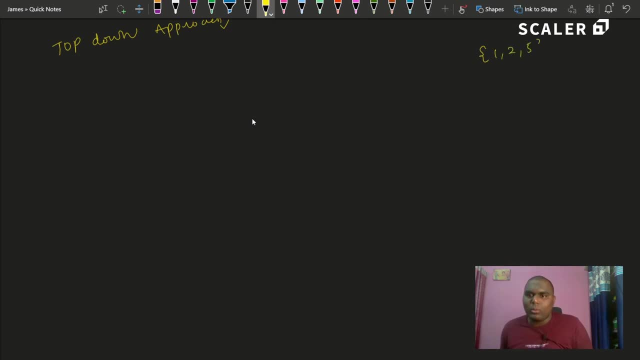 have now. so the array of the coins are 2, so the array of the coins are 2. so the array of the coins are 2, 1, 2, 5 and the target value is 1, 2, 5 and the target value is: 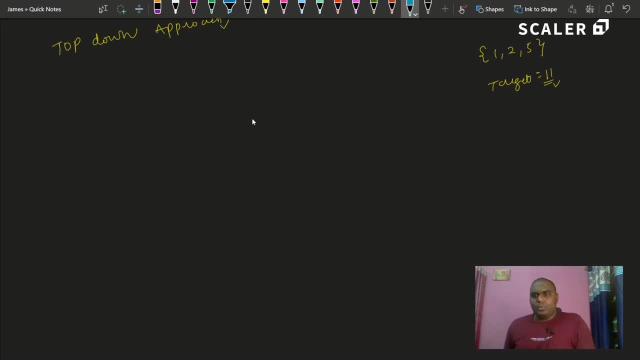 1, 2, 5 and the target value is 11. okay, 11, okay, 11, okay. so let me point out: the index is 0, 1, 2. so let me point out: the index is 0, 1, 2. so let me point out: the index is 0, 1, 2. so what is the last index? the last? 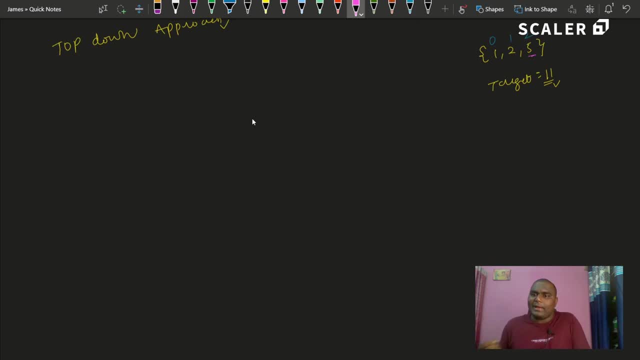 so what is the last index, the last? so what is the last index? the last index is 2, so i will be starting from a index is 2, so i will be starting from a index is 2, so i will be starting from a second index. so here, uh, i'm considering. 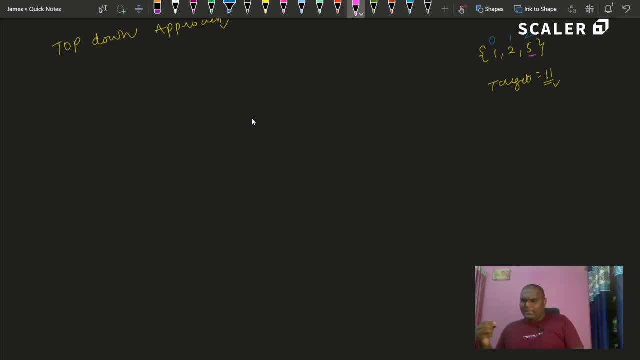 second index. so here, uh, i'm considering second index. so here, uh, i'm considering parameters, or my parameters, or my parameters, or my index and a target value. okay, index and a target value. okay, index and a target value. okay, let's say i will, i will be having a. 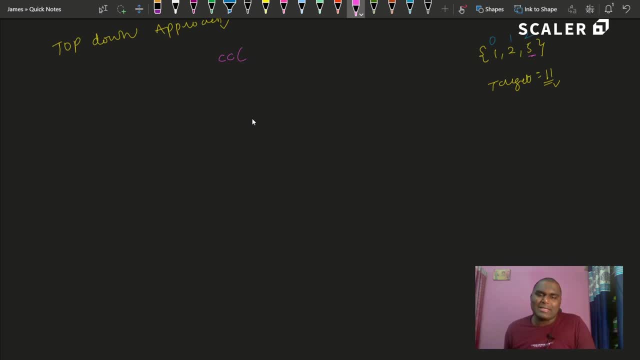 let's say i will, i will be having a. let's say i will, i will be having a function called a coin change. function called a coin change, function called a coin change. let's name this as a cc for our. let's name this as a cc for our. 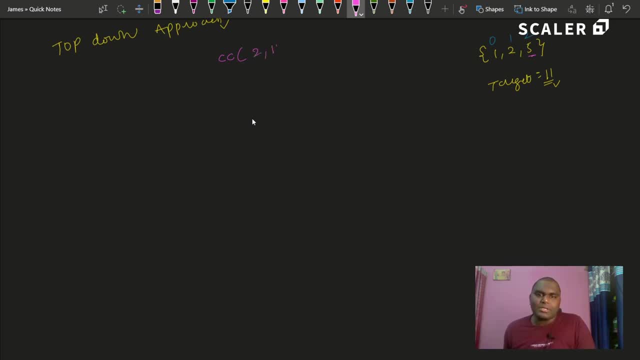 let's name this as a cc for our simplicity, simplicity, simplicity, and i will be starting at 2, and i am, and i will be starting at 2, and i am, and i will be starting at 2, and i am searching for 11, searching for 11. 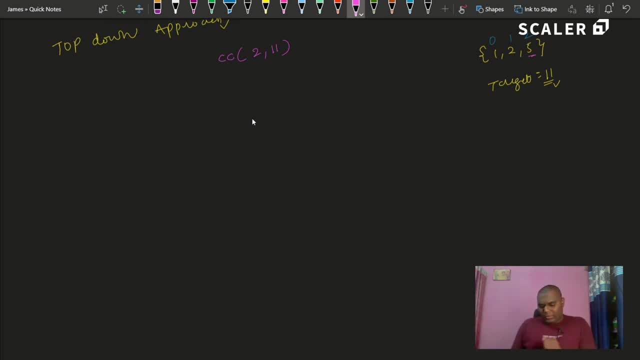 searching for 11. okay, this is what my initial state looks. okay, this is what my initial state looks. okay, this is what my initial state looks like, like, like, now, tell me, tell me. so, now tell me, tell me, so now tell me, tell me. so i'm currently here. what is the decision? 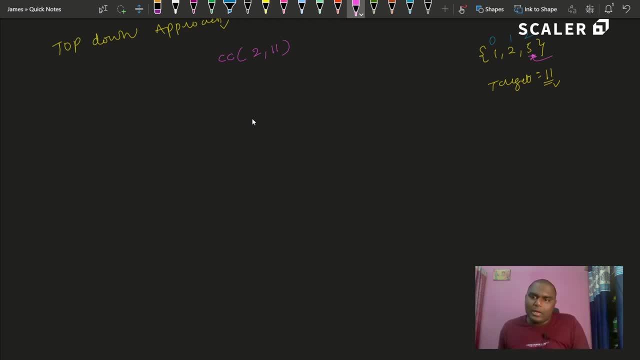 i'm currently here. what is the decision? i'm currently here, what is the decision? can i make here? can i make here, can i make here, so can i say: can i say uh. so can i say. can i say uh. so can i say, can i say uh, if, if? okay, so five is less than 11. 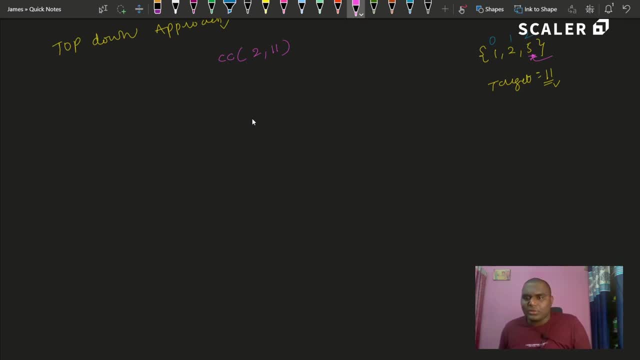 if, if okay, so five is less than 11. if, if okay, so five is less than 11. yes, yes, yes, like happens right, so five is less than. like happens right, so five is less than. like happens right, so five is less than 11. if i make the change of 11, 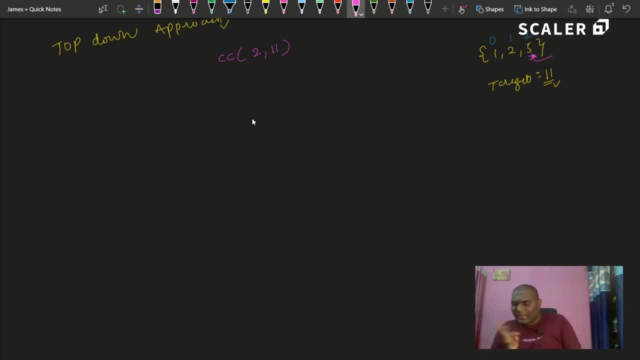 11 if i make the change of 11. 11, if i make the change of 11, i can have five in that thing. so i can have five in that thing, so i can have five in that thing. so secondary is like: uh, forget about rest. 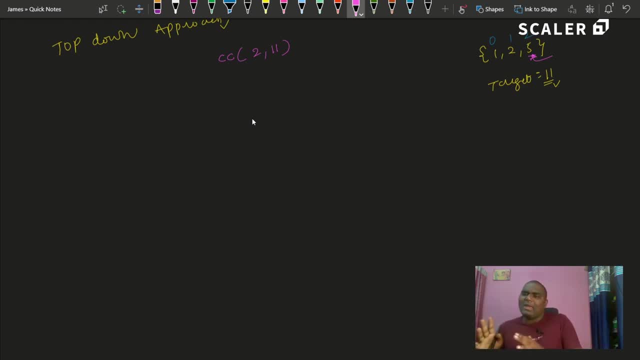 secondary is like uh, forget about rest. secondary is like uh forget about rest of the elements, of the elements, of the elements. just think about this five. so can i make. just think about this five. so can i make. just think about this five. so can i make. can i include a 5 in my 11 coins? 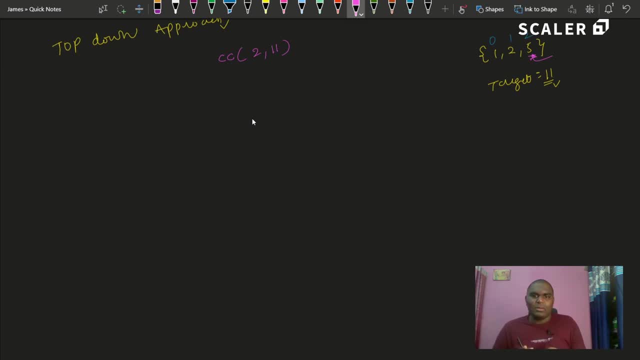 can i include a 5 in my 11 coins? can i include a 5 in my 11 coins? yes, i can write so 5 is less than 11. yes, i can write so 5 is less than 11. yes, i can write so 5 is less than 11, so i must can include that okay. 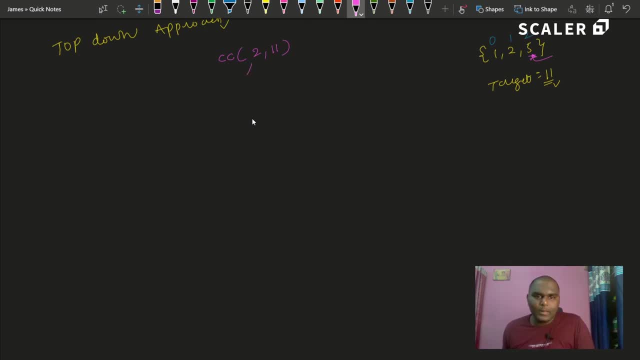 so i must can include that. okay, so i must. can include that. okay, so cc, and so my current sum will be so cc, and so my current sum will be so cc, and so my current sum will be: uh, going to be a six, right, so i'm. 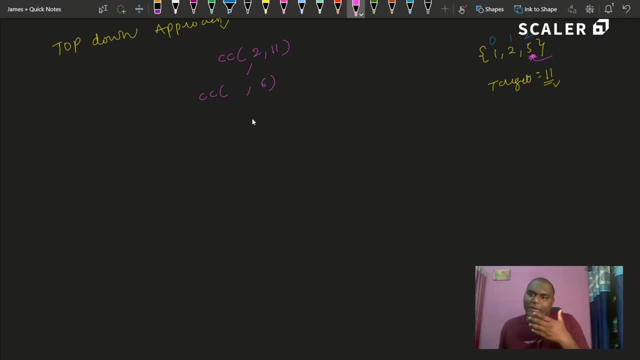 uh, going to be a six right. so i'm uh going to be a six right. so i'm searching for 11 initially. searching for 11 initially. searching for 11 initially, and i have included a five in it. okay, and i have included a five in it, okay. 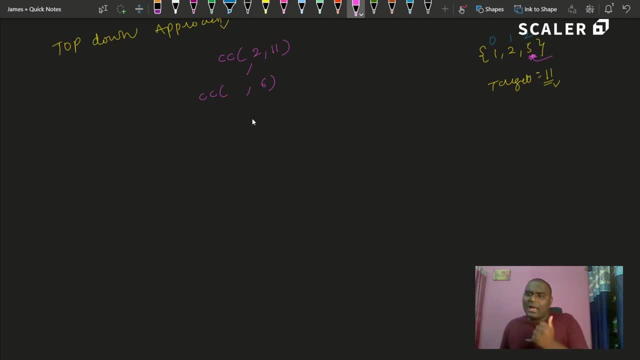 and i have included a five in it. okay, and um and um and um, i have reduced that target sum to the six. i have reduced that target sum to the six. i have reduced that target sum to the six now because i have reduced that 11 minus. 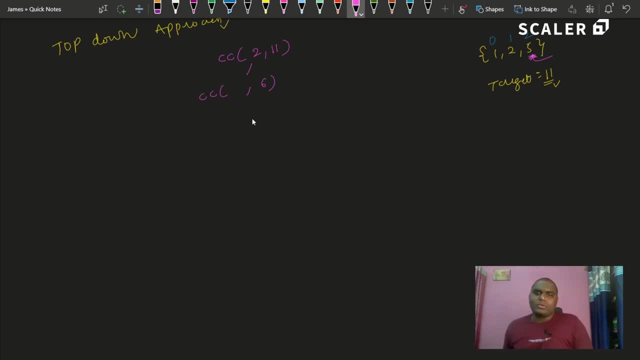 now, because i have reduced that 11 minus now, because i have reduced that 11 minus six. okay, six, okay, six, okay, done now. tell me, done now, tell me, done now, tell me. so so i can take that if i don't wish to take. i can take that if i don't wish to take. 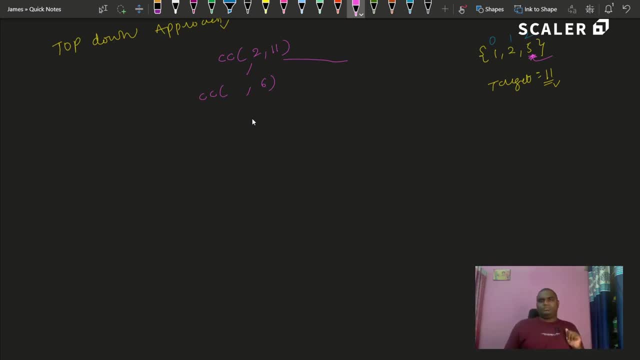 i can take that if i don't wish to take that, that that. so i'm not interested in taking that a. so i'm not interested in taking that a. so i'm not interested in taking that a file, file, file. that's right. so that's my choice, okay, so 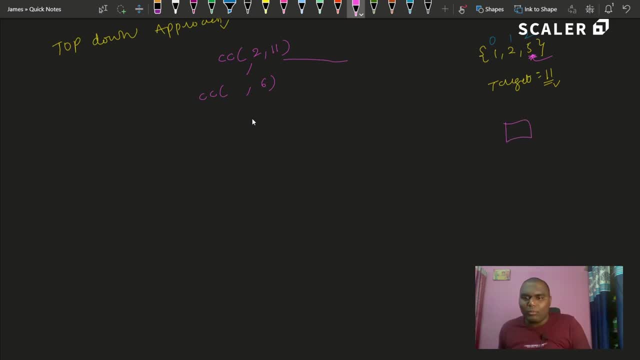 that's right, so that's my choice. okay, so that's right, so that's my choice. okay. so let's, let's assume you are shopkeeper. let's, let's assume you are shopkeeper. let's, let's assume you are shopkeeper and you have all the one coins here. two. 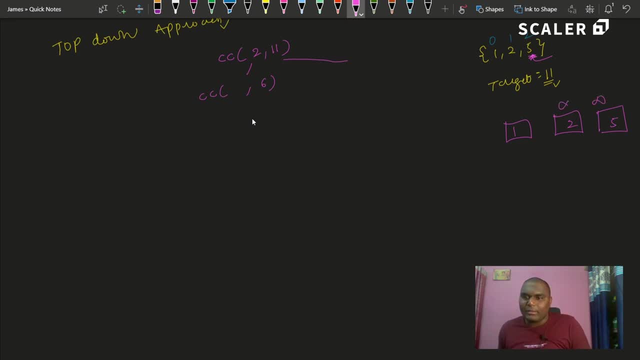 and you have all the one coins here. two, and you have all the one coins here, two coins here and five coins here, like coins here and five coins here, like coins here and five coins here, like infinite, infinite, infinite, infinite. and you, we have to give the change of. 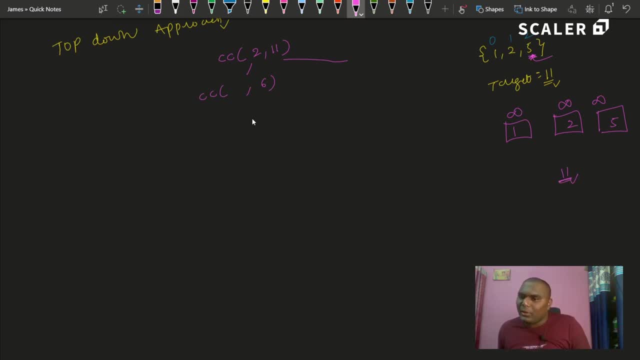 and you we have to give the change of, and you we have to give the change of eleven rupees, eleven rupees, eleven rupees. so it's your take. whether you can give, so it's your take. whether you can give, so it's your take whether you can give. take this uh five. so i wanted to give. 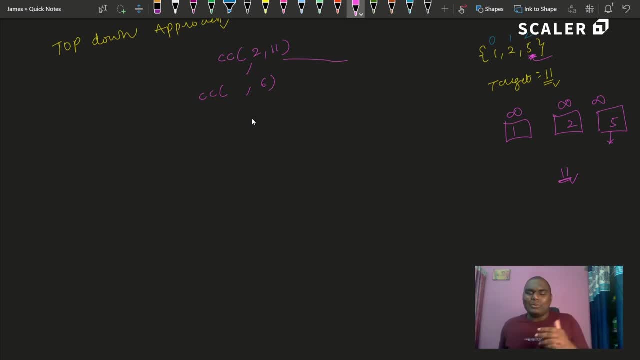 take this uh five. so i wanted to give. take this uh five. so i wanted to give only one rupee coins to the guy, only one rupee coins to the guy, only one rupee coins to the guy so i can uh. so that's a decision of. 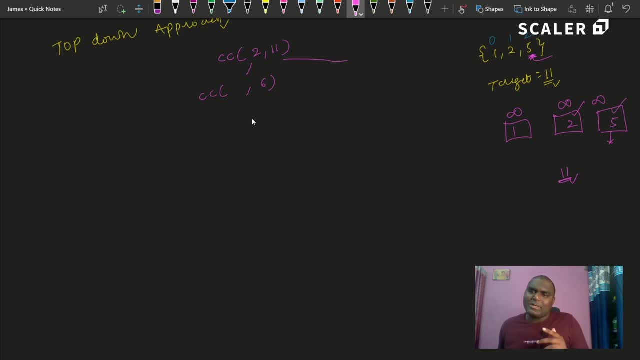 so i can uh, so that's a decision of. so i can uh, so that's a decision of shopkeeper: shopkeeper: shopkeeper: okay, so he can give two rupees he can. okay, so he can give two rupees he can. okay, so he can give two rupees. he can give five rupees he can give. 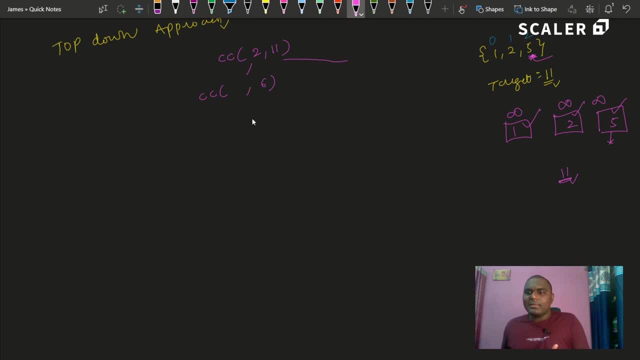 five rupees. he can give uh one rupee as well, but at the end of uh one rupee as well, but at the end of uh one rupee as well, but at the end of the day, it is the day. it is the day. it is his choice. okay, so that is what we have. 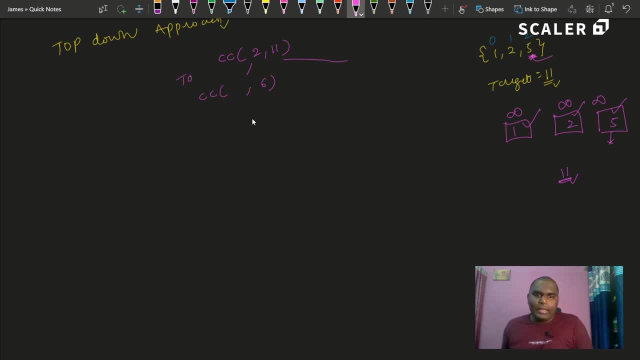 his choice: okay, so that is what we have. his choice, okay, so that is what we have to stick to stick to stick. okay, so here this is called a take. okay, so here this is called a take. okay, so here this is called a take. this is called. 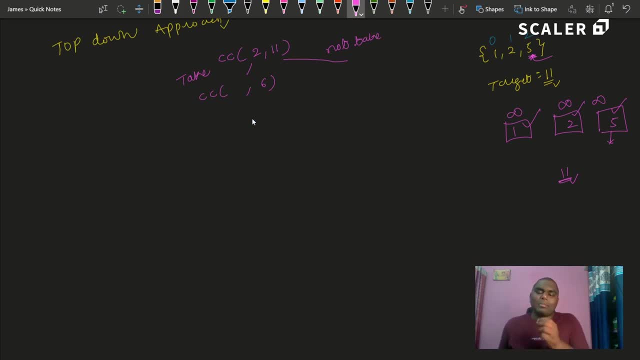 this is called. this is called not take okay, so take means you are not take okay, so take means you are not take okay, so take means you are considering that particular value, considering that particular value, considering that particular value into your uh change and not take means, into your uh change and not take means. 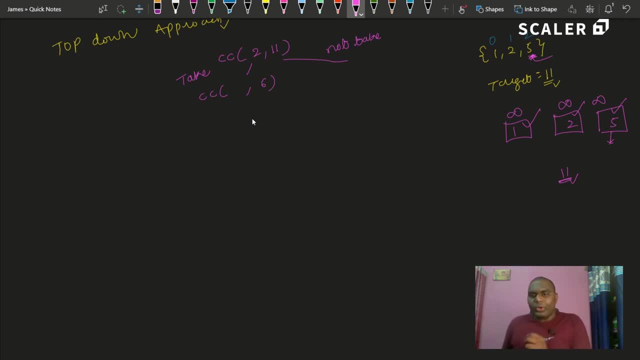 into your uh. change and not take means you are not including your uh that particular value into your sum. uh, that particular value into your sum. uh, that particular value into your sum. okay, okay, okay, now, now. so if you have included this, now, now. so if you have included this, 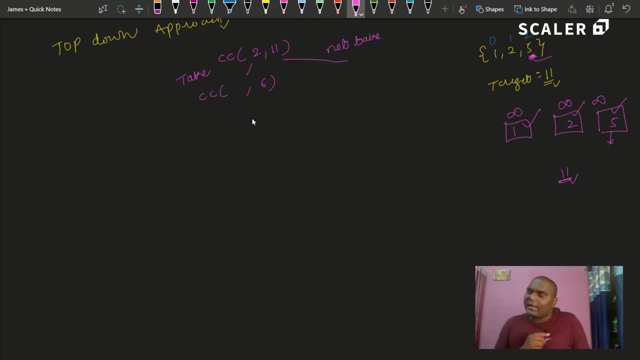 now, now. so if you have included this- okay, you have, you could. okay, you have you could. okay, you have, you could- included this particular five into your, included this particular five into your, included this particular five into your target sum, target sum, target sum. now tell me so, since it's an infinite. 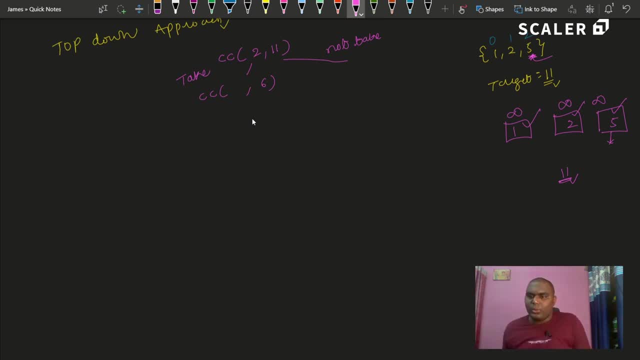 now tell me so, since it's an infinite. now tell me so, since it's an infinite setup in setup in setup in, you have infinite uh coins, okay. so here you have infinite uh coins. okay. so here you have infinite uh coins. okay. so here you will be having all the coins, okay. 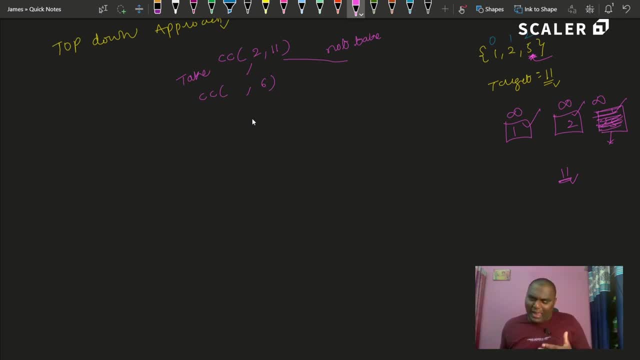 you will be having all the coins. okay, you will be having all the coins. okay, all like thousand infinite coins. so all like thousand infinite coins. so if i am making it a choice of like, if i, if i am making it a choice of like, if i, if i am making it a choice of like, if i am, 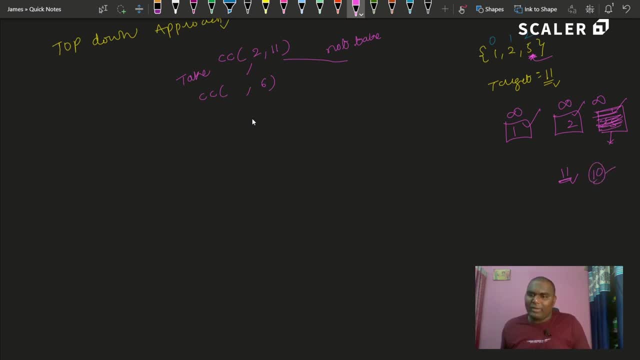 am am. i wanted the change of 10. i can give all i wanted the change of 10. i can give all. i wanted the change of 10. i can give all the five rice, the five rice, the five rice, all the five, two fives. that is possible. 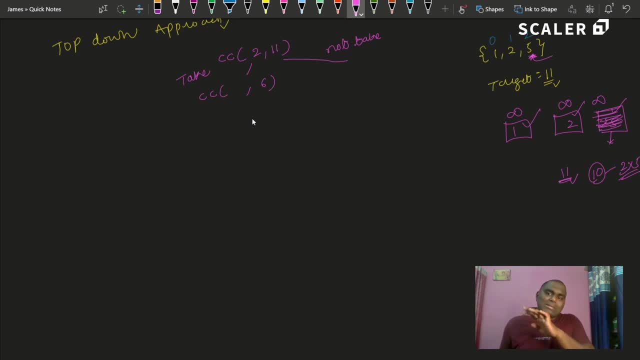 all the five, two fives that is possible. all the five, two fives, that is possible, right? so in that case though, if you have right, so in that case though, if you have right, so in that case though, if you have considered that particular value, considered that particular value, 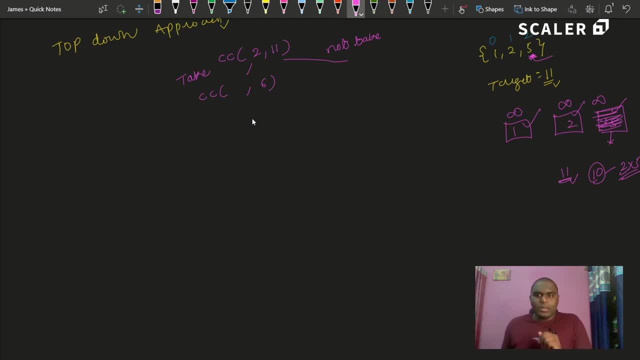 considered that particular value. you can again consider that value. so you can again consider that value. so you can again consider that value. so here do i need to move to my next index? here do i need to move to my next index. here do i need to move to my next index? no, i can stay there only, and again i can. 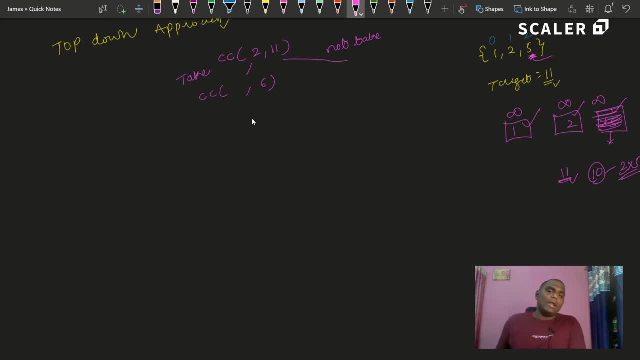 no, i can stay there only, and again i can. no, i can stay there only, and again, i can check whether that particular value is, check whether that particular value is, check whether that particular value is again included after after including one, again included after after including one again included after after including one time. 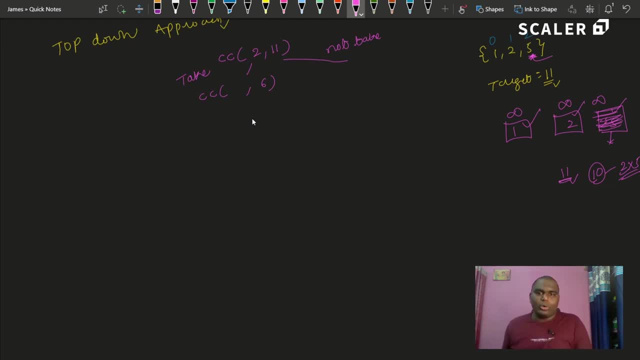 time, time and again i will check whether that can, and again i will check whether that can, and again i will check whether that can be included or not be included, or not be included or not. okay, so i will stay in that second index. okay, so i will stay in that second index. 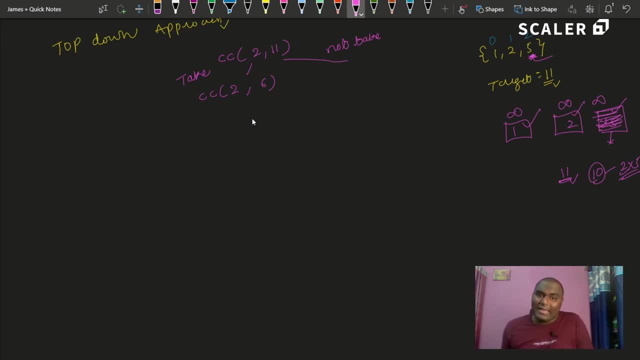 okay, so i will stay in that second index only, only only now. this is the case of if i take, if i now. this is the case of if i take, if i now. this is the case of if i take, if i not take, if i not take, i don't wish to. 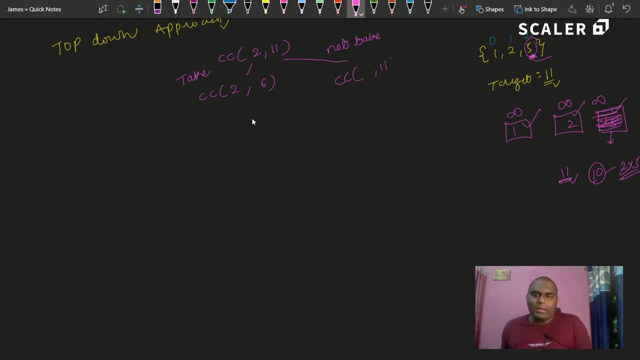 not take. if i not take, i don't wish to not take. if i not take, i don't wish to take this five, take this five, take this five. okay, then my target will be 11, and i'm so. okay, then my target will be 11 and i'm so. 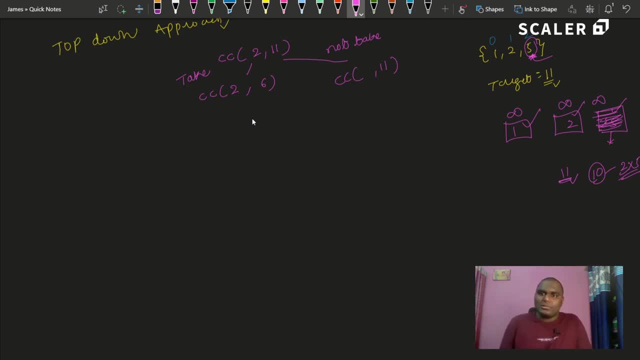 okay, then my target will be 11, and i'm so. if i'm not interested to take this file, if i'm not interested to take this file, if i'm not interested to take this file, i can move to. i can move to, i can move to us next index, right, so i will make my 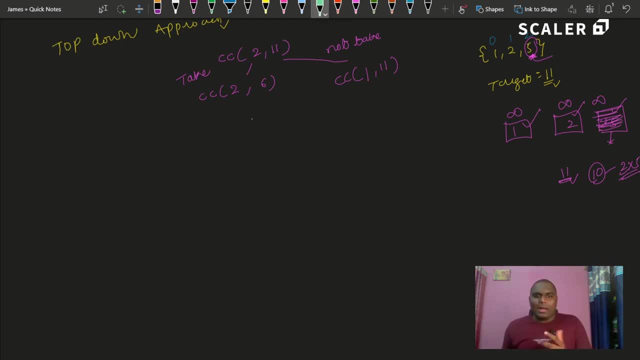 us next index. right, so i will make my us next index. right, so i will make my index as one index, as one index, as one. oh, i hope you guys have understood okay. oh, i hope you guys have understood, okay. oh, i hope you guys have understood. okay, let me tell you so here what i am doing. 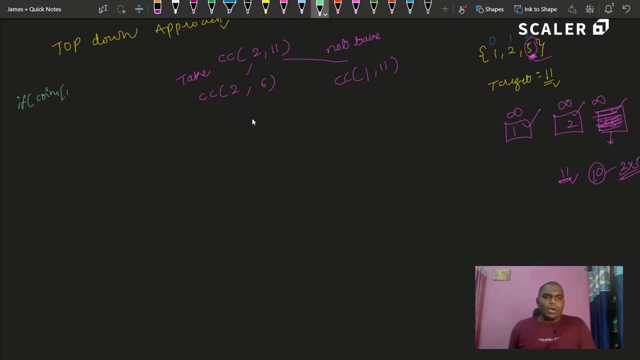 let me tell you so here what i am doing. let me tell you so here what i am doing. so, if so, if so, if let's say coins of index, let's say coins of index, let's say coins of index, uh, less than, uh, less than, uh, less than target, okay, so, less than target. so if 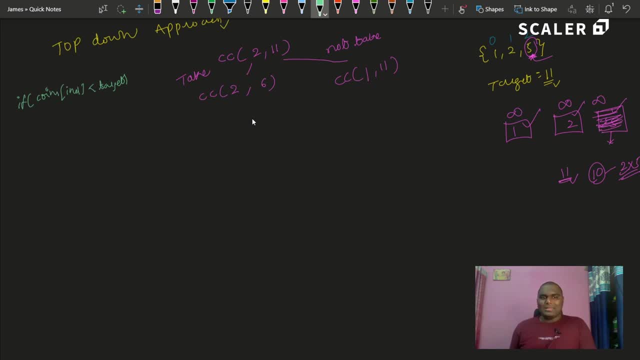 target- okay, so less than target. so, if target- okay, so less than target. so, if this is the case, what i'm doing. this is the case, what i'm doing. this is the case, what i'm doing- okay. if this is the case, what i'm doing- okay. if this is the case, what i'm doing. 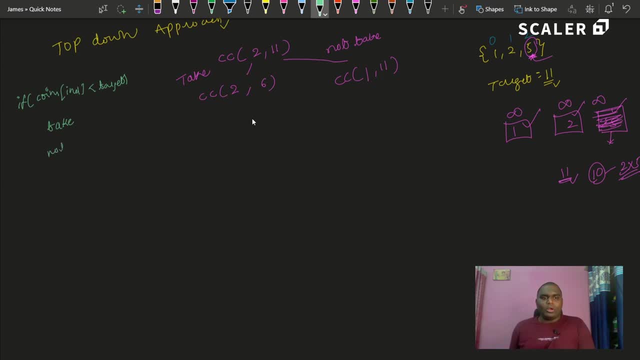 okay, if this is the case, what i'm doing? so either i can take, so either i can take, so either i can take or not take, or not take or not take. okay, if i'm taking this, i'm doing this. okay, if i'm taking this, i'm doing this like i'm my subtracting that particular. 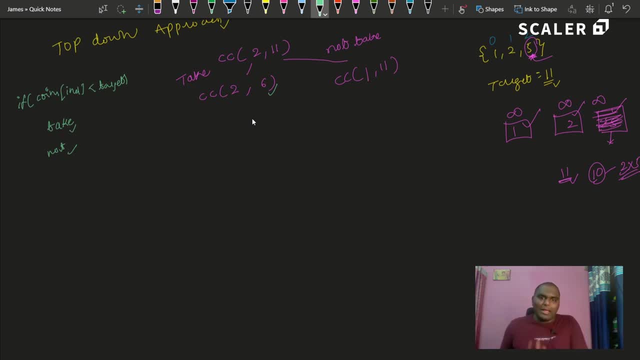 like i'm my subtracting that particular, like i'm my subtracting that particular coin from my target sum and i am again coin from my target sum and i am again coin from my target sum and i am again staying back there only because i have staying back there, only because i have. 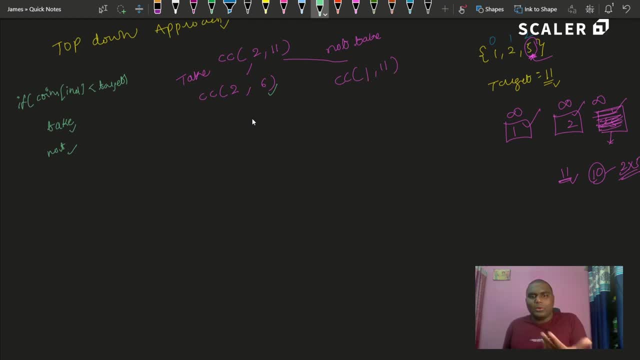 staying back there only because i have to to to make the uh i have to include as i don't make the uh i have to include as i don't make the uh i have to include as i don't know whether again that value can be, know whether again that value can be. 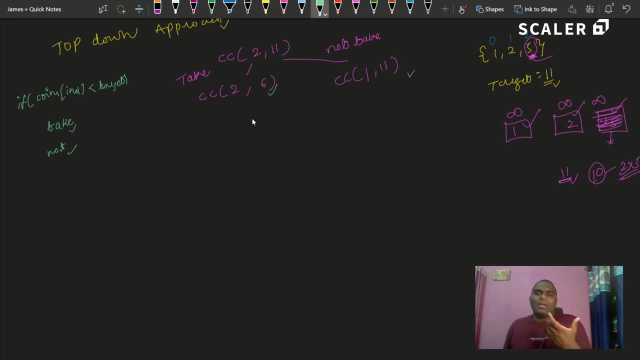 know whether again that value can be included or not included, or not included or not. okay and okay and okay. and if i, if i don't wish to take that kind, if i, if i don't wish to take that kind, if i, if i don't wish to take that kind, i can simply just move on, okay, so, uh, my 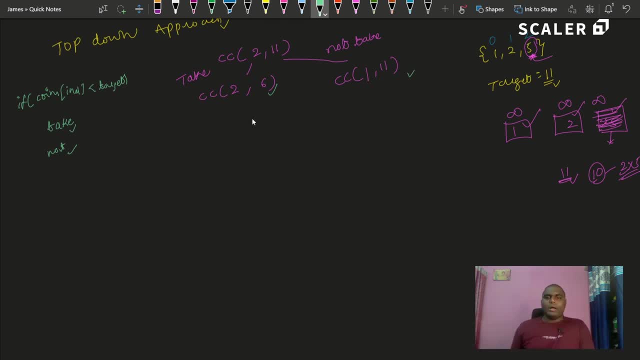 i can simply just move on, okay. so, uh, my, i can simply just move on okay. so, uh, my target sum will be target somewhere okay. target sum will be target somewhere okay. target sum will be target somewhere okay. so, here if i, if i, so, here if i, if i. 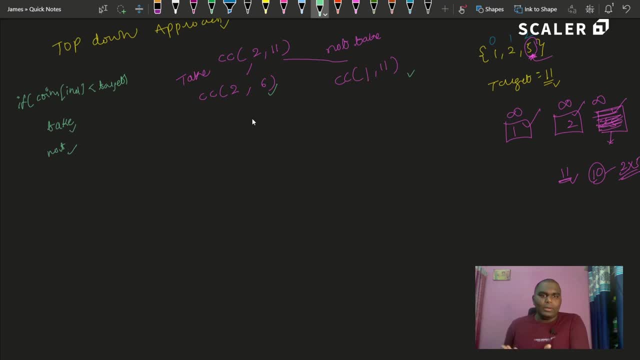 so here, if i, if i consider that, if you, if you take that, consider that, if you, if you take that, consider that, if you, if you take that particular uh coin, what you need to do particular uh coin, what you need to do particular uh coin, what you need to do, you need to increase your coins, right? so? 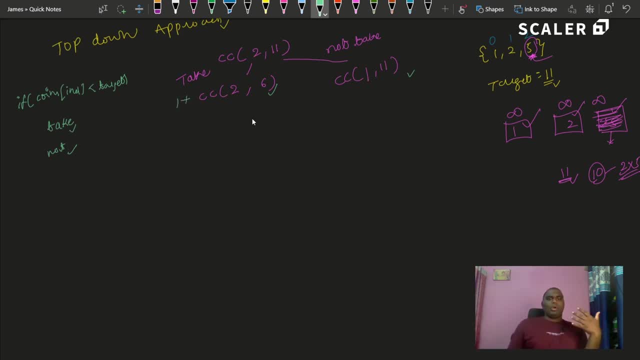 you need to increase your coins, right? so you need to increase your coins, right. so i will simply return one plus. i will simply return one plus. i will simply return one plus. okay, if you are, if you wish to take. okay, if you are, if you wish to take. 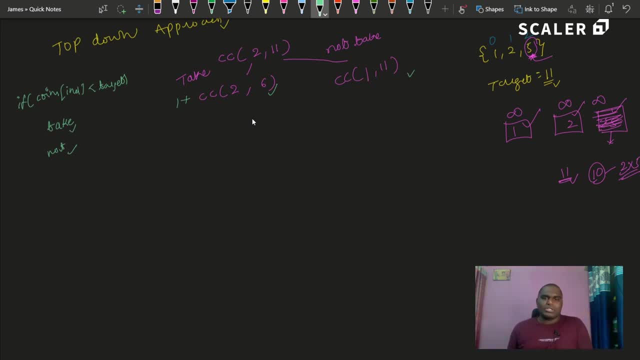 okay, if you are, if you wish to take that coin, you have to increase one value that coin. you have to increase one value that coin, you have to increase one value. so, how much okay now. so, how much okay now. so how much okay now, let's go. so again, you are standing that. 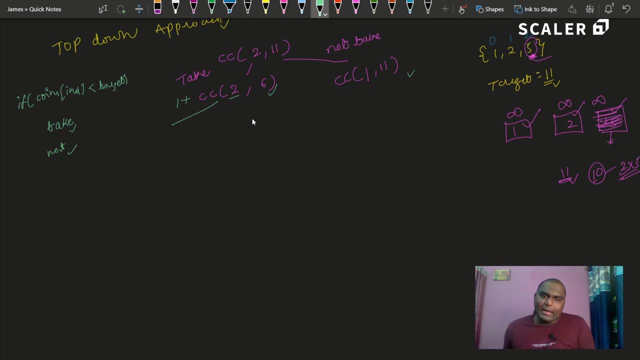 let's go so again you are standing that. let's go so again you are standing that particular thing, particular thing, particular thing, so uh, now second index, and you have a. so uh, now second index, and you have a. so uh, now second index, and you have a target of. 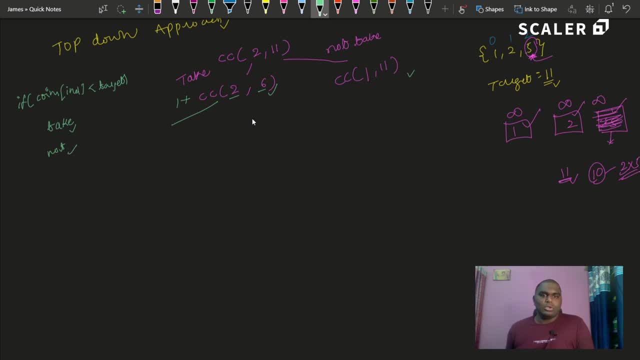 target of target of six, so five is less than six. yes, six so five is less than six. yes, six so five is less than six. yes, so again, what you can do, you can take. so again, what you can do, you can take. so again what you can do, you can take that value. 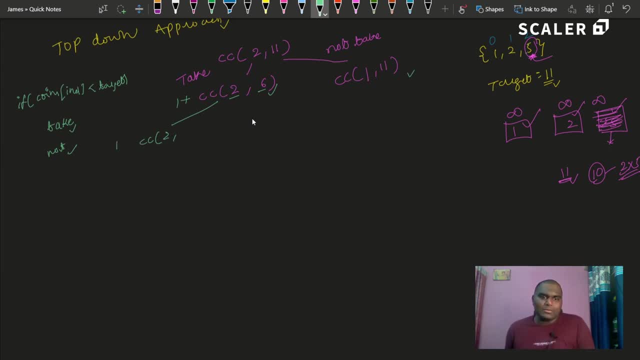 that value, that value. so two, and i am, if i take that, i am so, i am if i take that, i am, so i am if i take that i am standing there itself, standing there itself, standing there itself, and i am making the sum as one now, and 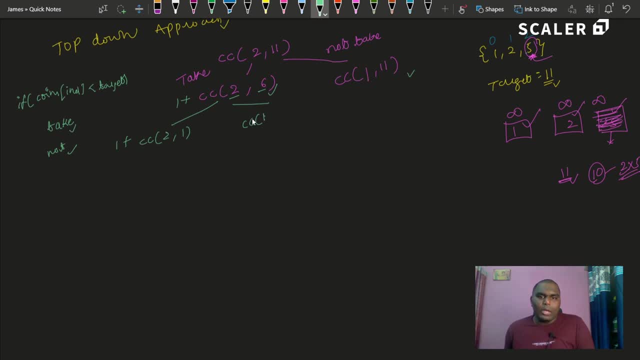 and i am making the sum as one now, and, and i am making the sum as one now. and if i don't wish to take that, if i don't wish to take that, if i don't wish to take that, so it will be one, so it will be one. 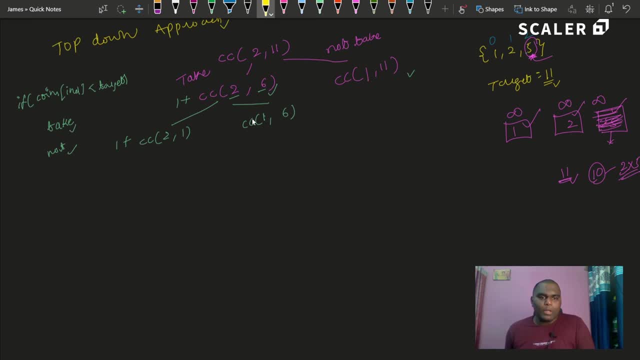 so it will be one and six now and six now and six now, now again. so i am standing at second now again. so i am standing at second now again. so i am standing at second index, index index and i have, i am aiming for target one now. 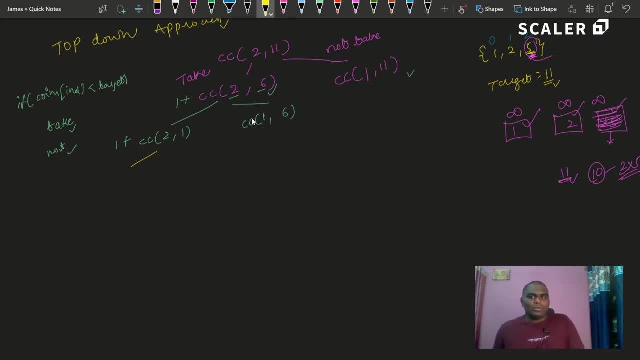 and i have. i am aiming for target one now and i have i am aiming for target one now. so five greater than one right. so five greater than one right. so five greater than one right. so i am, i want the change for one rupee. so i am, i want the change for one rupee. 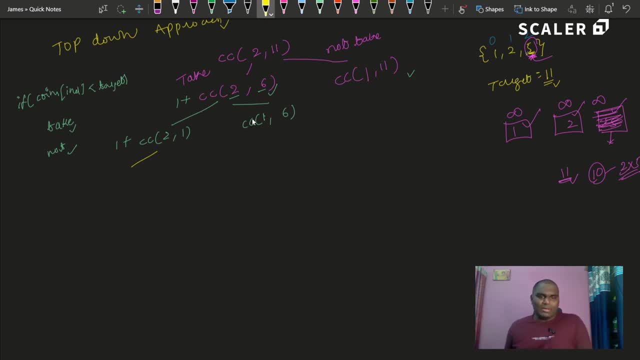 so i am. i want the change for one rupee and you are showing me five rupees that and you are showing me five rupees that and you are showing me five rupees that is not sufficient, like it's exceeded, is not sufficient, like it's exceeded. 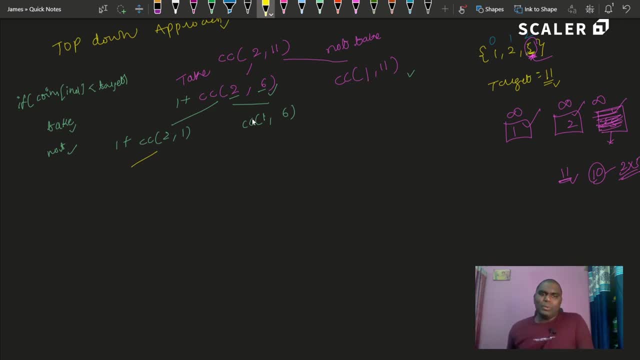 is not sufficient, like it's exceeded right, so you must not include that right. so you must not include that right, so you must not include that. so what you will do so, what you will do, so, what you will do, so, can i say, so, can i say. 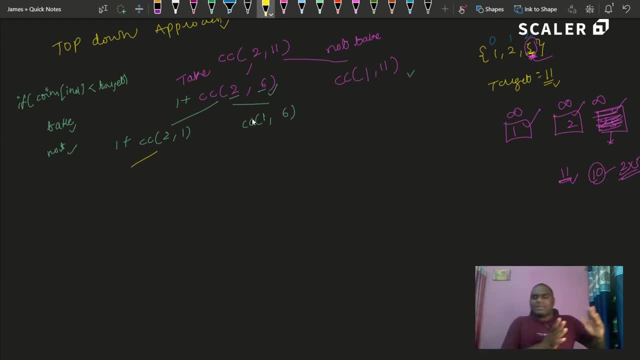 so can i say so if five is not included? so, if five is not included, so if five is not included, uh, there are some other coins which, uh, there are some other coins which, uh, there are some other coins which might include. right, so what i can do? i? 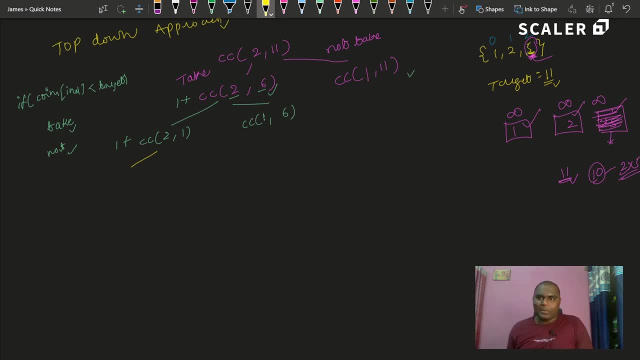 might include right so what i can do. i might include right so what i can do. i can simply i won't take that i won't take. can simply i won't take that i won't take. can simply i won't take that, i won't take that. 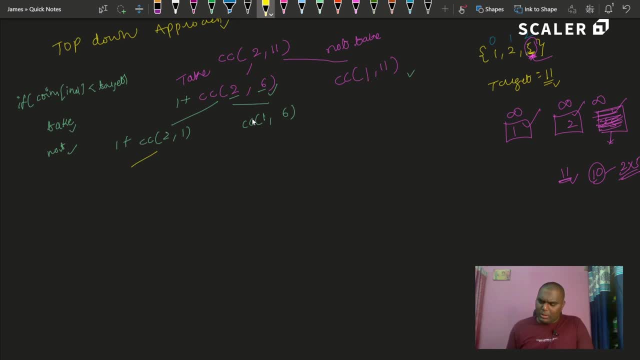 that that, okay, i won't take that, i can just move. okay, i won't take that, i can just move. okay, i won't take that, i can just move to another indexes. okay, which is a cc to another indexes. okay, which is a cc to another indexes. okay, which is a cc of. 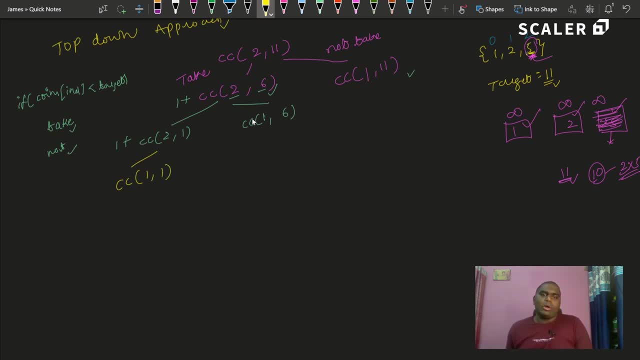 of of one, so at two snakes, one and again target one. so at two snakes, one and again target one. so at two snakes, one and again. target of one of one of one. yes, here i have only one choice, okay. yes, here i have only one choice, okay. 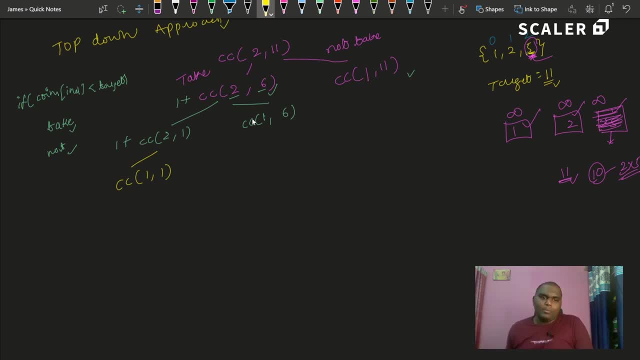 yes, here i have only one choice. okay, i wish not to take that, that's it. okay, now i'm standing at one index and i'm now i'm standing at one index and i'm now i'm standing at one index and i'm searching for. searching for. 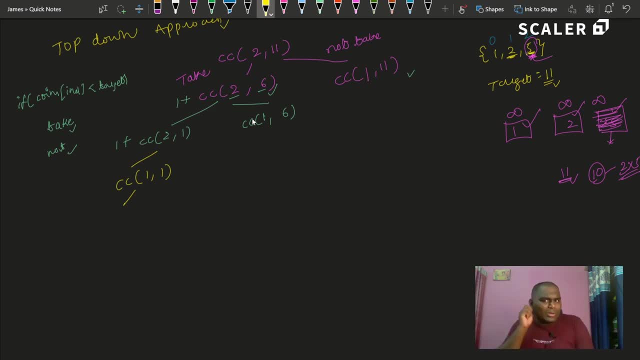 searching for one value. yes, uh, two greater than one value. yes, uh, two greater than one value. yes, uh, two greater than one. so i may not include that i have only one. so i may not include that i have only one. so i may not include that i have only one choice here. 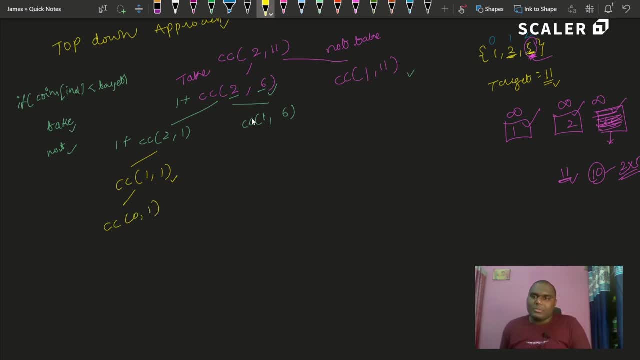 one choice here. one choice here: now again: what i get to zero comma one. so now again what i get to zero comma one. so now again what i get to zero comma one. so i'm standing at one rupee coin and i'm i'm standing at one rupee coin and i'm. 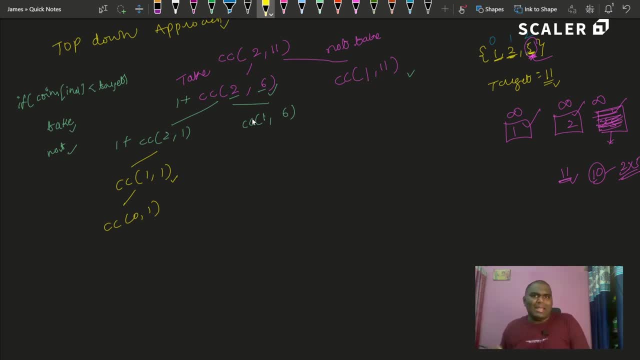 i'm standing at one rupee coin and i'm searching for one rupee target. so is searching for one rupee target. so is searching for one rupee target. so is that defined? that defined? that defined? yes, i can include. so which is a less? yes, i can include so which is a less. 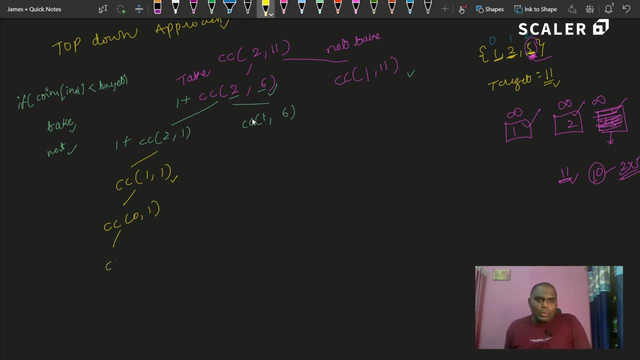 yes, i can include so, which is a less than or equal to so than, or equal to so than or equal to so i can include so one plus. so i can include so one plus. so i can include so one plus. so i have taken that. okay, i have taken that. 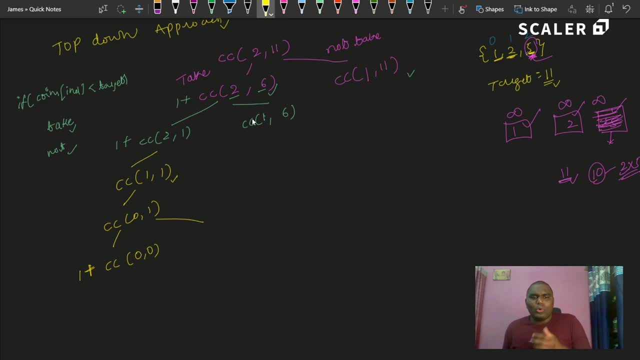 i have taken that. okay, i have taken that. i have taken that. okay, i have taken that. zero comma, zero, zero, comma, zero, zero, comma, zero, right. and i, if i don't wish to take that right, and i, if i don't wish to take that right, and i, if i don't wish to take that, cc of. 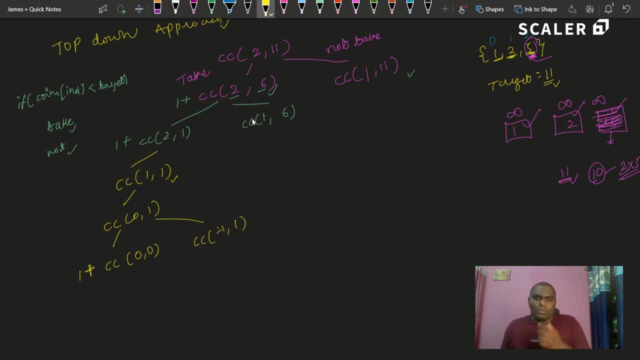 cc of cc of minus one and minus one and minus one, and my sum will be minus one. only my sum will be minus one, only my sum will be minus one, only okay, so, okay, so, okay. so now tell me my target sum became. now tell me my target sum became. 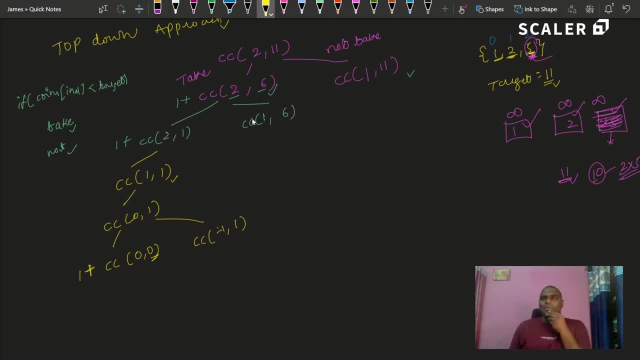 now tell me: my target sum became: uh, my target uh coin will become a zero. uh, my target uh coin will become a zero. uh, my target uh coin will become a zero. so, so, so i got. it means that i got the change for. i got it means that i got the change for. 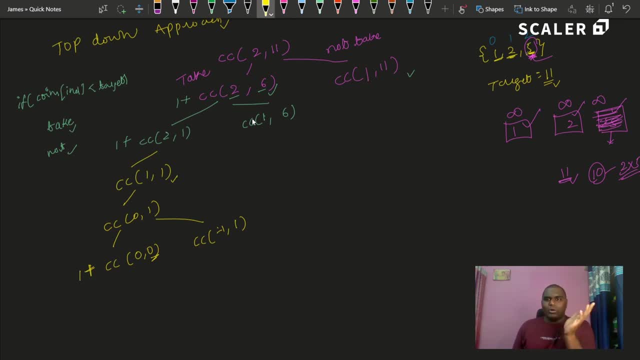 i got. it means that i got the change for what i'm looking for, what i'm looking for, what i'm looking for. it means that i got the change what i'm. it means that i got the change what i'm. it means that i got the change, what i'm looking for, so i will simply return zero. 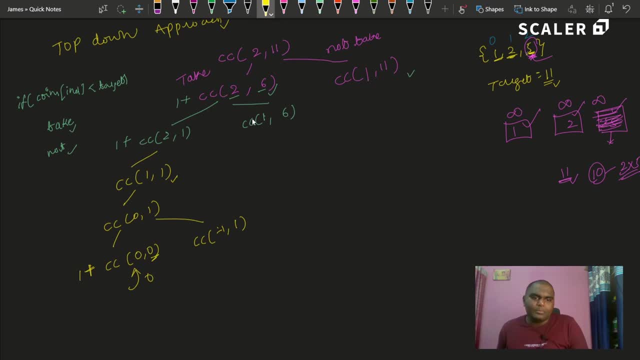 looking for, so i will simply return zero. looking for, so i will simply return zero here, here, here. okay, we'll simply return a zero here. okay, we'll simply return a zero here. okay, we'll simply return a zero here. so so, so you have written zero and one plus zero. 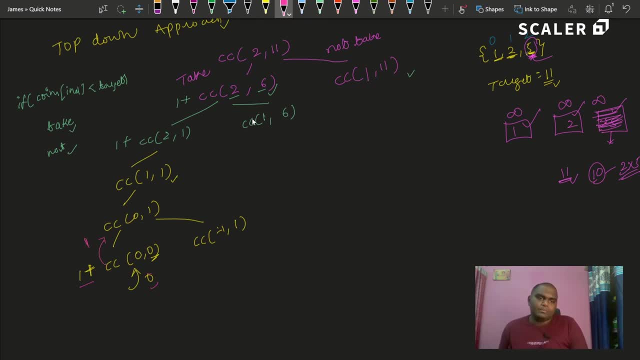 you have written zero and one plus zero. you have written zero and one plus zero. it's a one, so you will. it's a one, so you will. it's a one, so you will return one here. return one here. return one here. you will return a one here. now you have. 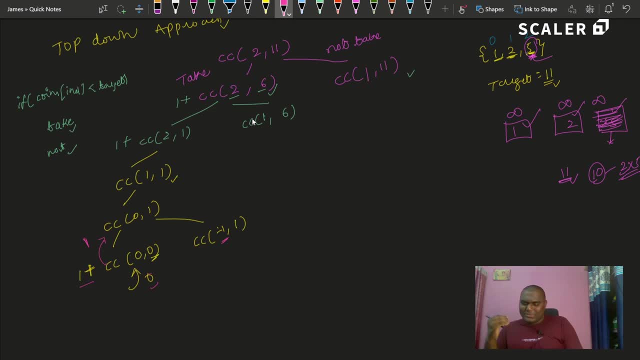 you will return a one here now you have. you will return a one here now you have seen a negative index, seen a negative index, seen a negative index. okay, since you have seen a negative. okay, since you have seen a negative. okay, since you have seen a negative index. what you need to do: 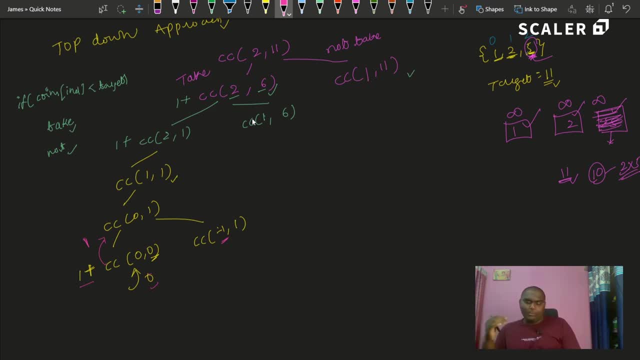 index what you need to do, index what you need to do, okay. so basically, since you are uh, you okay. so basically, since you are uh, you okay. so basically, since you are uh, you want a minimum number of coins, want a minimum number of coins, want a minimum number of coins so we can return something: a max value. 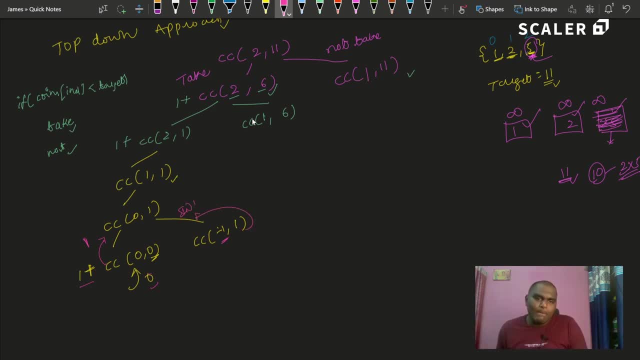 so we can return something, a max value. so we can return something a max value like uh into max into max, or 1 e 9 into max, or 1 e 9 into max or 1 e 9. so if you are returning 1 e 9, it might. 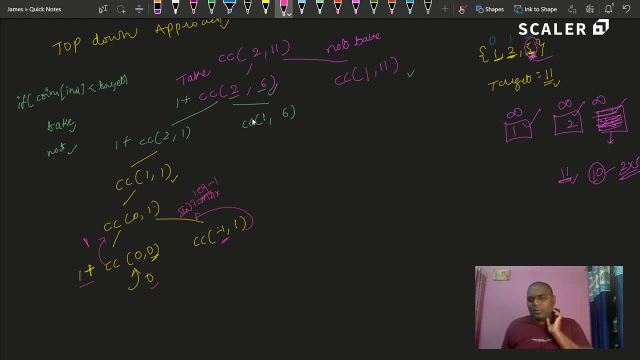 so if you are returning 1 e 9, it might. so if you are returning 1 e 9, it might get overflow. so just get overflow. so just get overflow. so just do minus one. it will, oh yeah, like that. do minus one, it will, oh yeah, like that. 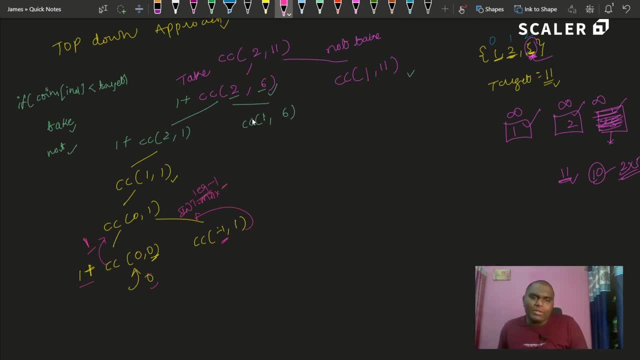 do minus one, it will, oh yeah, like that, okay, okay. okay, now you will consider minimum of these. now you will consider minimum of these. now you will consider minimum of these, both, both. both right, so minimum of these, both and you right, so minimum of these, both and you. 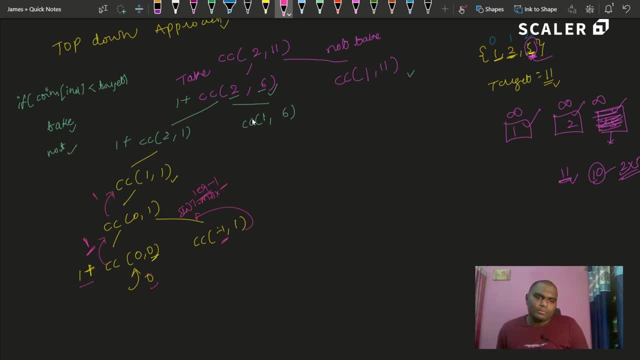 right. so minimum of these, both and you will return, one will return. one will return. one, so one. so one, so one, and here you will return. so you have only, and here you will return. so you have only, and here you will return. so you have only one option. 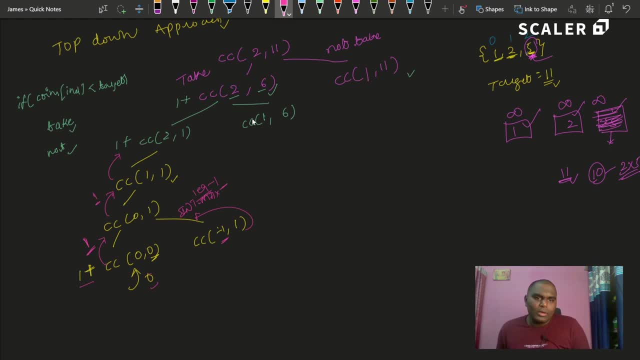 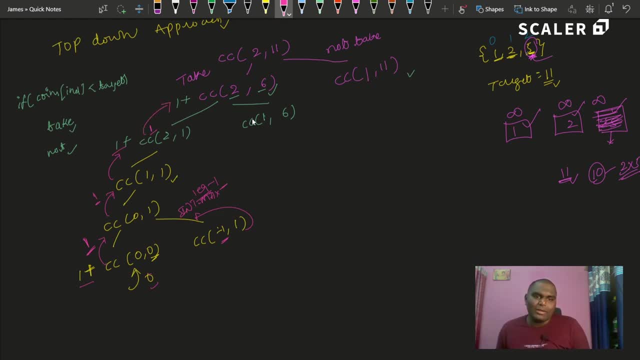 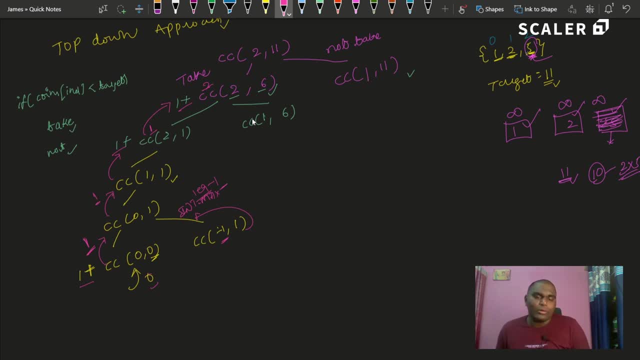 so from left side: okay, you got. so from left side: okay, you got uh three. right, so one plus sorry from uh three. right, so one plus sorry from uh three. right. so from left side you got two. left side, you got two. left side, you got two. okay. from left side, you got two. 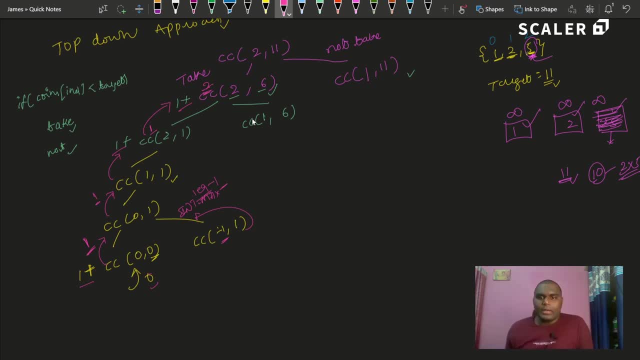 let's see here, and you are currently standing at this, and you are currently standing at this, and you are currently standing at this particular, particular, particular once index, and you want the sum of six once index and you want the sum of six once index and you want the sum of six. so 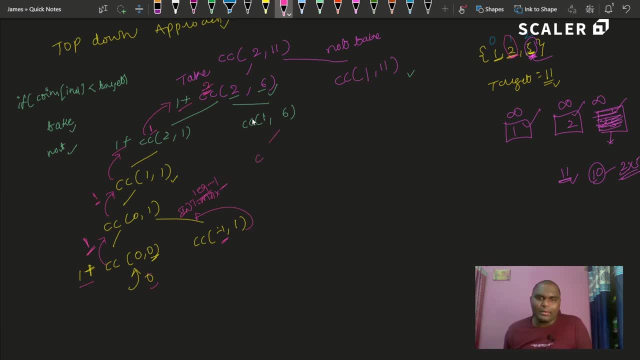 so so, two less than six: yes, so it means that two less than six: yes, so it means that two less than six: yes. so it means that you can take that guy, you can take that guy, you can take that guy. cc of one comma four. cc of one comma four. 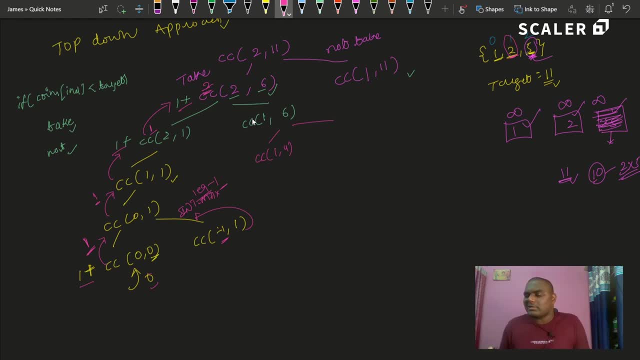 cc of one comma four, or or: or you, you might not, you are not you, you might not, you are not, you, you might not, you are not interested in that thing, interested in that thing, interested in that thing. so you will just move down and you will. so you will just move down and you will. 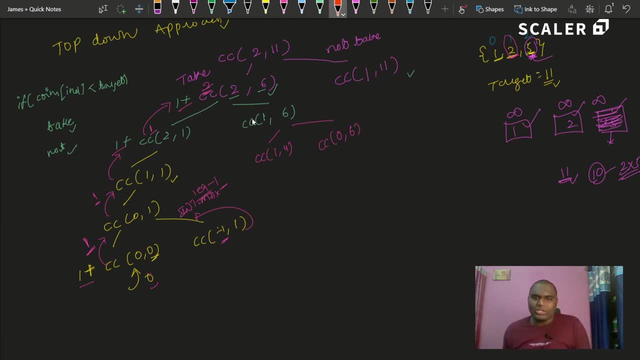 so you will just move down and you will keep that sum, keep that sum, keep that sum as it is now again. you are standing at as it is now again. you are standing at as it is now again. you are standing at here, since you have considered this, you. 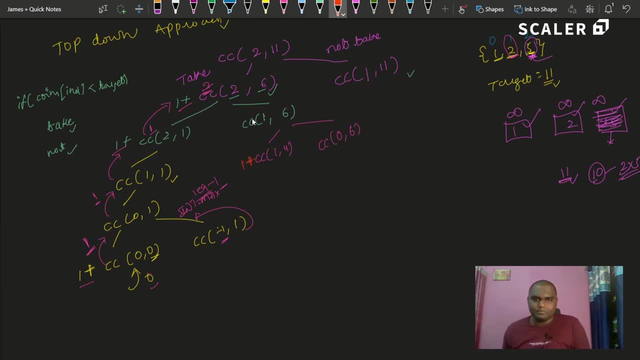 here, since you have considered this, you here, since you have considered this, you have to make, have to make, have to make plus one. okay, now, you came here and again, so you are now. you came here and again, so you are. now you came here and again, so you are standing at one and you want the sum of 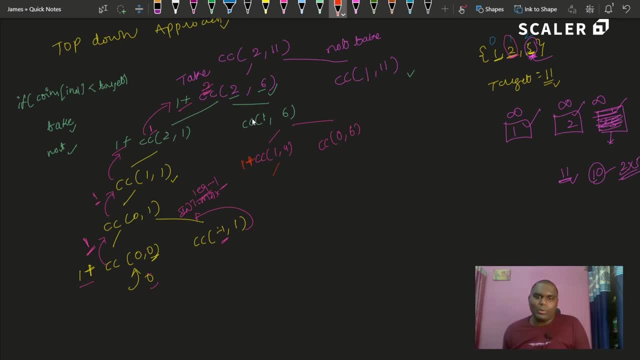 standing at one and you want the sum of standing at one and you want the sum of two, two, two, sorry four. so two less than four. again sorry four. so two less than four, again, sorry four. so two less than four again. you can consider that one plus cc. 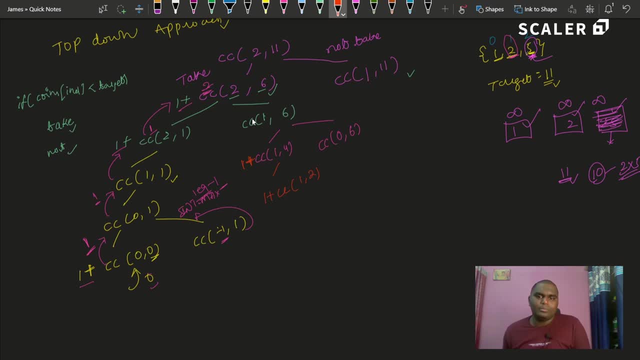 you can consider that one plus cc. you can consider that one plus cc, um, um, um, one comma two. one comma two, one comma two. and it's your decision, you are not, and it's your decision, you are not, and it's your decision, you are not interested in that. so zero comma four. 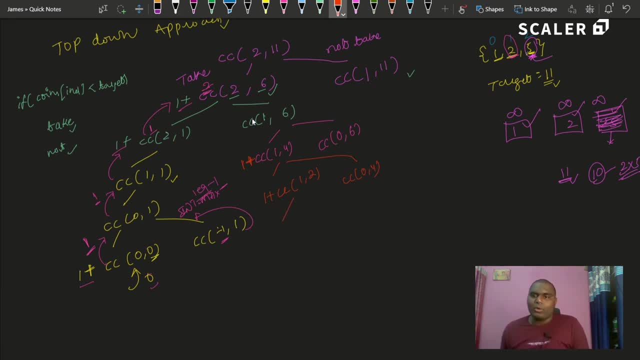 interested in that, so zero comma four. interested in that, so zero comma four. so again you came to left side and you. so again you came to left side and you. so again you came to left side and you will solve this and you are currently will solve this and you are currently. 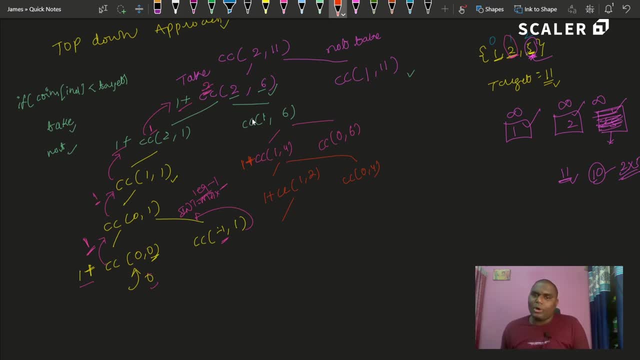 will solve this. and you are currently standing at one index means at second. standing at one index means at second. standing at one index means at second point, point, point. and you want the target of two, so again, and you want the target of two, so again. and you want the target of two, so again. it's less than or equal to, it's an. 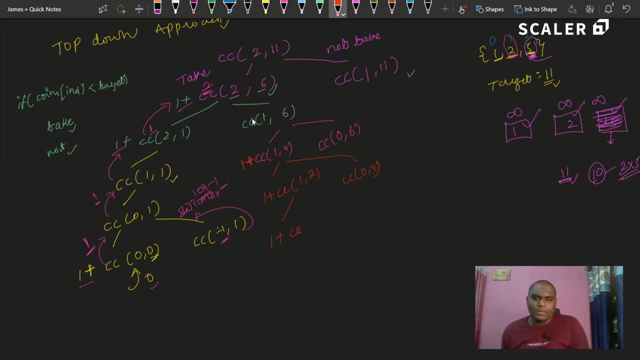 it's less than or equal to it's an it's less than or equal to it's an valid thing. so one plus valid thing. so one plus valid thing. so one plus cc, cc, cc, and and and one comma zero. one comma zero, one comma zero, and here your target sum became zero. so 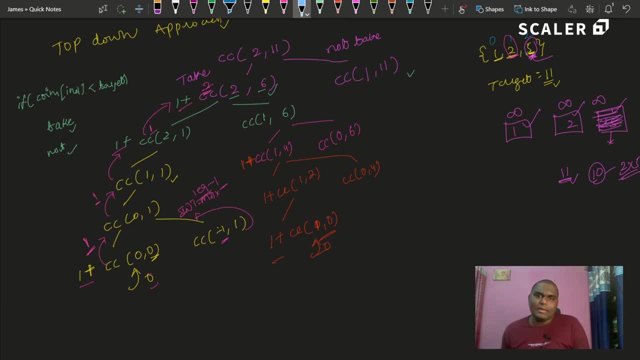 and here your target sum became zero. so, and here your target sum became zero. so you will return a zero here, one plus zero. you will return a zero here, one plus zero. you will return a zero here, one plus zero. it's a, it's a, it's a one, so you will return one here, so one. 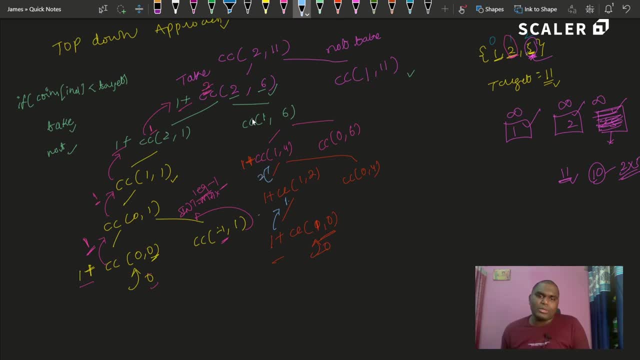 one, so you will return one here. so one one, so you will return one here. so one plus one, it's a two, so you will return. plus one, it's a two, so you will return. plus one, it's a two, so you will return two here. one plus two, it's a three, so you. 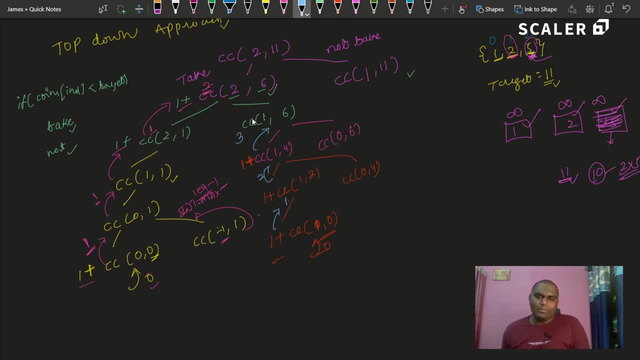 two here, one plus two, it's a three. so you two here, one plus two, it's a three. so you will return three here, will return three here, will return three here from a left side. okay, okay, so did i forgot something here? so okay, so did i forgot something here? so? 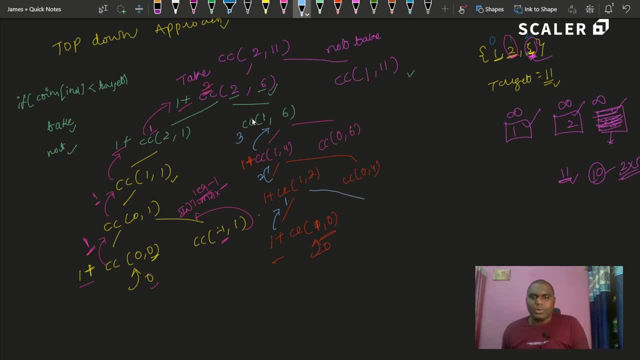 okay, so did i forgot something here? so it's your wish as well, like here, okay. it's your wish as well, like here, okay. it's your wish as well, like here, okay. so if you wish not to take this, so, if you wish not to take this. 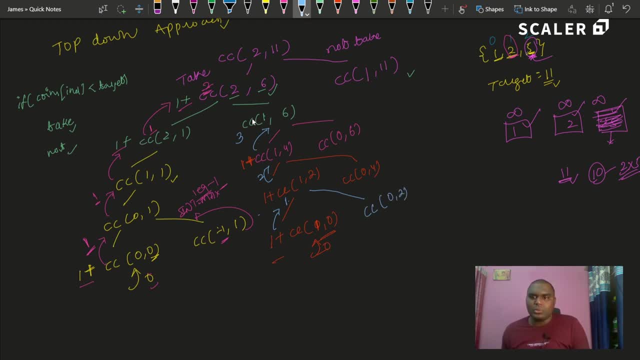 so if you wish not to take this, it will be a zero comma two. okay, so it will be a zero comma two. okay, so it will be a zero comma two. okay. so, if you are standing at a one, if you are standing at a one, if you are standing at a one, okay. so, if you are standing at one, if you. 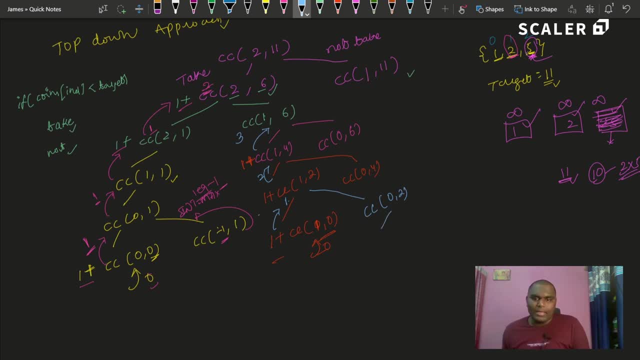 okay. so if you are standing at one, if you okay. so if you are standing at one, if you consider this, consider this, consider this and um. you can take up that, so cc of and um. you can take up that, so cc of and um. you can take up that, so cc of zero comma one. 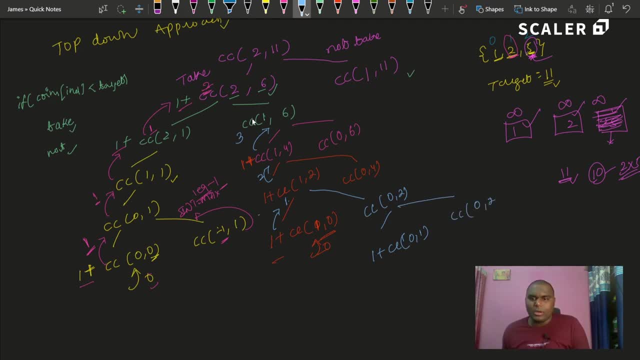 zero comma one, zero comma one. and if you wish not to take cc of zero and if you wish not to take cc of zero and if you wish not to take cc of zero, com, com, com, minus one comma two, okay, so, minus one comma two, okay so. 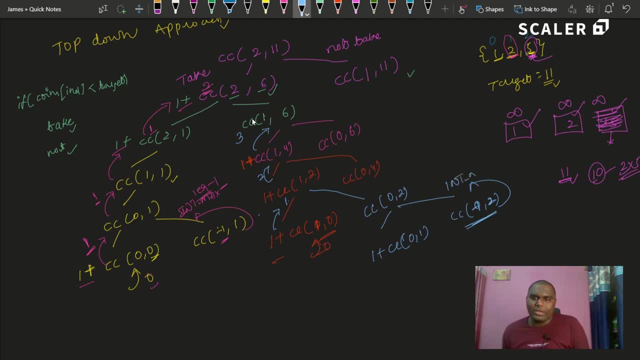 minus one comma two. okay, so it will return uh into max since you. it will return uh into max since you. it will return uh into max since you have reached uh, have reached uh, have reached uh. negative index: okay, and again you will go. negative index: okay, and again you will go. 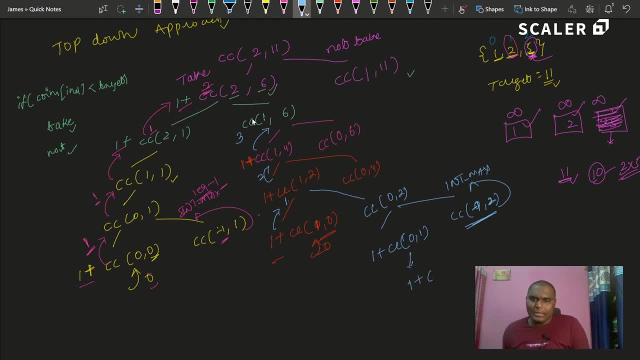 negative index. okay, and again, you will go here, here, here, and you can again consider that cc of a and you can again consider that cc of a and you can again consider that cc of a: zero, comma, zero, comma, zero, comma, zero, okay, zero, okay, zero, okay. so it will essentially have reached a. 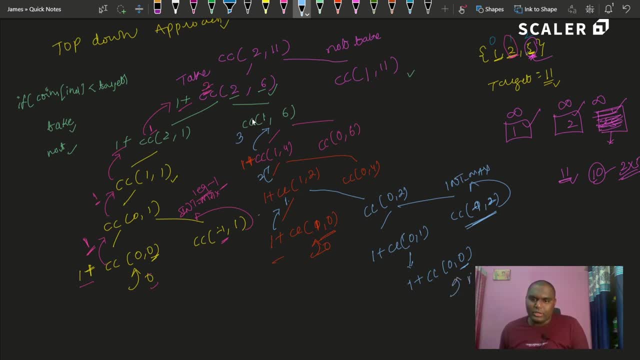 so it will essentially have reached a. so it will essentially have reached a zero, zero, zero. it will return in. it will return in, it will return in: sorry zero. and one plus zero it's a zero, sorry zero, and one plus zero it's a zero, sorry zero, and one plus zero it's a zero. so one plus zero it's a one. 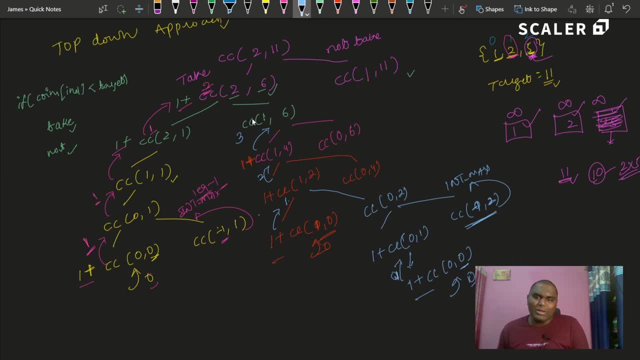 so one plus zero it's a one. so one plus zero it's a one. sorry, sorry, sorry. it will return one and one plus one. it it will return one and one plus one. it it will return one and one plus one, it will become two. yep, so, uh, minimum of these two, say two. 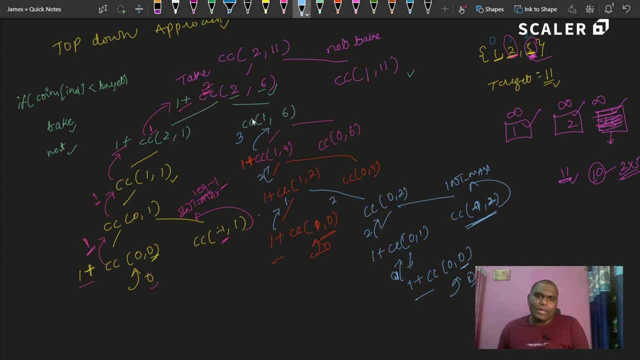 yep. so, uh, minimum of these two, say two. yep. so, uh, minimum of these two, say two. so, minimum of this one comma two. it's a so minimum of this one comma two. it's a so minimum of this one comma two. it's a one, so you will return one plus. 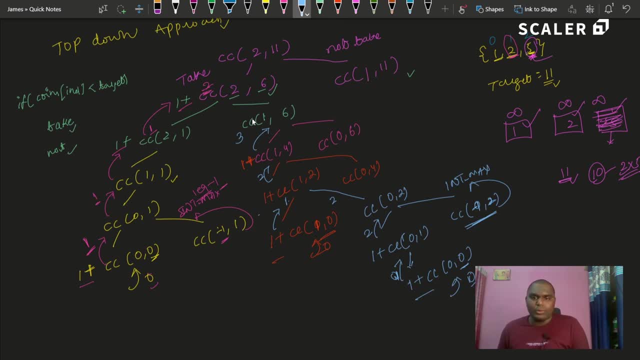 one, so you will return one plus one, so you will return one plus one, so it will be two. one, so it will be two one, so it will be two, and so you need to solve this, and so you need to solve this, and so you need to solve this. now let's say: 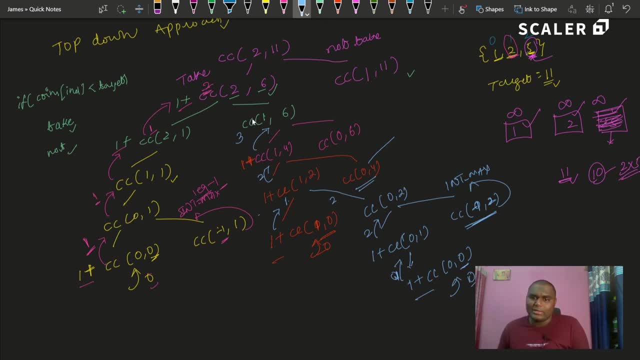 now let's say now, let's say you: um. so you are currently standing at you, um. so you are currently standing at you, um. so you are currently standing at second index, zeroth index, second index, zeroth index, second index, zeroth index, and you wish to solve this as a uh. 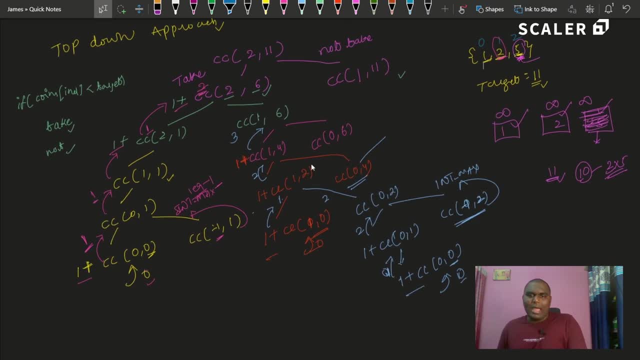 and you wish to solve this as a uh and you wish to solve this as a uh. four okay, so. four okay, so. four okay, so means that you have uh, means that you have uh, means that you have uh. five okay, so you have a one rupee coin. 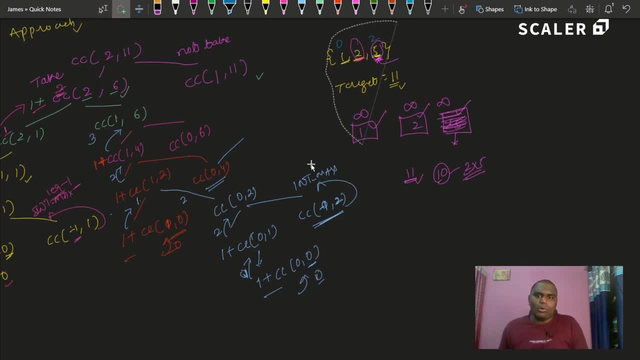 five. okay, so you have a one rupee coin. five. okay, so you have a one rupee coin. currently you are at one rupee coin. currently you are at one rupee coin. currently you are at one rupee coin and you want to make the change of four. 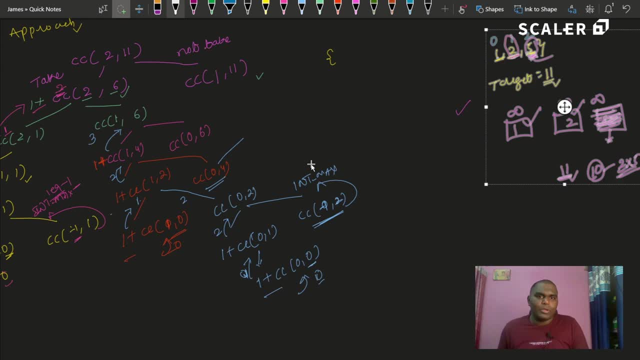 and you want to make the change of four. and you want to make the change of four. so that is possible, right, that is so, that is possible, right, that is so, that is possible. right, that is possible, possible, possible. so you will say 0.3, 0.3. 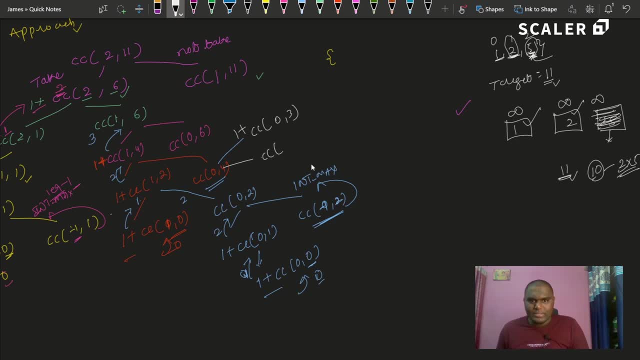 0.3 and if you wish 0.3 and if you wish 0.3 and if you wish not to take that, not to take that, not to take that, it will be cc of minus one comma three. it will be cc of minus one comma three. 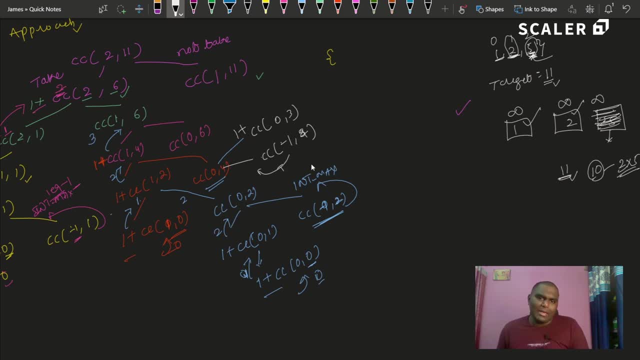 it will be cc of minus one comma three, oh sorry four, oh sorry four, oh sorry four. so it will return into max. so you will go this thing. or cc of cc of a zero comma: a two so one plus sorry, so again. a two so one plus sorry, so again. 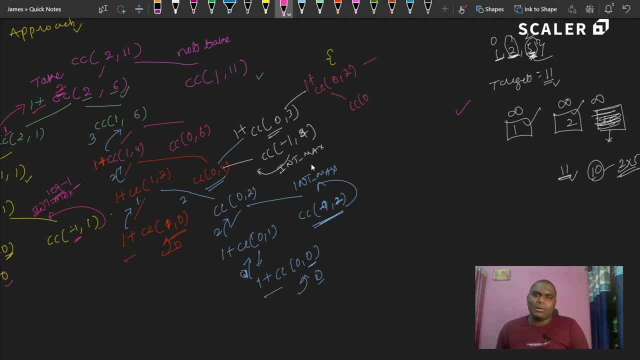 a two, so one plus sorry, so again, uh it will. if you wish not to take this, uh it will. if you wish not to take this, uh it will. if you wish not to take this cc of cc of cc of minus one comma r2, minus one comma r2. 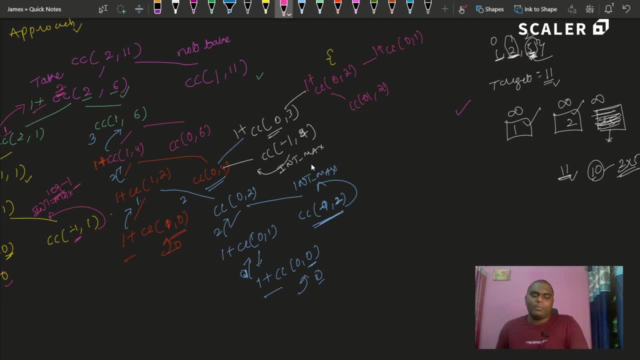 minus one comma r2. so if you wish to carry on and zero, so if you wish to carry on and zero, so if you wish to carry on and zero, comma one, comma one, comma one. and you are currently standing at one to and you are currently standing at one to. 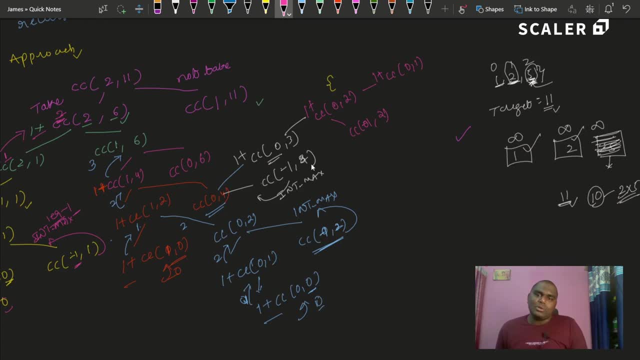 and you are currently standing at one to be coin and you want one to be changed. be coin and you want one to be changed. be coin and you want one to be changed. and also again if you wish not to take. and also again if you wish not to take. 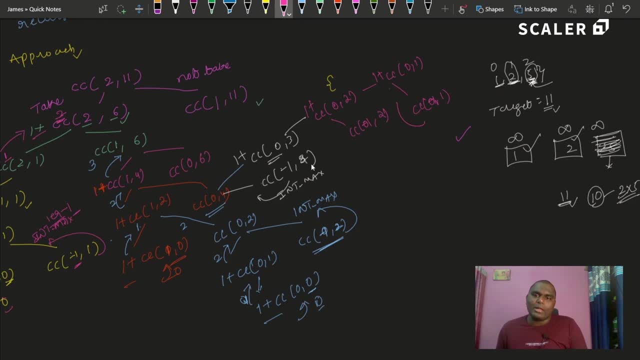 and also again, if you wish not to take this, and it will return minus one comma this, and it will return minus one comma this, and it will return minus one comma one. so it will return into max here, it will return into max and you will go again. so here, 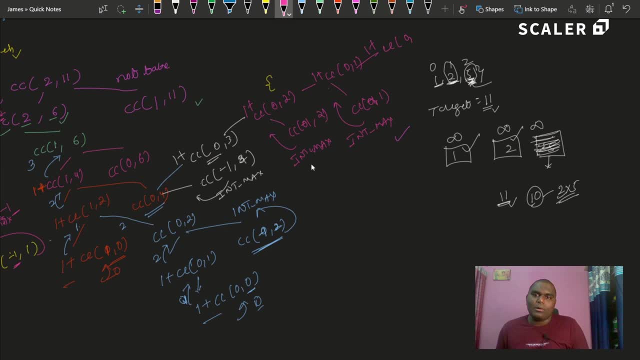 and you will go again. so here and you will go again. so here again, you can stand at a one plus cc again. you can stand at a one plus cc again. you can stand at a one plus cc of of of zero, zero, and you wish not to take up. 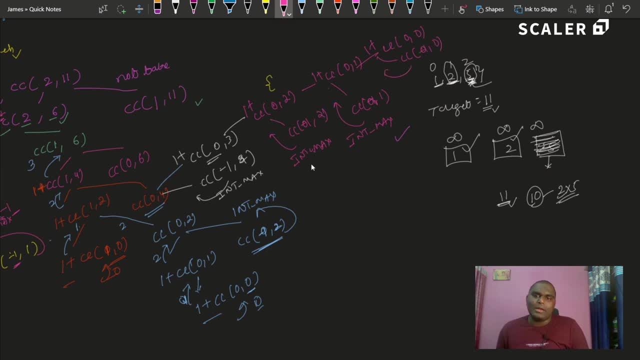 zero, zero, and you wish not to take up zero, zero, and you wish not to take up this, this, this, and minus one comma zero, so it will, and minus one comma zero, so it will, and minus one comma zero, so it will return into max, return into max. 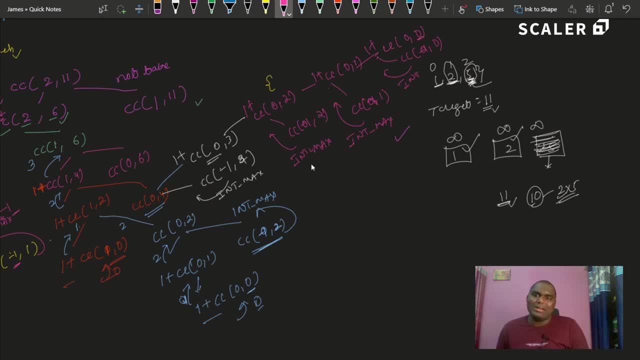 return into max, it will return one. so since you have it will return one. so since you have it will return one. so since you have reached some zero, it will return zero. reached some zero, it will return zero. reached some zero, it will return zero. so one plus zero it's a one, so it will. 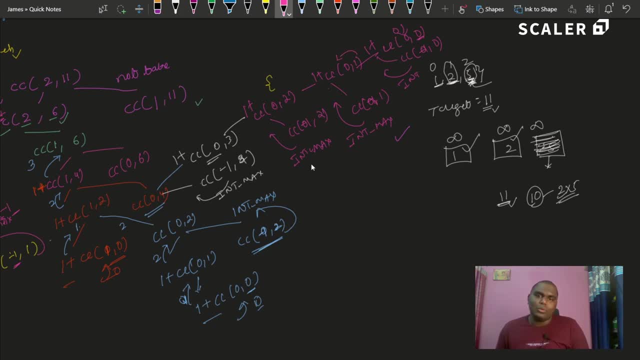 so one plus zero. it's a one. so it will so one plus zero. it's a one. so it will return one, return one. so one plus one. it will be two. so it will so one plus one. it will be two. so it will so one plus one. it will be two, so it will return two. 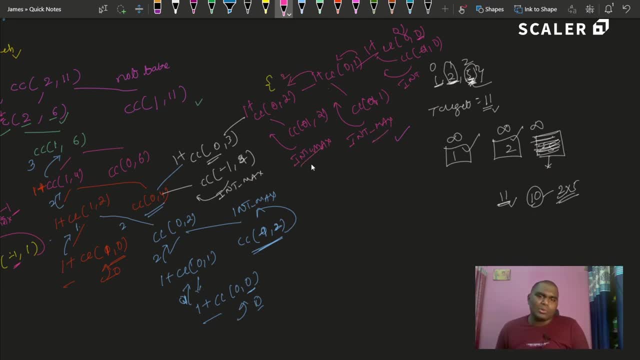 return two, return two. so again it's a max, max, max and all so. so again it's a max, max, max and all so. so again it's a max, max, max and all. so it will be a one plus two, it's a three. it will be a one plus two, it's a three. 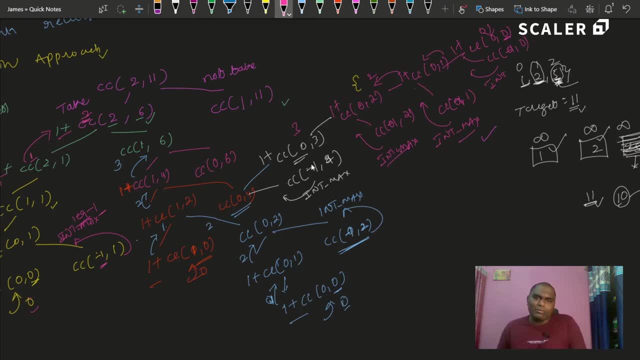 it will be a one plus two, it's a three. so so so yeah, so in max of uh, yeah, so in max of uh, yeah, so in max of uh three, a minimum of three comma into max three, a minimum of three comma into max three, a minimum of three comma into max. so it will be three. so one plus three. 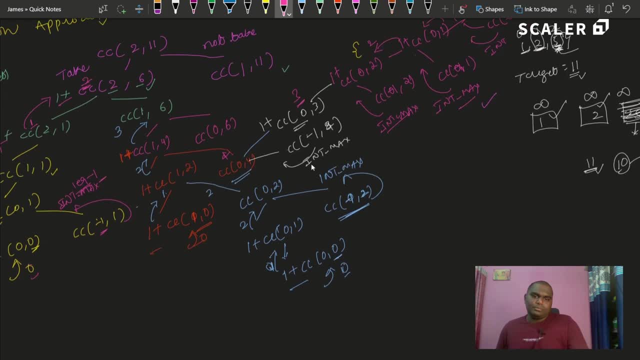 so it will be three. so one plus three. so it will be three, so one plus three. it's a, it's a, it's a four. so uh, here four. so uh, here four. so uh, here four, four. so uh, here four, four. so uh, here four. okay, so two comma four, it's like two. 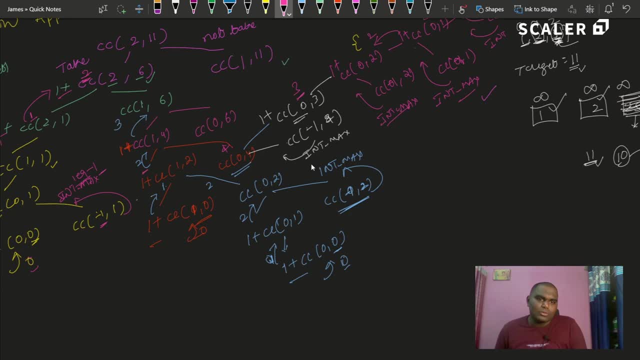 okay, so two comma four, it's like two. okay, so two comma four, it's like two. okay, minimum is two. so okay, minimum is two. so okay, minimum is two. so um here, one plus two, it's a three. um here, one plus two, it's a three. 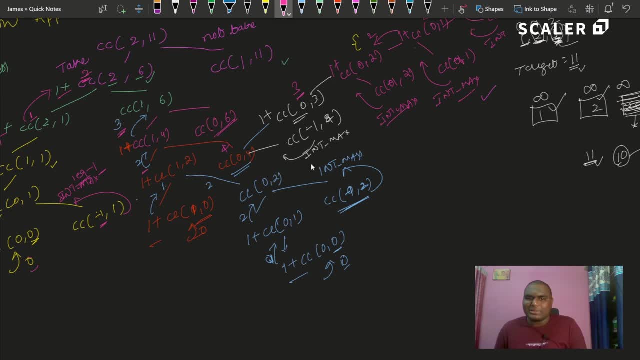 um, here, one plus two, it's a three. okay, so again you need to traverse on. okay, so again you need to traverse on. okay, so again you need to traverse on this side, this side, this side. so i'm not making this. so i'm not making this. 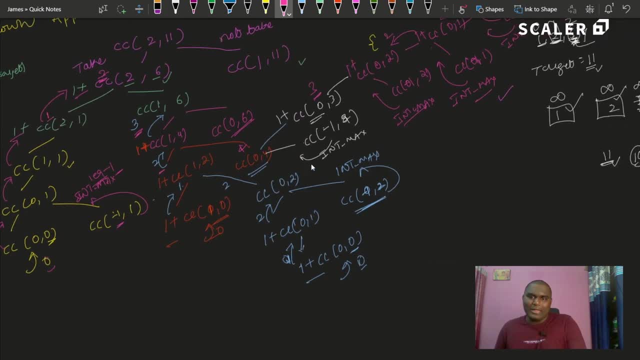 so i'm not making this. okay, so it's already a mess. okay, you okay. so it's already a mess. okay, you okay, so it's already a mess. okay, you can, can, can. i hope you have figured out what is. i hope you have figured out what is. 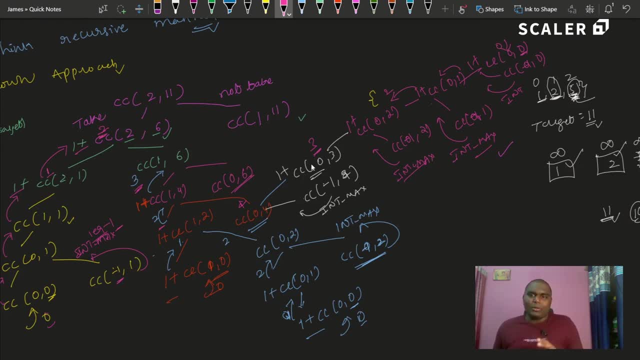 i hope you have figured out what is happening here, happening here, happening here: okay, so give it a shot. okay, you will okay, so give it a shot. okay, you will okay, so give it a shot. okay, you will get to know, so, get to know, so, get to know, so. so we are doing only three, three rules. 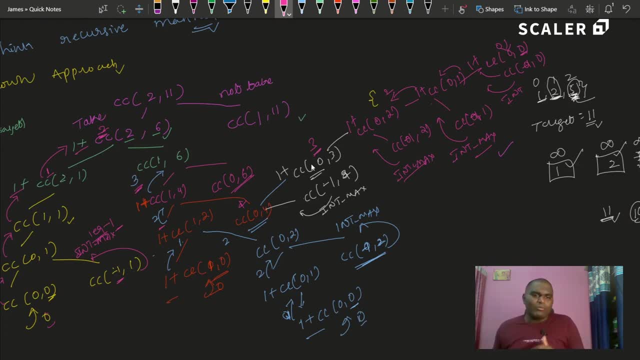 so we are doing only three, three rules. so we are doing only three, three rules. okay, i will let me summarize those. okay, i will let me summarize those. okay, i will let me summarize those. things, things, things, okay. so, before moving on, uh, let's assume okay. so, before moving on, uh, let's assume. 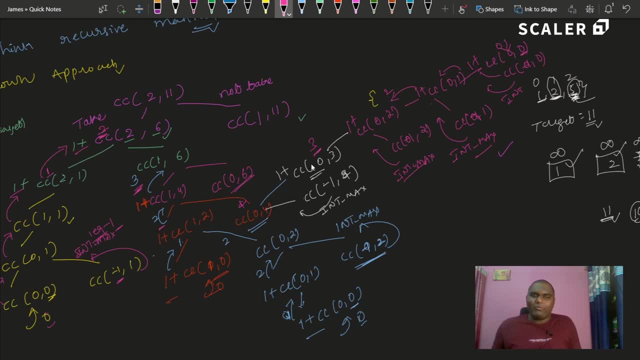 okay, so before moving on, uh, let's assume it has something written. it has something written, it has something written, and uh again, minimum will be three only. and uh again, minimum will be three only. and uh again, minimum will be three only. uh, we know that answer is three. so 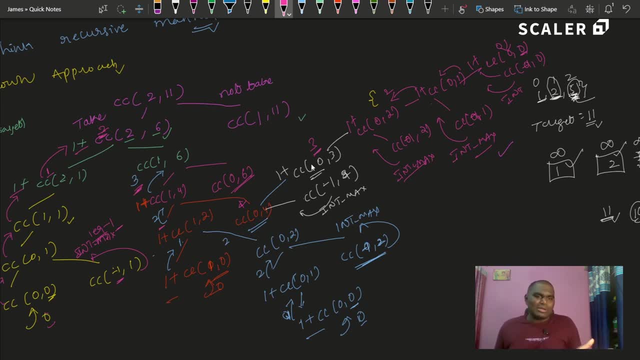 uh, we know that answer is three. so, uh, we know that answer is three, so anything. so i'm pretty much sure that anything. so i'm pretty much sure that anything. so i'm pretty much sure that nothing was less than three, so i will. nothing was less than three, so i will. 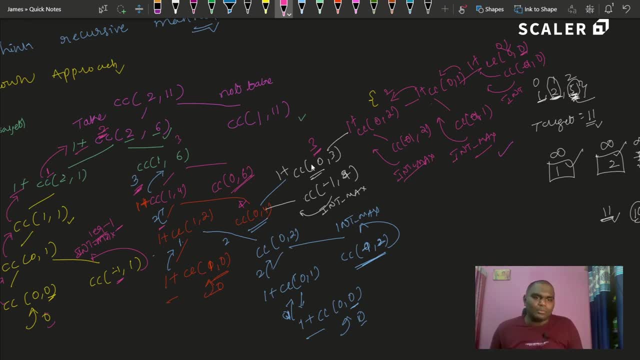 nothing was less than three. so i will return simply three here. return simply three here. return simply three here. and here i got a two, and here i got a two, and here i got a two. okay, so two is minimum, so one plus two. okay, so two is minimum, so one plus two. 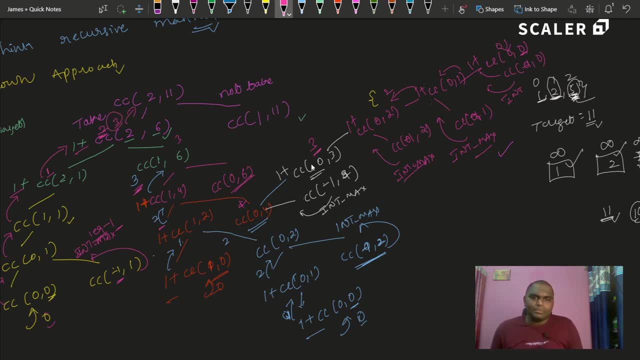 okay, so two is minimum. so one plus two, it's a three, it's a three, it's a three, so it will return three. so so it will return three, so so it will return three. so, uh, not take. uh, if you go on, carry on this, anyway you will get um three as. 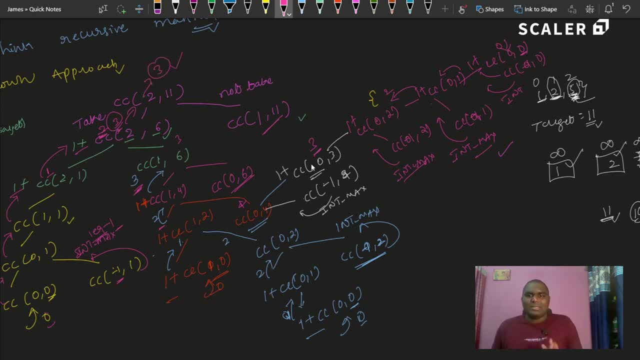 this. anyway, you will get um three as this. anyway, you will get um three as minimum, so it will turn three as your minimum. so it will turn three as your minimum. so it will turn three as your answer. so this is how it looks like okay answer. so this is how it looks like okay. 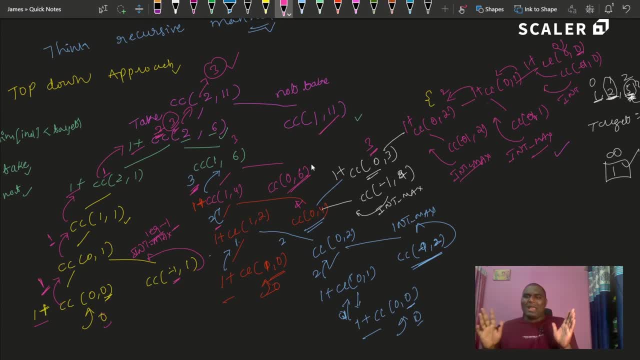 answer. so this is how it looks like. okay, so a big uh tree. okay, because you will so a big uh tree. okay, because you will so a big uh tree. okay, because you will be having a lot of combinations. that's be having a lot of combinations, that's. 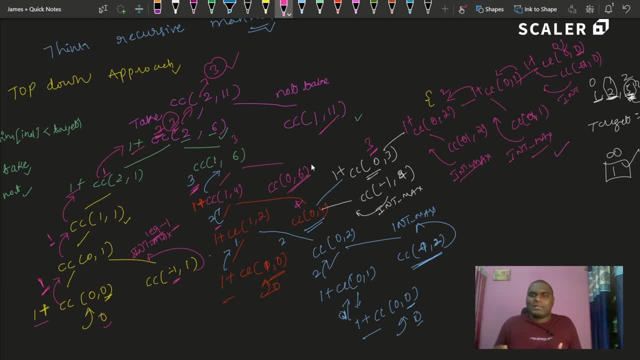 be having a lot of combinations. that's why, because, uh, you will be having, why, because, uh, you will be having, why, because, uh, you will be having infinite uh supply of coins- right, that is infinite, uh. supply of coins- right, that is infinite uh, supply of coins, right. that is the reason why you have. 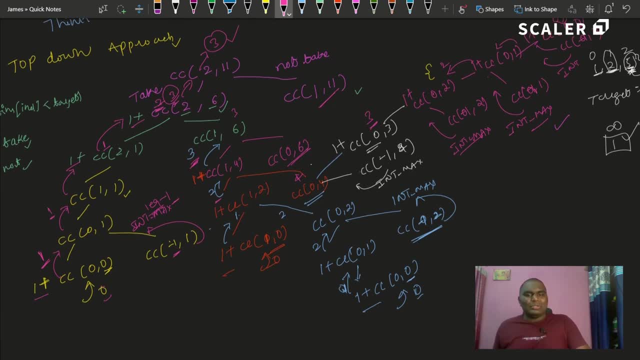 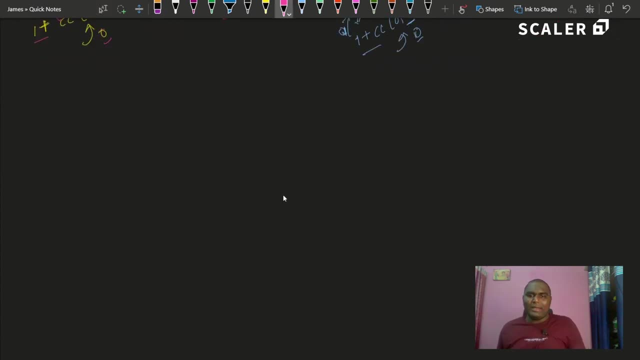 the reason why you have, the reason why you have this big recurrence tree. okay, so, let's this big recurrence tree. okay, so, let's this big recurrence tree. okay, so, let's go on. uh, try to code this up. go on, uh, try to code this up. go on, uh, try to code this up. okay, let me summarize what we have did. 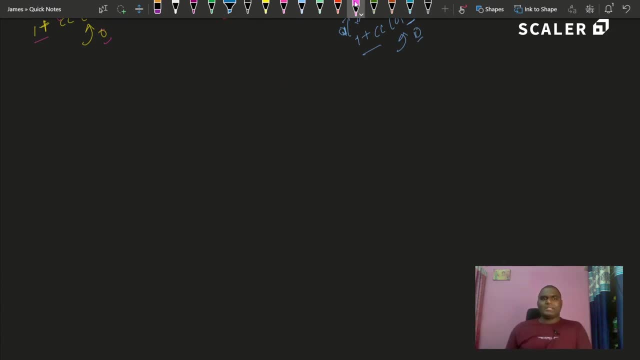 okay, let me summarize what we have did. okay, let me summarize what we have did so far. so far, so far. okay, so, basically, okay, so, basically, okay. so, basically, we have a function called a coin change, we have a function called a coin change. we have a function called a coin change where we will be having a index. 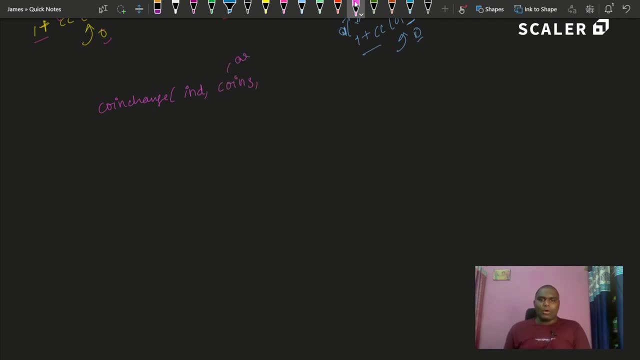 where we will be having a index, where we will be having a index, and a coins means it's an array or a and a coins means it's an array or a and a coins means it's an array or a vector, vector, vector, and this is an integer and you will be. 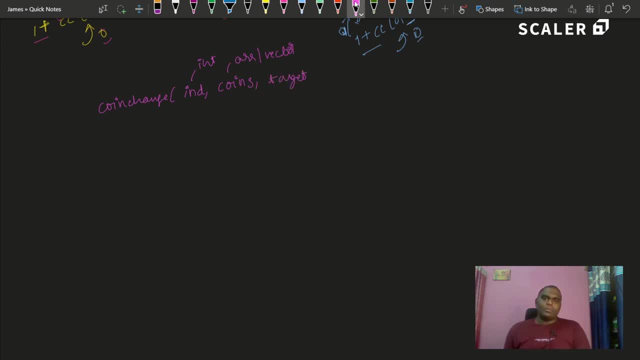 and this is an integer, and you will be- and this is an integer- and you will be having an having an having an target value: okay, target value, okay, target value. okay, either, and it's an integer now, you either, and it's an integer now, you either. and it's an integer now you will be entering into this particular. 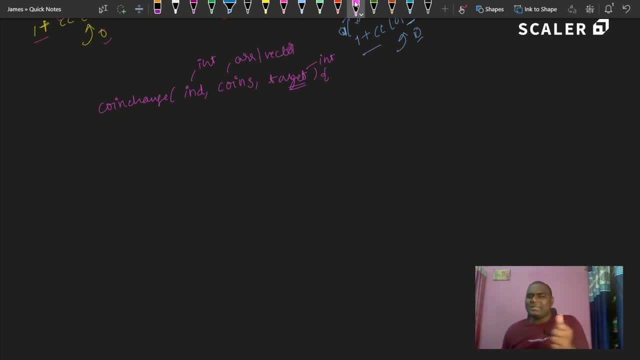 will be entering into this particular, will be entering into this particular function, function, function. and first so what will be our base case and first so what will be our base case and first so what will be our base case. figuring out the base cases. figuring out the base cases. 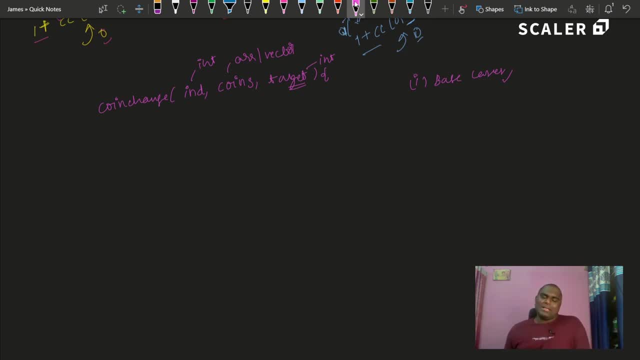 figuring out the base cases. first thing: sigma rolling uh recursion. first thing: sigma rolling uh recursion. first thing: sigma rolling uh recursion. okay, so base cases. so uh, can i say: okay, so base cases. so uh, can i say my first base case would be: what if my target equal to equal to zero? what if my target equal? 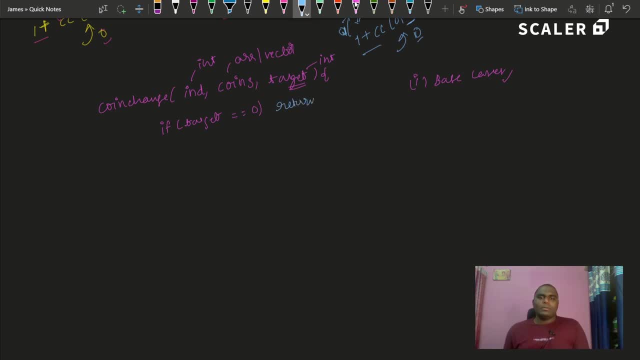 to equal to zero, and i say simply return zero because i don't require any coins. right so to make uh the sum of zero target of zero, you don't require any coins. that's an simple one base case. and next, so what? if so, since i am starting uh my index at the max thing, so what i can reach so till. 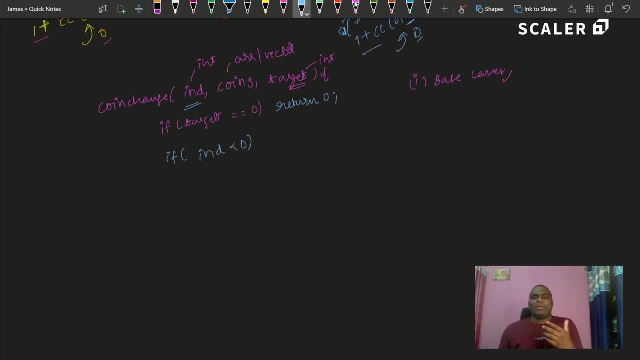 i can reach index less than zero. so whenever my index less than zero, it means that i have reached a negative index. so can i say: whenever i have seen a negative index, i can simply return into max. so because i am- uh, i am aiming for minimum answer. so 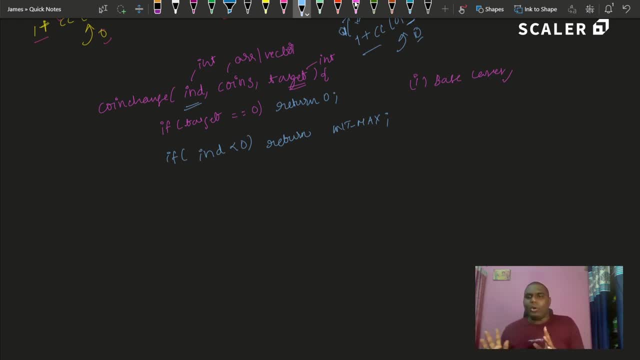 i am returning in max, so you know it will be going to be, and not in my answer. cool and yeah, these are all the two base cases. okay, base cases. now. our actual logic comes here. now, first thing. so it has passed these both. now what you need to. 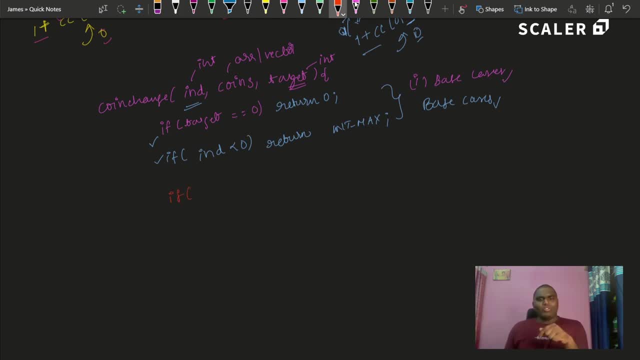 check. so you need to first check the coin which you're currently standing is less than zero. so you need to first check the coin which you're currently standing is less than zero. less than the target or not means, let's say, you have a currently on coin of five rupees and you 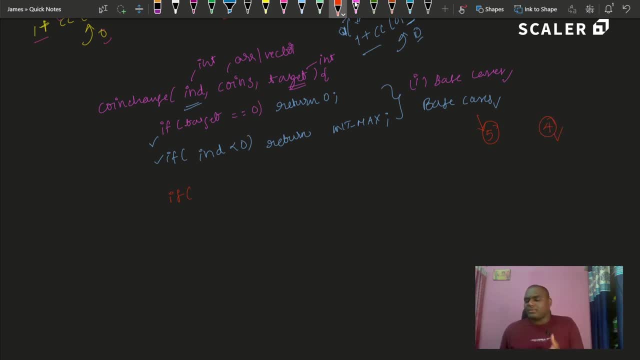 want the sum of a fourth. okay, your target is four. now, obviously you can't include five in that particular. uh answer, right, target, right to make that target, right. so what you can do. so, let's say, whenever coins of that particular index greater than a target target greater than target, then you, you can't include that coin. so simply what you. 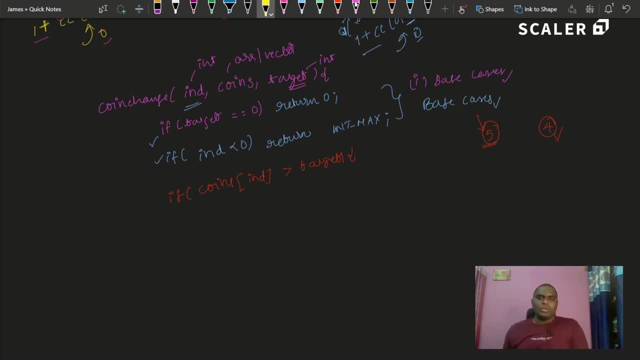 what you need to do? we just need to go to another coin. so simply return a coin, change coin, change uh, index minus one coins and mount come out. that's it. so what if this is false? okay, so coins is less than target, less than are equal to target as well. then what you need to do? you need to include that in your answer. 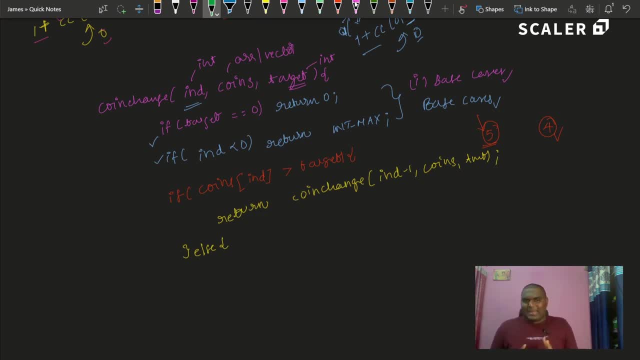 that is one choice, okay, so it is less than okay now. uh means like: um, you are currently standing at two and you want the sum of four, target of four, so it is possible. now it's your choice to whether to take that answer in or to take that two coin into. 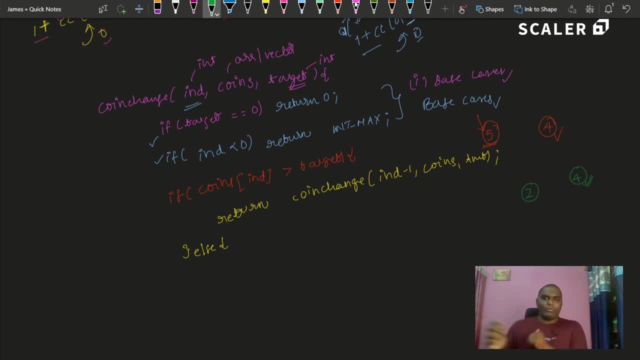 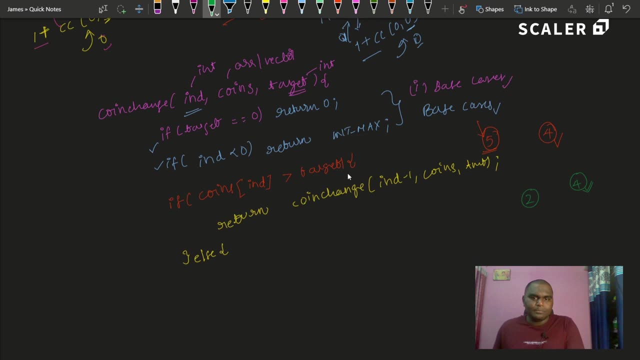 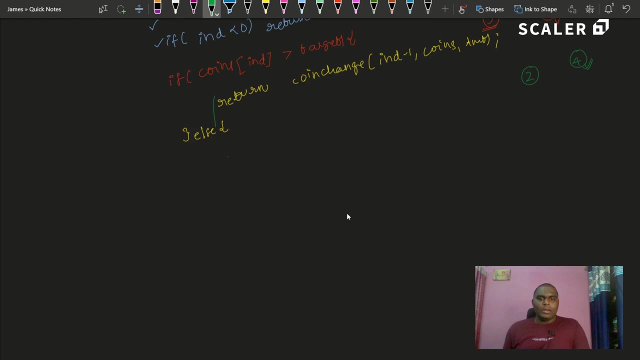 your four or not to take that coin into your four. okay, so let's say i will have a two. uh, variables, okay, are two variables. let's say in a take. okay, so if i take that coin i must need to keep track of that, right? so one plus. i just need to increase my coins. so one plus coin change. 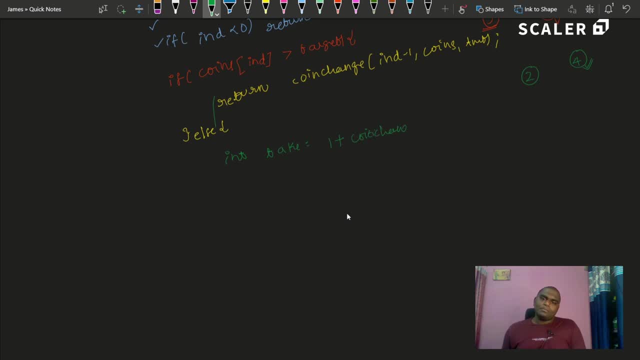 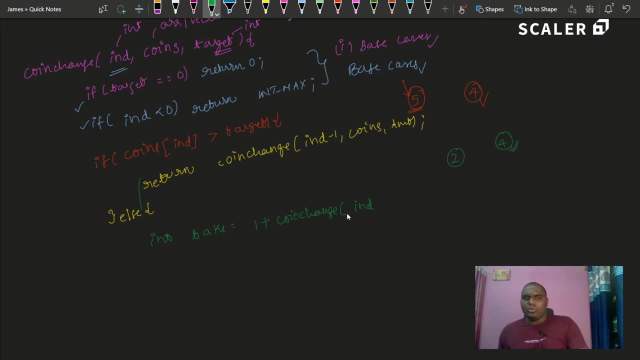 coin change. uh, if i include that, if i include that coin, now what i need to do? so? so, since i have infinite supply of coins, i need to keep a stay there itself. that is what we have seen in the currency right, so i will be staying there. i'm not increasing or decreasing my 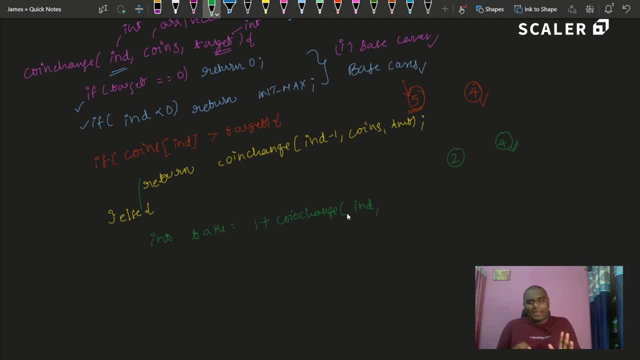 index. i'm sharing there only and my coins are coins like, so whatever i got the coins, i will be supplying that and so if i consider that into my answer means a target, i just need to make that target minus points of index, agree. so, uh, if i include that, i have to remove that from my target. 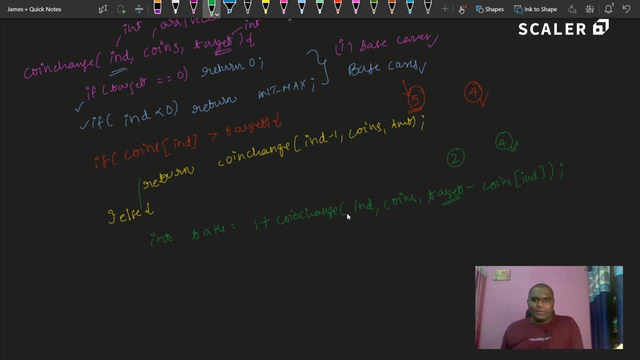 right, then only i can make it that to a zero until the comsommes enough, and then i can keep my coins to the zero target only, and if i wait for like about an hour, then it increases the trading price. if i include that, i have to remove that from my index. right, then only i can make it that to a zero. 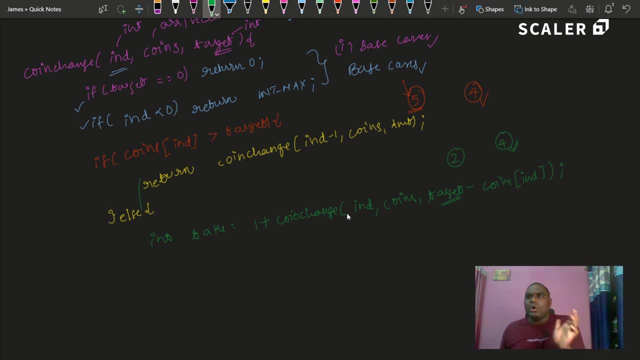 so our agenda is to make the target equal to zero, and whenever we have assumed a target is zero, our job is done. we have found the change. this is for take. so what if I wish not to take? not take then what I need to do. so I don't need to increase my coins, so I 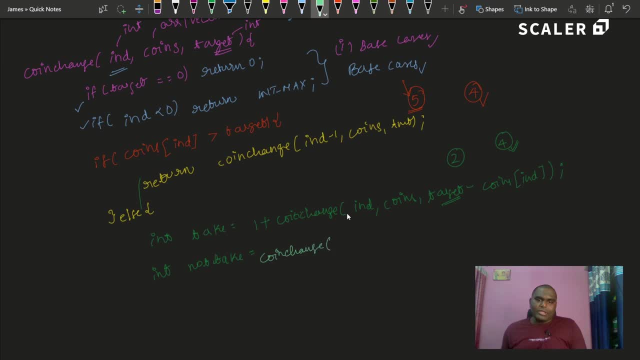 will simply call coin change. if I wish not to take that particular coin, I have to go to next coin. so index minus one coins target. I am not taking my, I am not considering that particular coin. that is the reason why I am not doing subtraction that particular coin. 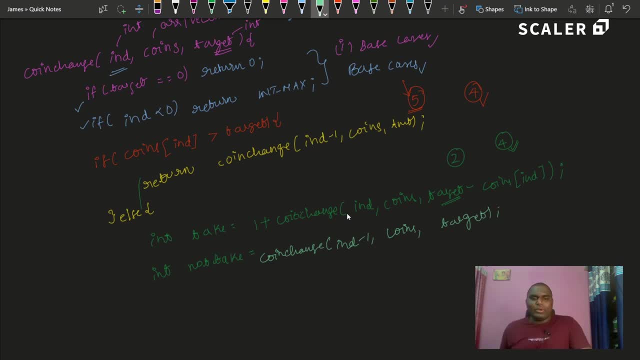 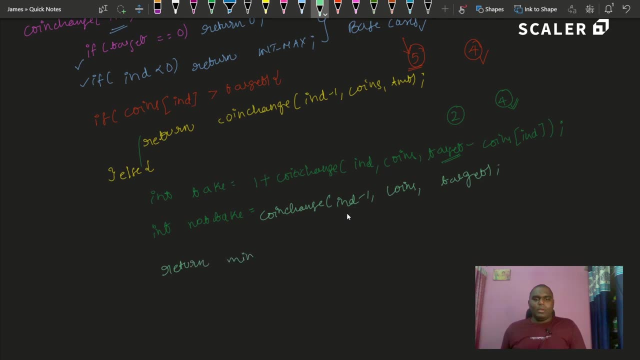 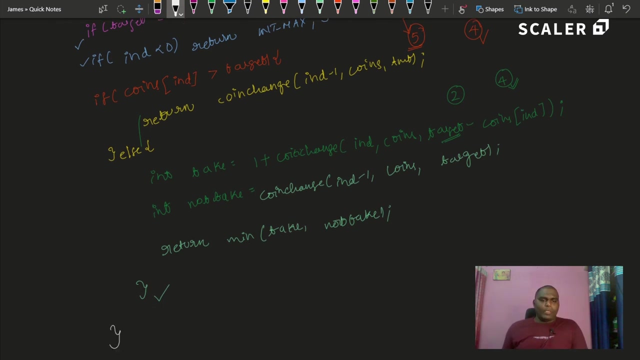 from my target. So, after making these two recursive calls, What I need to do? I need to simply return minimum of take comma, not take, agree, done, done, so, yeah, so did we figure out all the cases? did we figure out all the cases? no, I don't think. 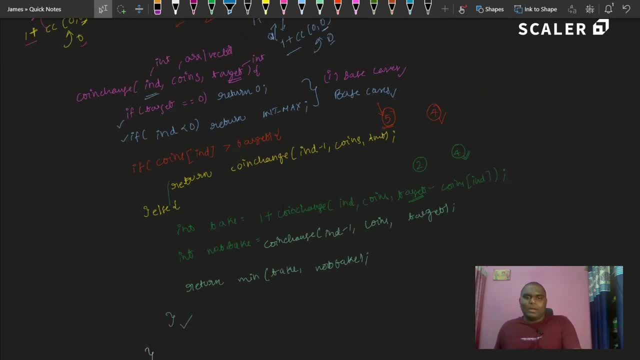 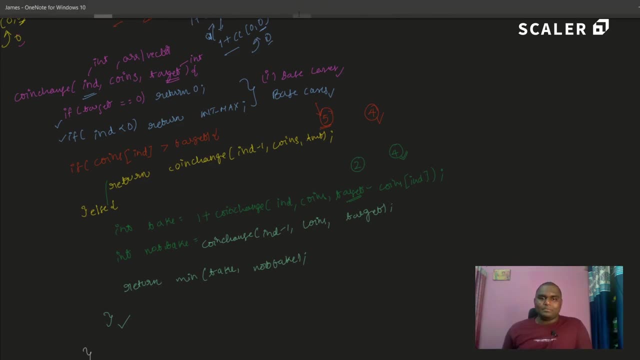 Why so? let's say: if you are in an interview, you have to ask this question in the beginning. okay, so let's say: I am, my target is thousand, let's assume thousand. and I have given you coins of coins of zero, one one. okay, Let's assume one one. 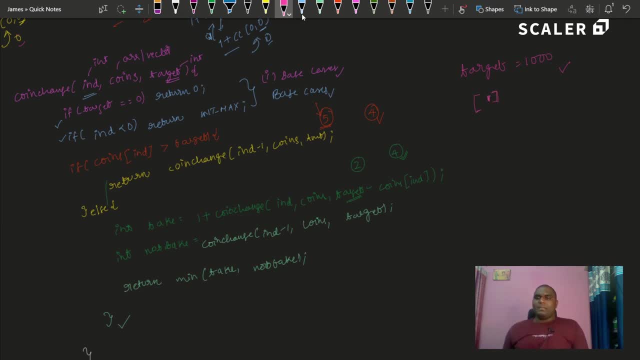 Okay, Let's assume one, or let's say: okay, so let's change this. okay, so I have given you in a target of three rupees, okay, target of three rupees, and I have given you these coins of two rupees. I have given you only two rupee coins and you need to make the target of three. 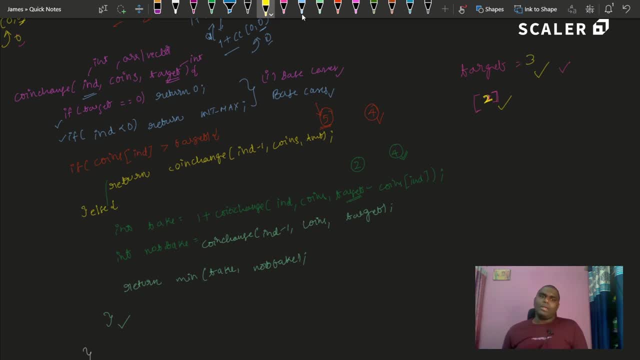 rupees now. is that a possible? no, that is not a possible right. So if you, If you take one two rupees coin, it will be minus one. okay, you still, you need a one rupee coin. and if you take a two, two rupee coins you have like you are giving four rupee change. 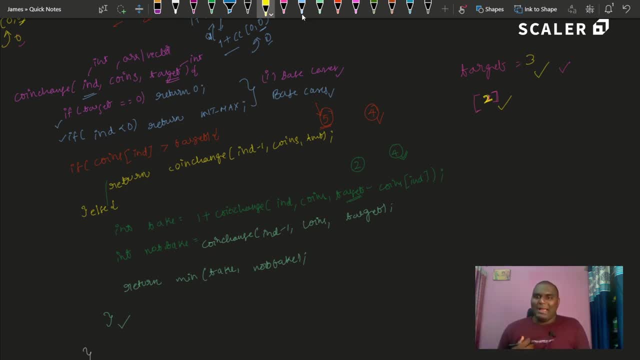 not three rupees. okay, So, as a shopkeeper, I am getting lost. okay, so I am not. yeah, I am not interested in that case. okay, so in that case, our answer will return into max. okay, so, into max, it will turn into max So. 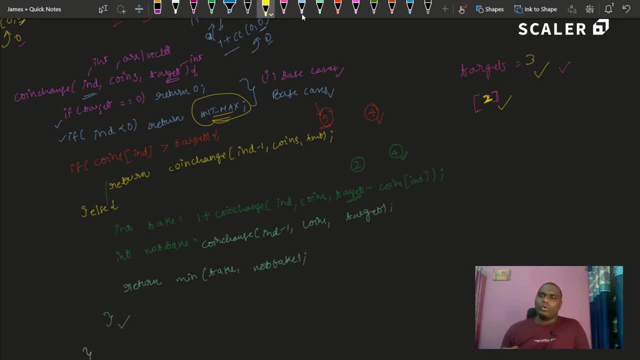 Okay. So it's your interviewer choice what to return, okay. so whether he wanted to return something like not possible or something, okay, it's interview choice. but mostly they will say return minus one. okay, If there is no particular answer, you can't make the choice for the like you can't make. 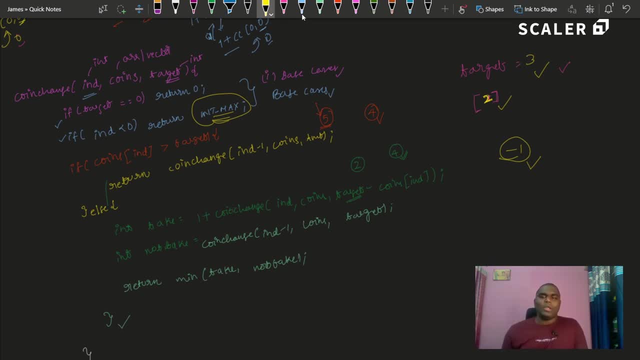 the change for the given target. just return minus one. okay, So in this scenario, I will return a minus one in my like main function. Okay, So now that's it for the code. okay, so let's quickly go on write the write the code for. 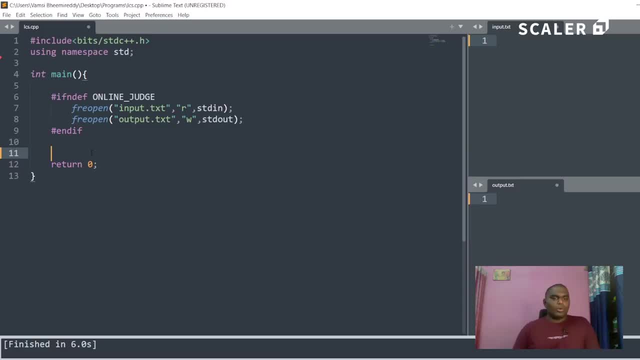 this particular approach. now let's try to code the approach, what we have discussed so far, okay. So the input format for this particular thing would be: you will be given a first n, okay, and you will be given then target. Then you will be given set of coins. 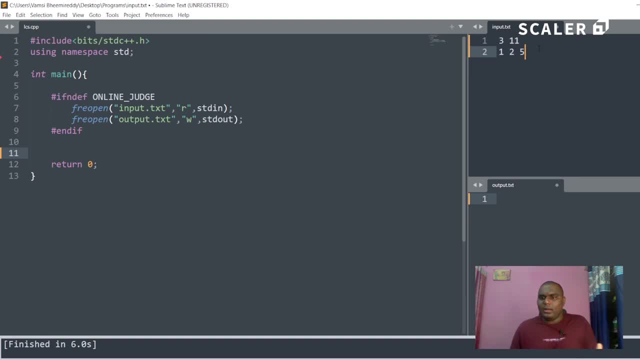 Okay, So it means our n target and a vector. okay, now let's try to accept that input. so int n target and you required a vector of this size, let's say coins of the size n. okay, and you need to accept them. Now we need to process our answer. so let's say we, let's assume we have a function called 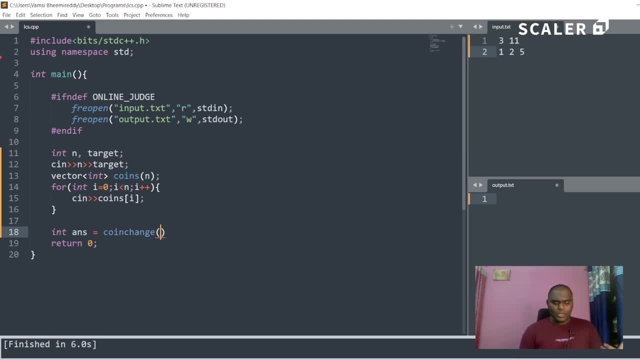 coin change and it is accepting index coins and target. so here we are passing index as n minus one. Okay, Now let's go and code this particular a function- change of index. and then we are int and then int target. Okay, First our first, our base cases. 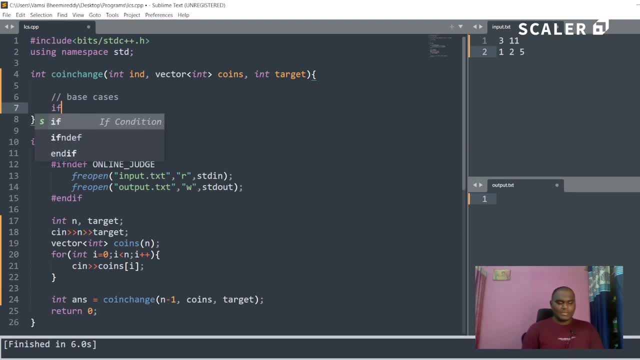 Okay, So first base cases: whenever our target is equal to zero, our target is equal to zero. simply, we are returning zero. our target is zeros. we are simply returning zero if our index are less than zero. index less than zero means and we are. we have seen an negative index. 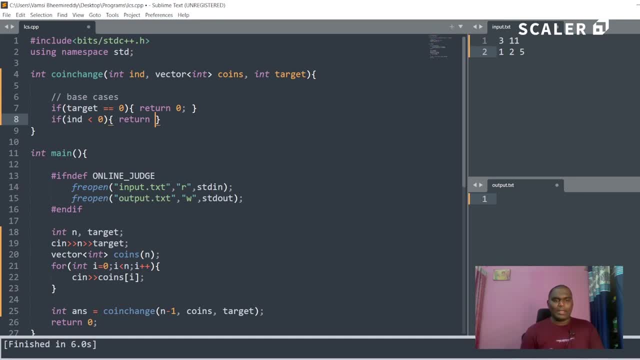 then what we need to do. so, as we have discussed, we are returning and maximum value. Okay, So here the maximum. so I'm going to consider int max, let's say a ten power nine. Okay, So if we return ten power nine, in some cases it might get into the overflow. 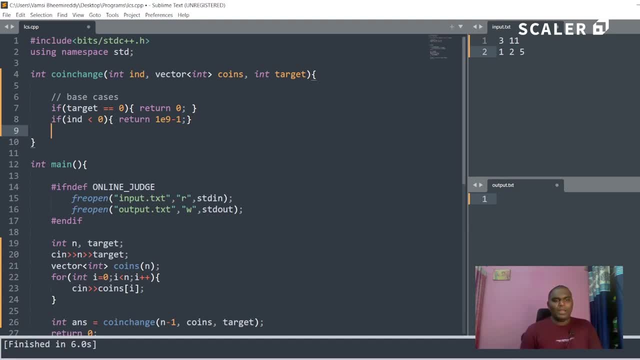 Okay, So we can do minus one second. Now. this is our base cases. now, what is the first case? what if a current coin is coin is Okay, Smaller, sorry, large, greater than what? greater than your target? if it is greater than your target, you must not include that. instead, you have to go to another coins. okay, other coins. 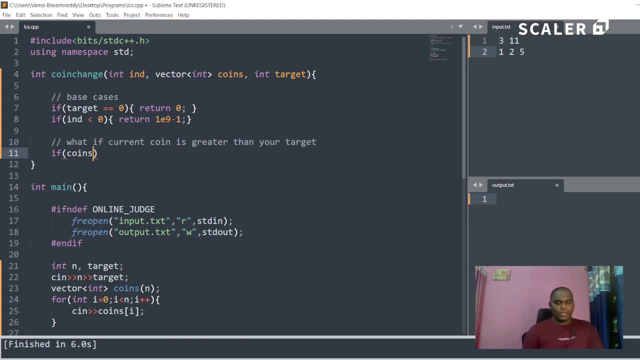 So if, if coins of index greater than at the target value, Okay, Then simply return coin change. we have to go to the next index means you are currently at index and then you, if you, if you have to go to the next index, then it is a coins, then 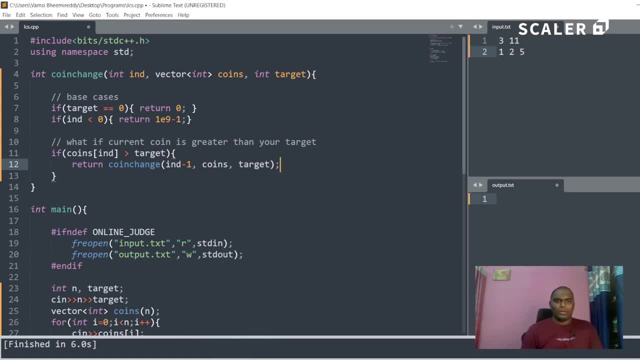 it is a target, so you are not including that value. so that is why you are keeping the target as it is. so if this is not the case- if this is not the case- means it's a less than so. it's like current coin is, and and if it is less than target, it means that you can include. 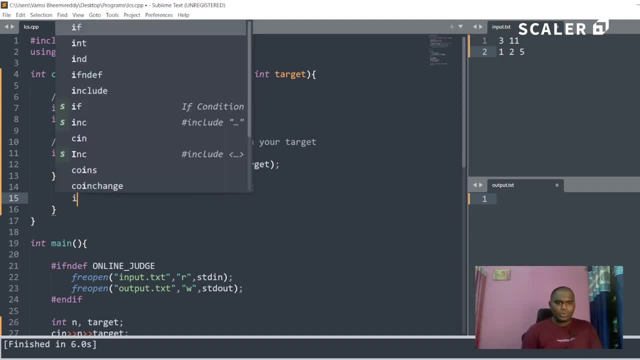 that or you can not include that. that's your choice. So let's say: int take, I can take that value, or I cannot take that value. Okay, That's a depends upon the choice. So if I include that value, okay, let's say I have decided to take that coin. so then what? 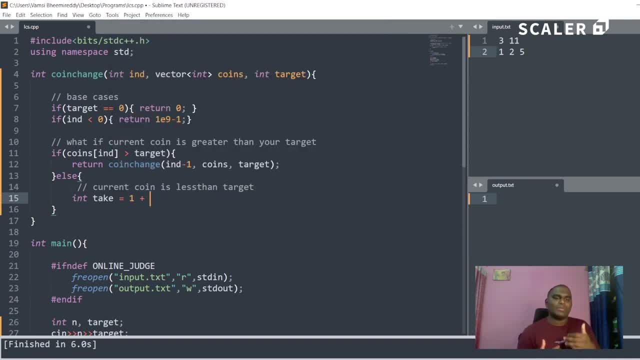 I need to do so. I have to include that I have to increase my count, right so? coin change, and again, do I need to go back to the next element or do I need to stay back here itself? I need to stay back here itself. why so? I have infinite set of coins, right so? so, though, if 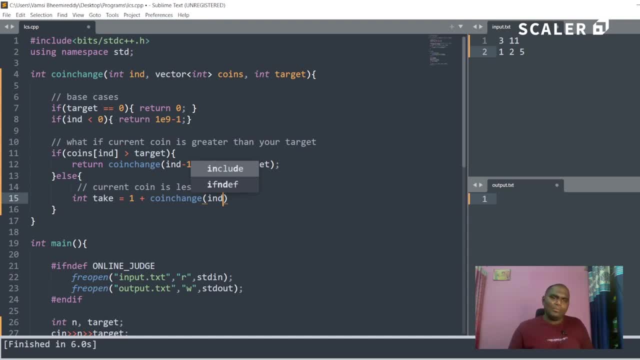 I consider that particular coin for the target I have to. I have to check again whether I can make another coin of this particular target coin, this as well. so that is why I will stay at this particular index. only then a coins now what I need to. 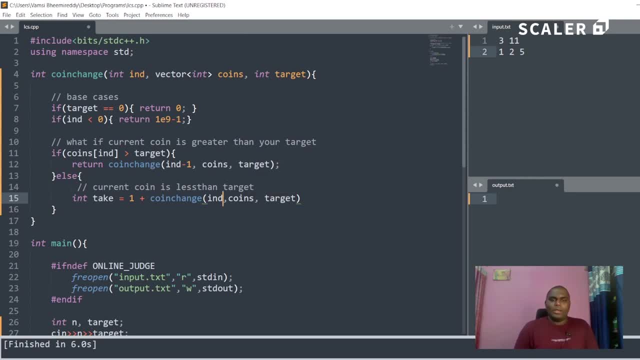 do so. I have taken that coin. okay, I have taken that coin. if I have taken that coin, what do I need to do? I have taken that coin. what do I need to do? I need to include: I have to decrease that particular coin. is that particular coin? 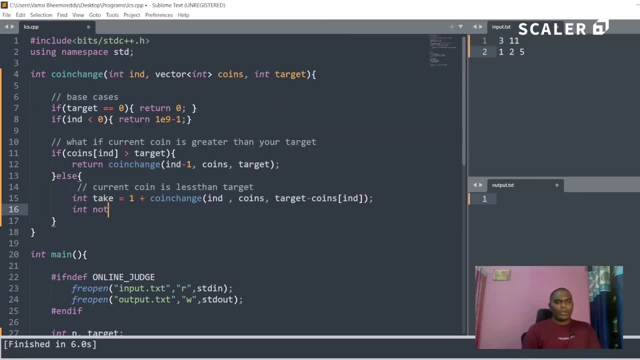 Done. So if I have decided not to take up that coin, Oh, now what if? what happens? so I may not increase my coin value, since I have not taken that? instead, I can have to go to the next index, right? so if I decide not to take current value, 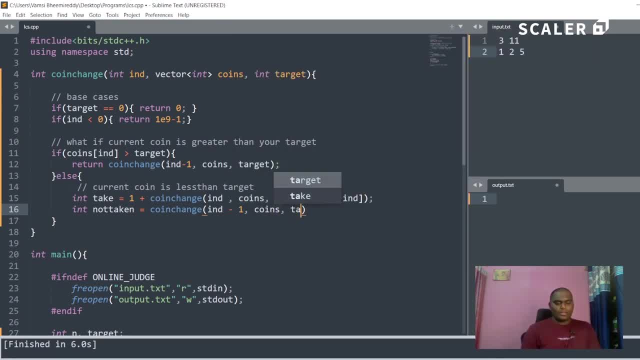 then I have to go to the next one, then coin. since I have not taken that value, my target will be as it is Now. at the end, what I need to do, I need to return minimum of taken and not taken. so this is what a algorithm looks like. 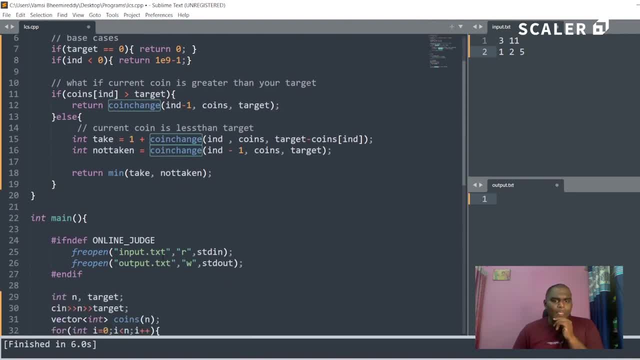 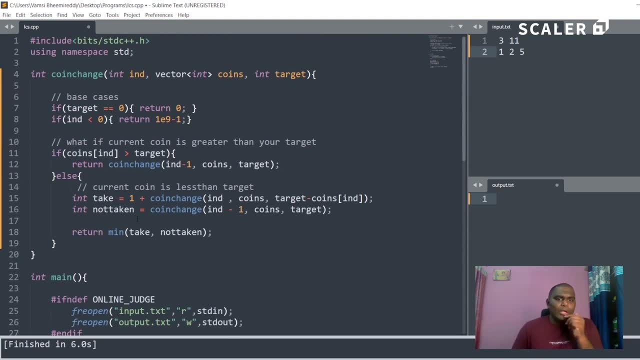 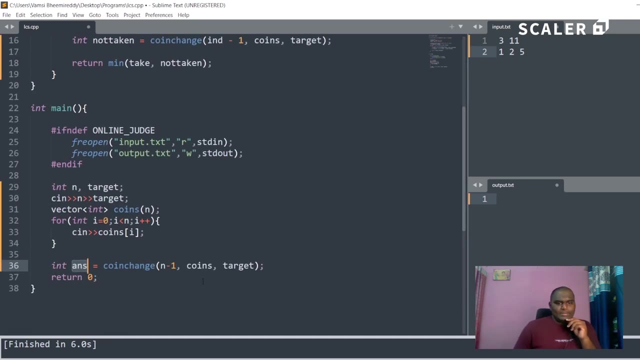 okay, so I am hoping this would return our answer. okay now. so we are getting our answer in answer variable, and so here we need to. I need to make a corner case where we will be returning, like where we will be not having enough coins to make the current change okay. 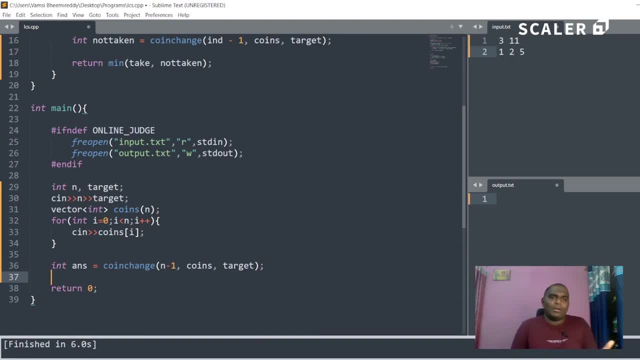 so then what? so what it will return? our algorithm will return 1 e 10 power 9 minus 1. okay, so if answer equal to 10 e power 9 minus 1, so it means that there is some suitable guy. okay, so I can make the change. so in that case, 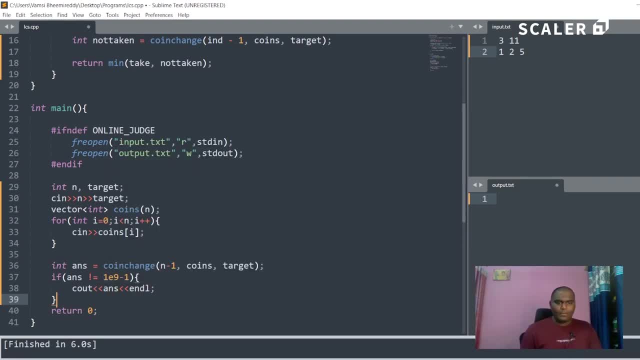 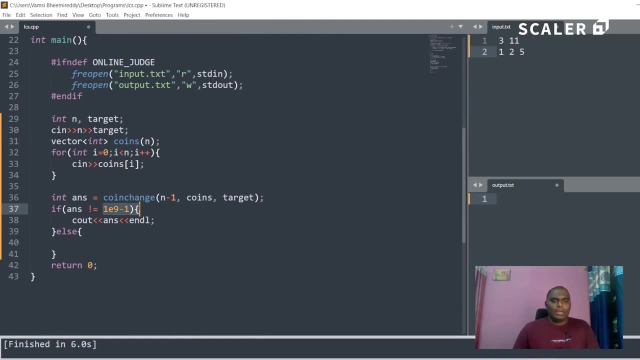 I can. I can print this answer only so. if not, if my current answer is: answer is 10 power e 10 power, 9 minus 1, then I can simply print. I can simply print a minus 1 done so? yeah, yeah, So let's. 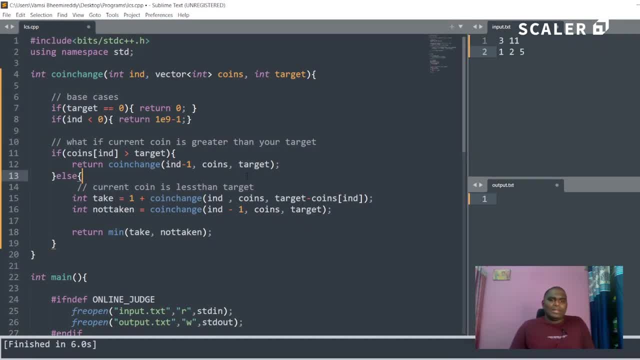 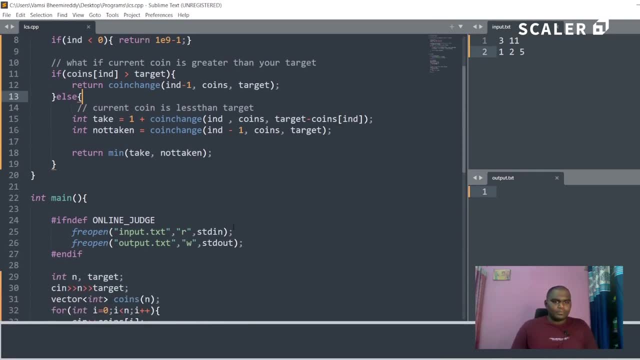 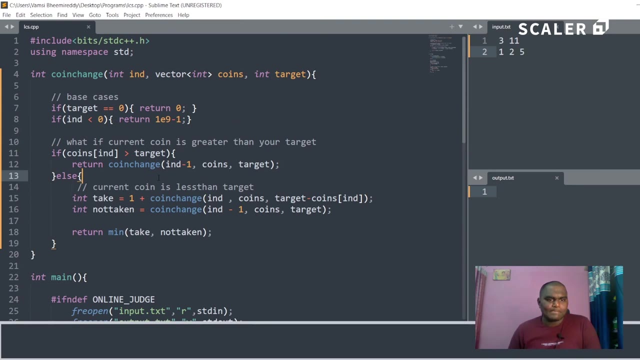 So this input, I am expecting output as a 3.. Let's try to run this code first and then we'll see. since it's Rikasu and the complexity of this approach would be exponential. it is taking a lot of time, Okay. So if given three, okay, let's check out for failure, like where it will be not making not. 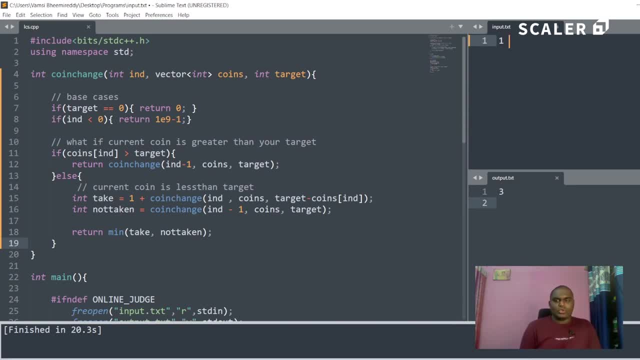 have enough coins to make the change. so my I have a size of one and I'm looking for three and the current values I have is two. okay, I'll save this. Okay, And I will return the answer very quickly this time, I guess, yeah. 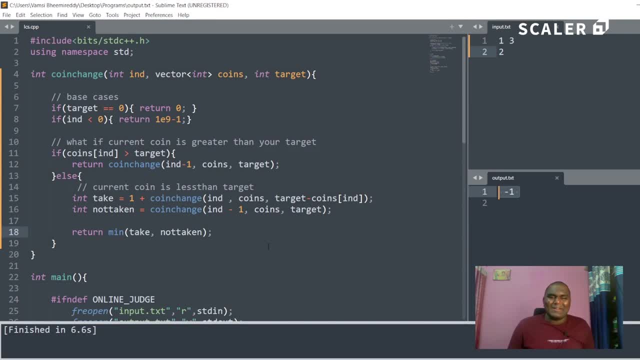 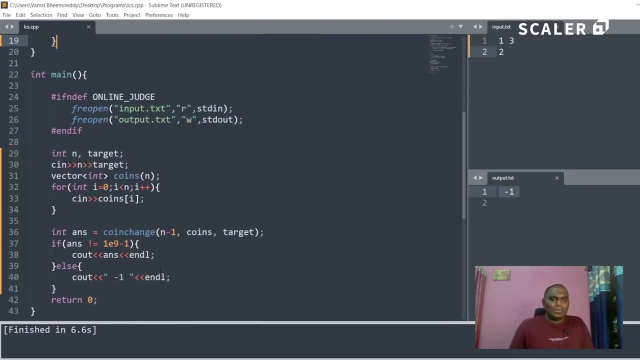 So we got minus 1. so why does it answer very quick? because, um, so we have very less number of cases to check for. so yeah, that is what a time complexity means, why time complices so much important. oh yeah, so it is returning correct answer. now let's try to analyze the 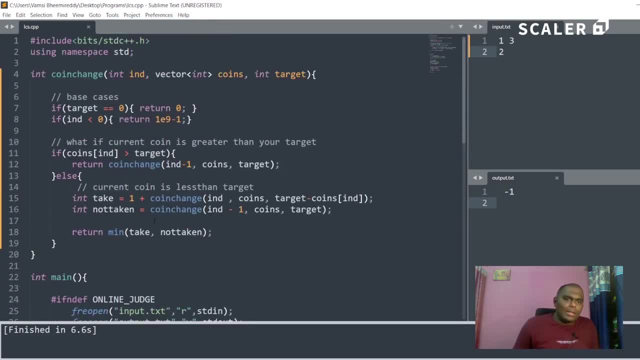 time complicities. this particular approach, yeah, so it is definitely going to be exponential. okay, so why? how exponential? so I am making a two function calls here. okay, so it is a like at max. in worst case. I am making two function calls. okay, then it will be two power, two power or something. so what is that something here? 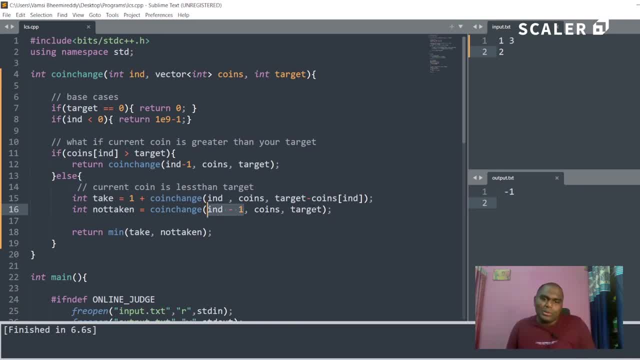 so can I say: what are all my changing factors here? so target and index and target. so can I say I am finding all the possibilities of an current index on the target. so in that case, in worst case, it would be index into target. but if we have here infinite set of coins, since we have infinite set, 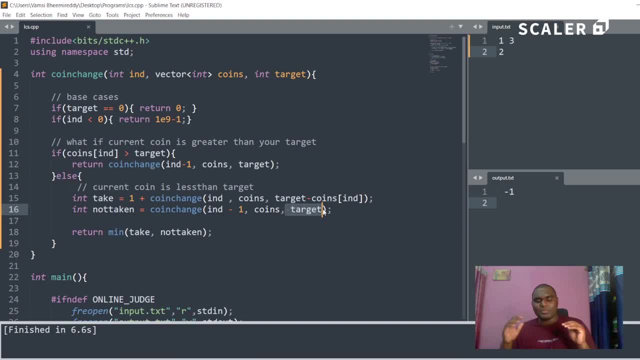 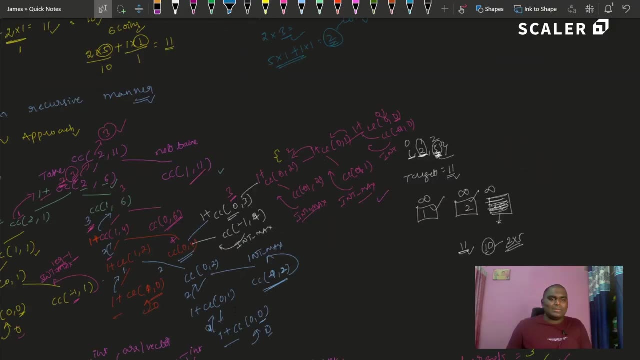 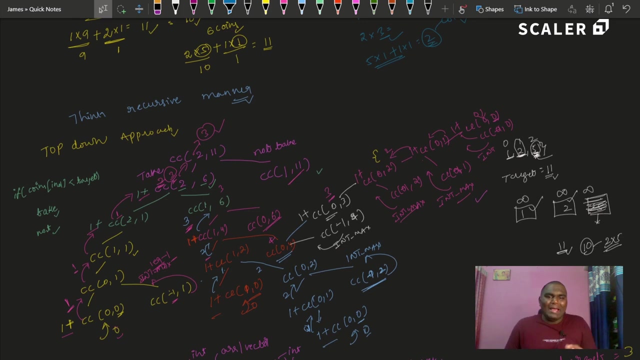 of coins it that time, the time complexity of this particular approach would be greater than two power index into target because we have infinite set of coins. since we have seen that recursive tree as well, it has a lot, lot of recurrences. okay, it has a lot of recurrences. okay, I have stopped at the middle. 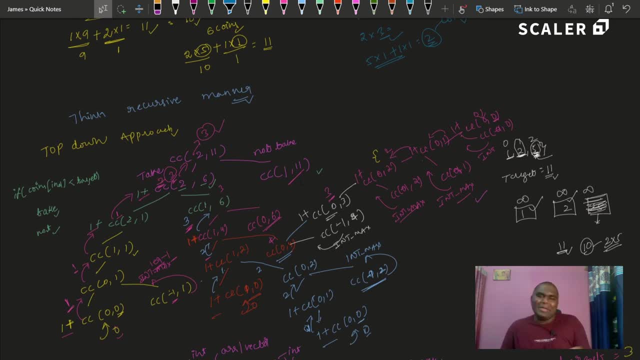 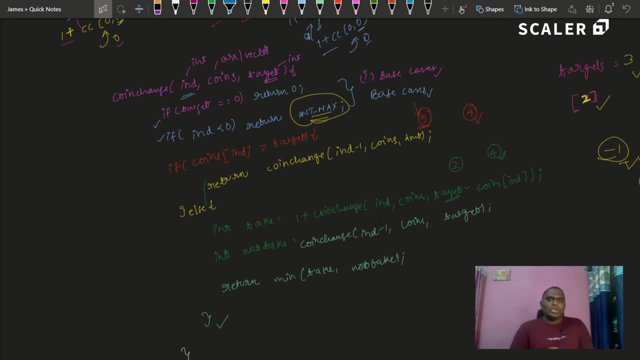 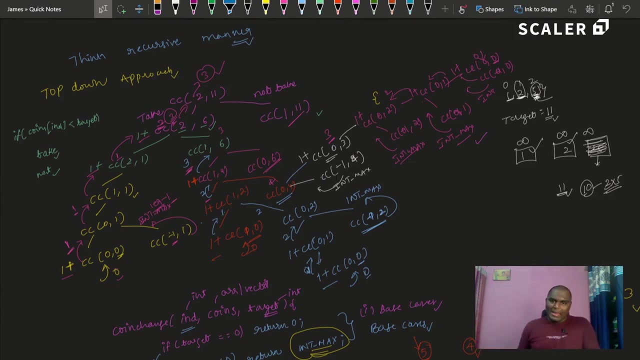 but it has a lot okay. so, yeah, if you are in an interview interviewer, then straight away ask you to optimize this particular solution. so how to optimize this, how to optimize this, so what you can see here? so I can see, I can see I am repeatedly solving the problem which I have solved a previously doesn't make sense, yeah it. 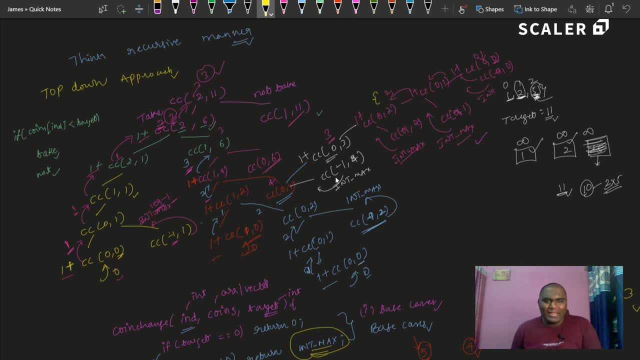 makes sense, right? so let's see, so let's figure out, let's figure out something. so here, CC of 0 comma 1, and again I am solving CC of 0 comma 1. yeah, and again I am solving CC of 0 comma 1, again I am. 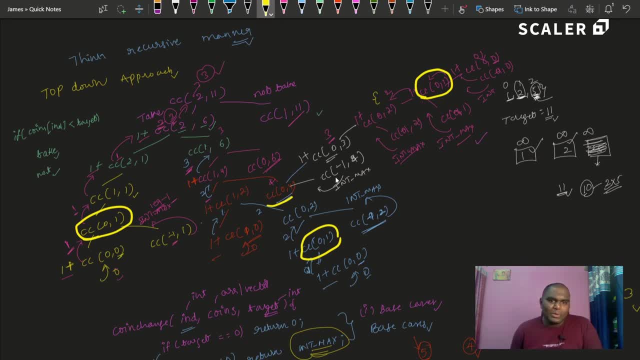 solving CC. so it's repeated like I repeated, right, so 1 comma 4 again. and so, yeah, 0 comma 0, everywhere, 0 comma 0, and again I will be having 0 comma 0, 0 comma 0. okay, so I am solving the same problem again. 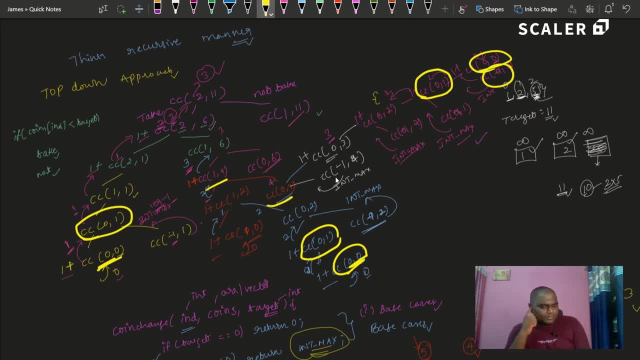 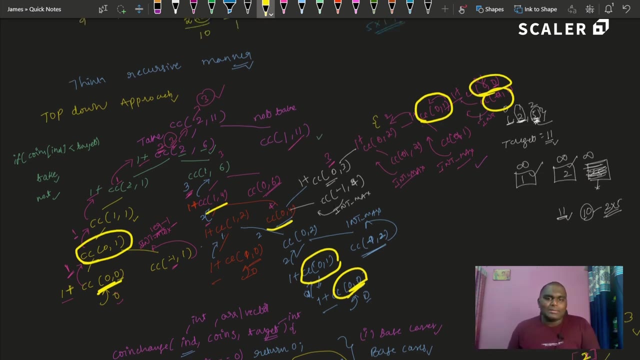 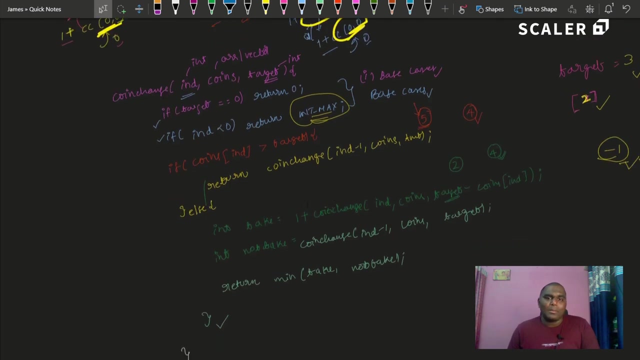 and again, so can I say it has optimal structure. sub problems so and so. whenever there is some cases where I will be doing same task repeatedly, like same same task more than one time, in that case I can say memoise, I can memoise the answer. so memoising answers can be comes under dynamic. 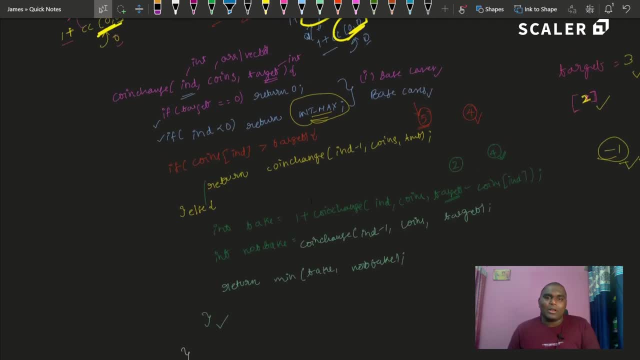 programming. okay, so how can you convert this particular logic into the dynamic programming? so basically, let's say so: first you need to figure out of what are all the changing factors here, so index and target, or the changing factors here, index and target. so you have to create an. 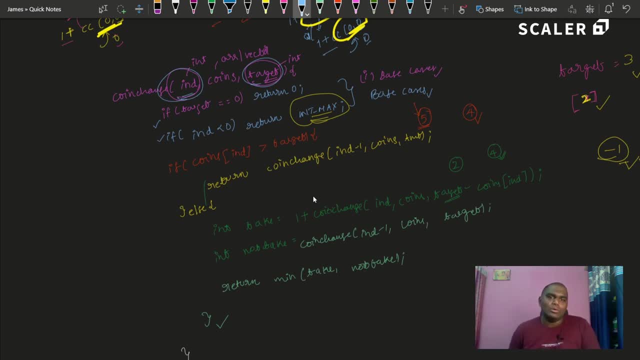 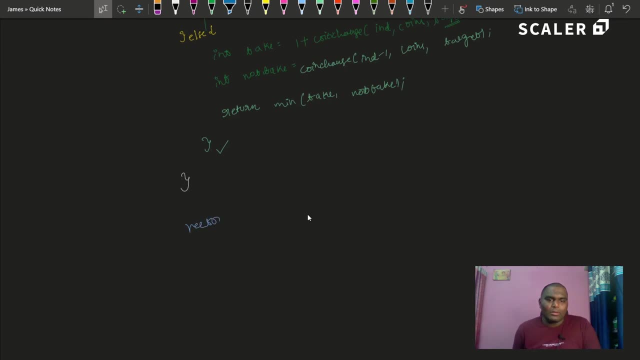 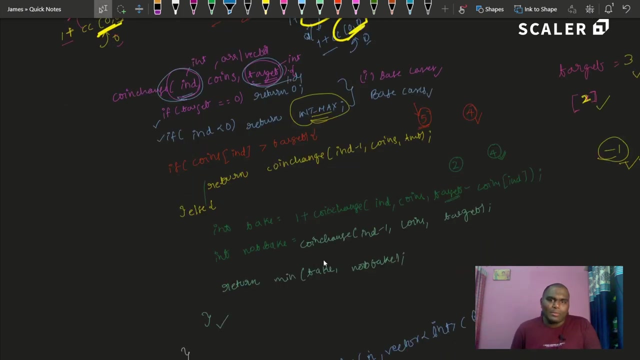 2d matrix with the size of index into our target. okay, so let's say simply a vector of our vector int dp n into vector of int target. initially, I am- let's assume I am initially filling it with minus 1. okay now. so what I can do, I can pass this dp here. okay, I can pass this dp here. 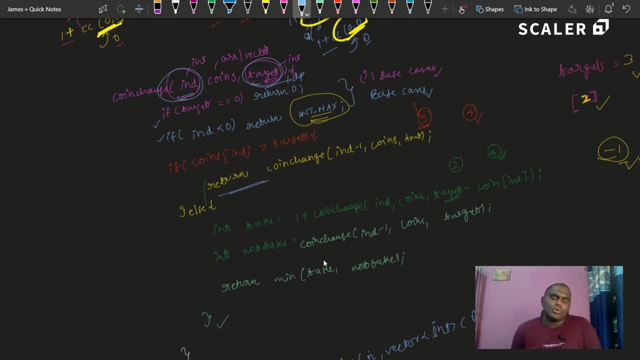 and whenever I am written I can pass this dp here and whenever I am written I can pass this dp here, returning my answer. so not simply returning the answer. so before returning answer to my main function, I can say: store that in my state, dp state. so what will be my dp state? so dp of index of. 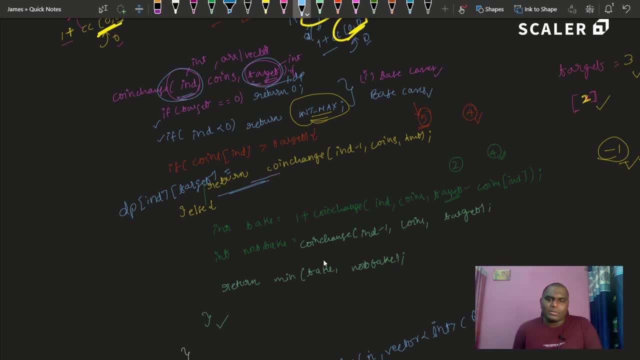 target. so I will store that answer into this particular state. so that is how I will do so. wherever I am making recursive calls I will do that. so here again I am considering the answer. so in dp of int and target equal to min of take comma, not take. 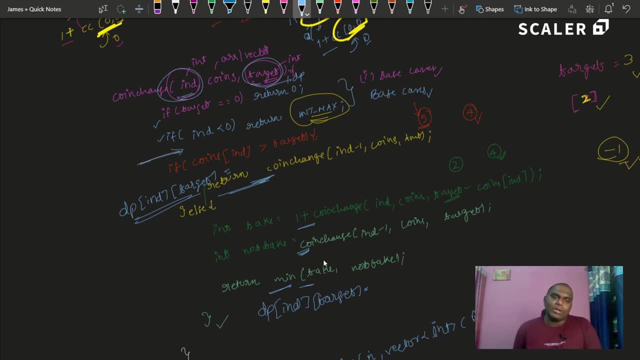 so here, before entering into this logic, like right after the base cases, I will include a check here whether I have solved that particular combination like so zero, comma, zero cases like in where index is zero and target I am searching for is zero. so such cases, so whenever I will check here, okay, 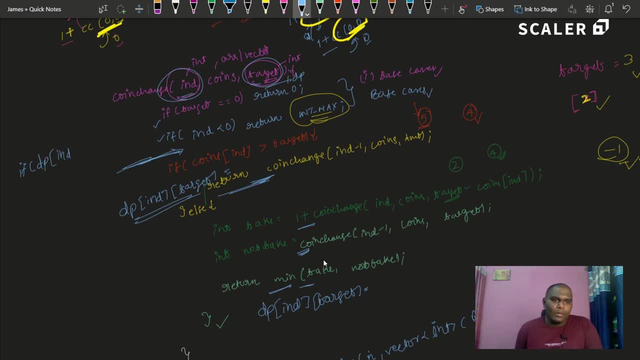 so like dp of index of target, so not equal to minus one. so if that index, like that particular state, has um, not uh, doesn't have minus one, it means that it has some value. it has already computed. so what I will do, I will simply return that answer. so dp of target done. yes, this works this. 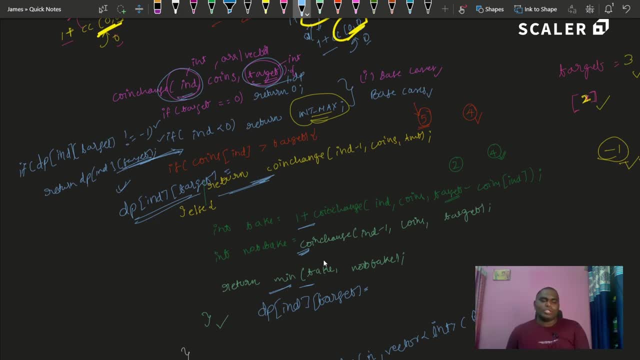 is what a memoization means. okay, so my motion means you will be having your recurrence recurrence code and you will be simply just converting that code to the dynamic programming by simply adding your dp states over there. okay, so let's go and code this particular solution. so we are not writing. 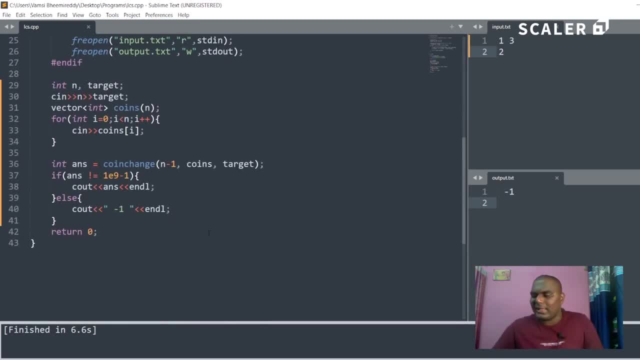 code from the scratch, so we will be just doing some modifications here only so. the first modification is: you need to create a two-dimensional or of vector e of size n into size of target. so I'm filling it with minus ones, okay, and I need to pass this. 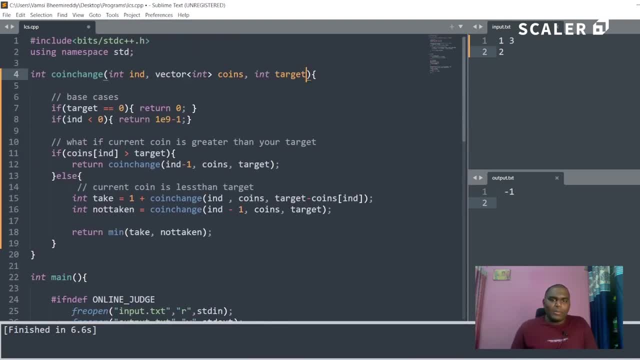 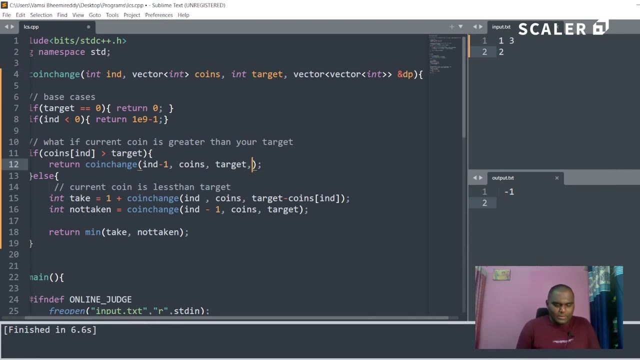 mint, then if I'm passing as my argument, I have to catch that in my parameter as well. so whenever I'm making call I need to update, as always. so here dp. so whenever I am returning something. so before returning I just have to db states x of 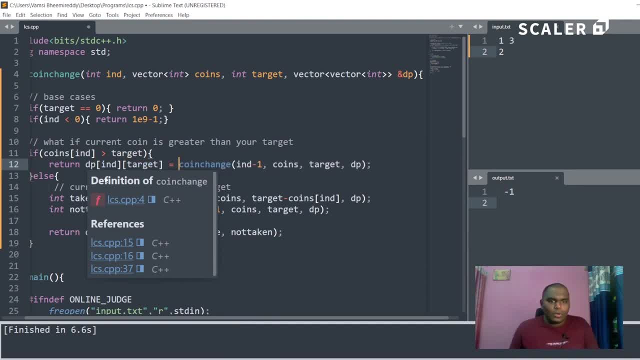 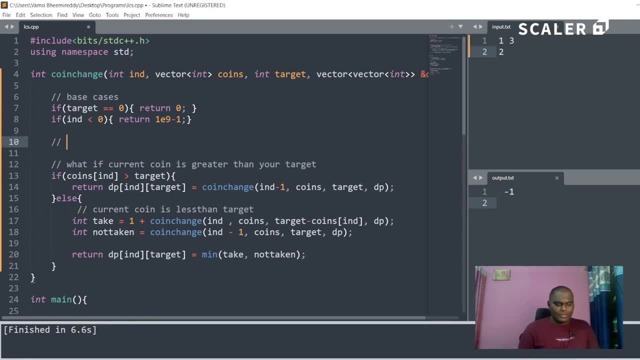 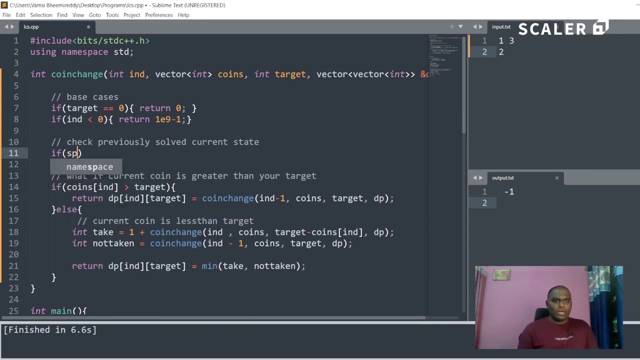 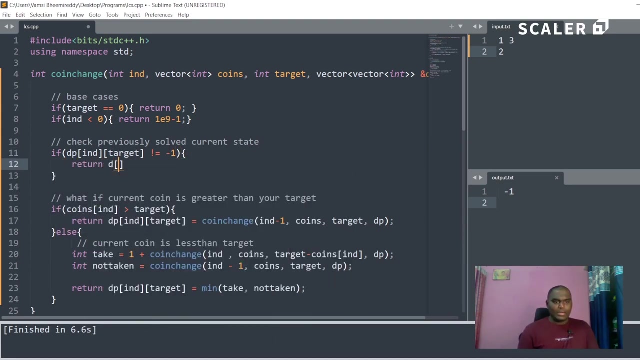 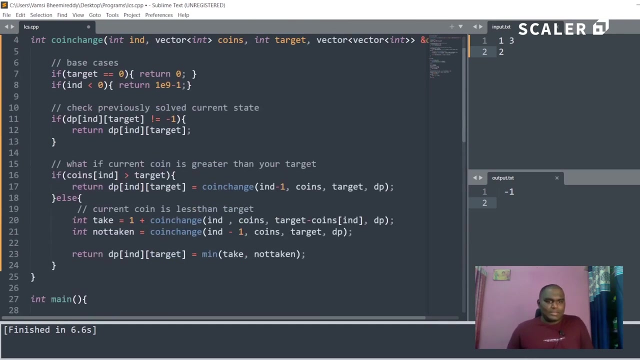 a target previously. if a dp of x of a current target is not equal to minus one. not equal to minus one means that simply return that. do we need to forgot anything? no, okay, save this and um, so let's try to give change our inputs. three, eleven and one, two, five, so I'm expecting three as my answer. okay. 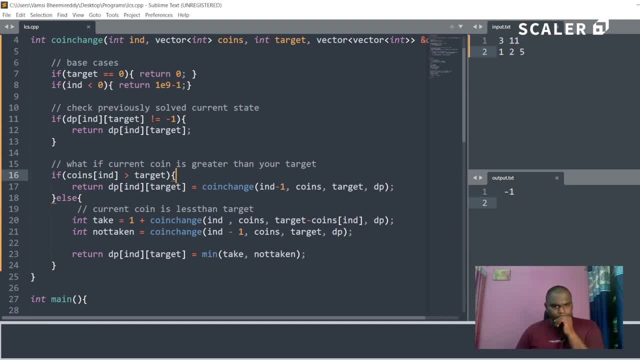 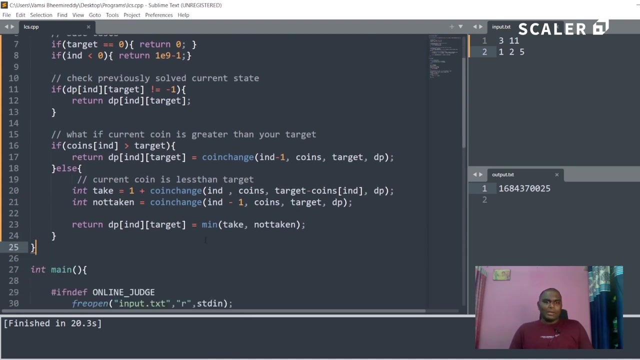 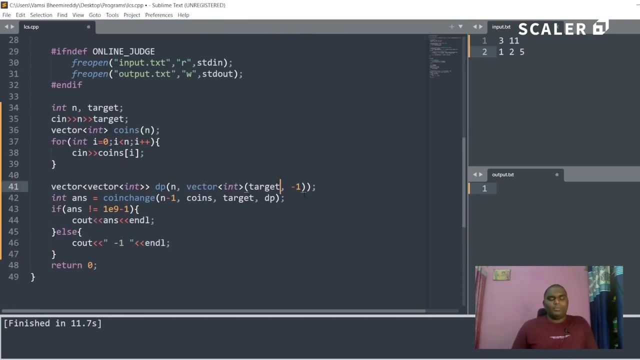 so I'm expecting three as my answer. so I'm expecting three as my answer. so I'm expecting three as my answer. so people getting back, so we got something bigger, two ammo. so yeah, so we need to include a target plus one y. so we are searching for target eleven. so we have to assign this space of 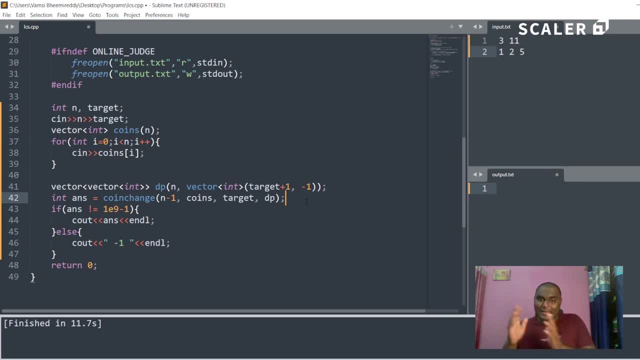 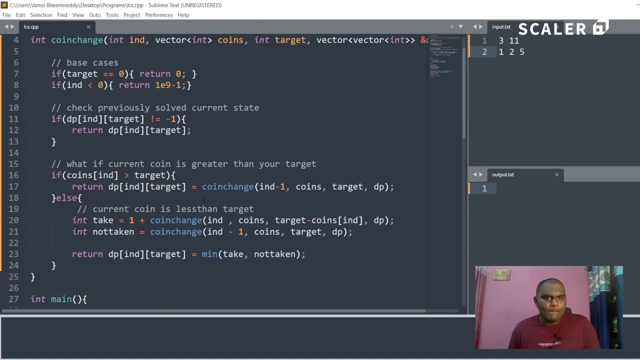 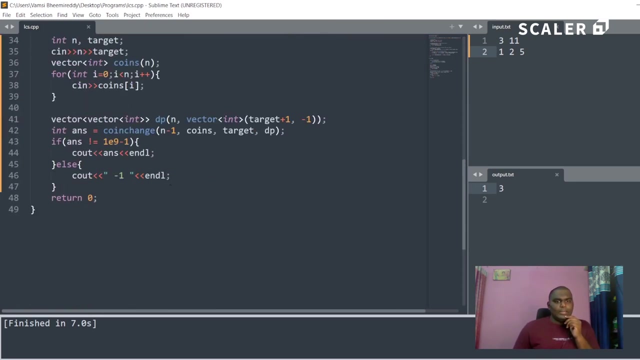 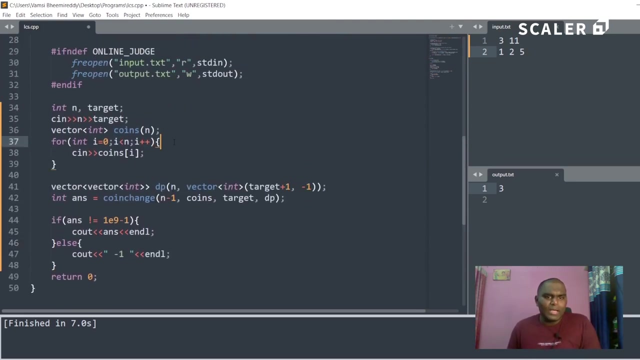 but we have to assign the states at till eleven, right, so that is a common. so after I think this course is good, I'm going to favorite this class one, right? also, I want a zero because- some silly mistake I did. let's try. it works fine, I guess. okay, now let's try to analyze. 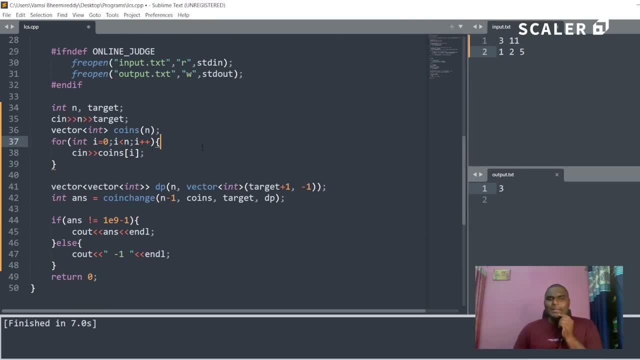 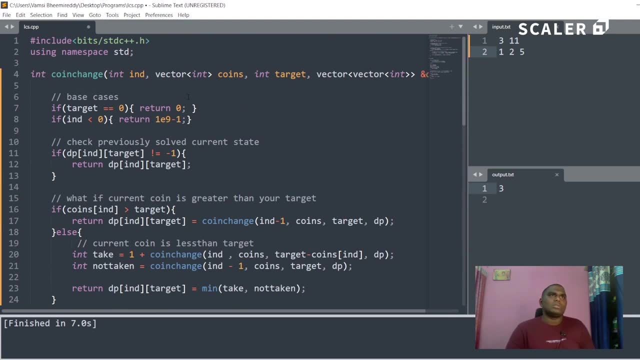 the time, complexity of this particular approach. so, basically, if you are in an interview, if you come till so far, it's fine, because I have seen this problem in a couple of platforms as well. the cases were not that much bigger. like maximum, like target will be maximum. 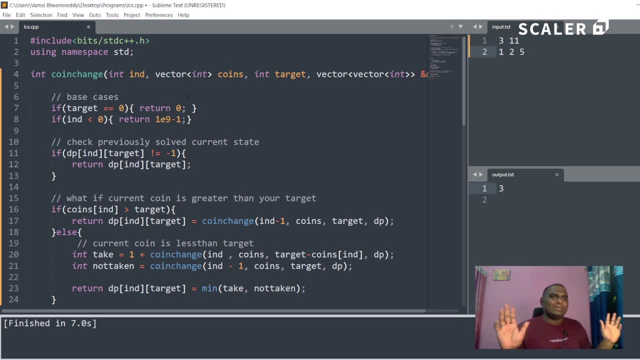 of 12 and the end will be maximum of 10, sorry, not 10,000,. okay, it's a 10 power 3 or 10 power 4 at max. okay, this particular DP solution. okay. so the time complexity of this approach. 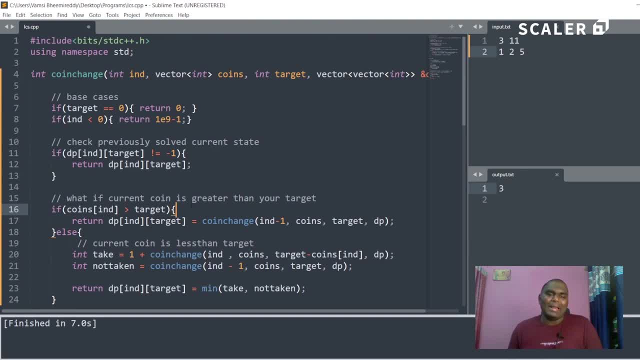 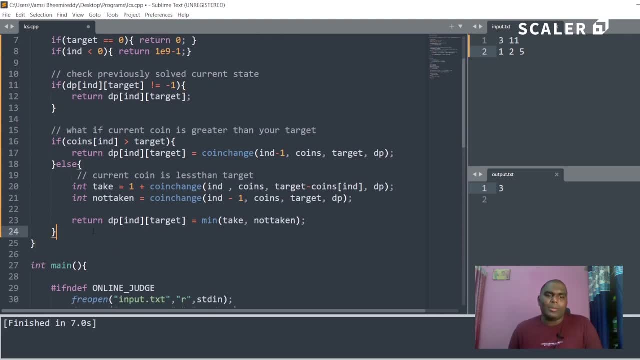 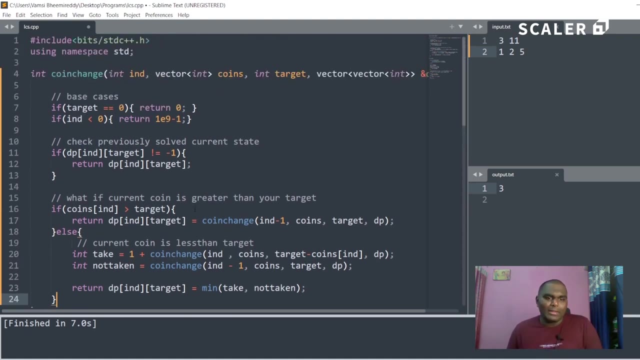 particular approach would be okay. it would be like: n into target- okay, and space complicities. since we have written memoization code, it will be taking extra stack space, okay. plus, we have taken the 2D dimensional vector- 2 dimensional vector with the size of n- into.